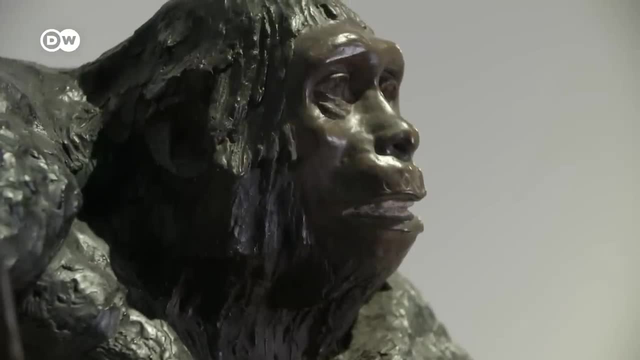 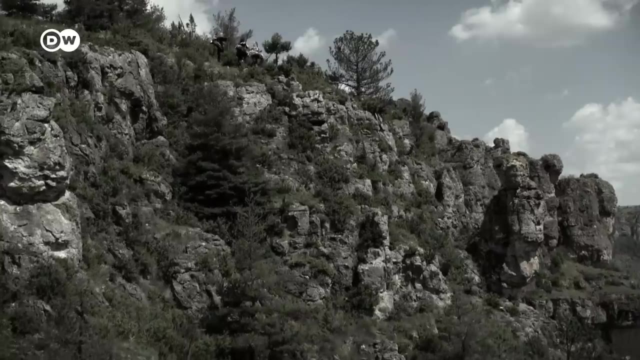 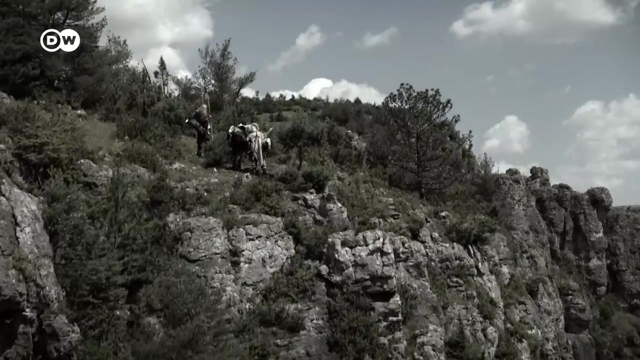 A more realistic picture of the Neanderthals evolved decades later. A more realistic picture of the Neanderthals evolved decades later. It was called the Neanderthal Extinct. Analysis of their remains and various artefacts provided details about the way they lived, the survival skills that they developed. 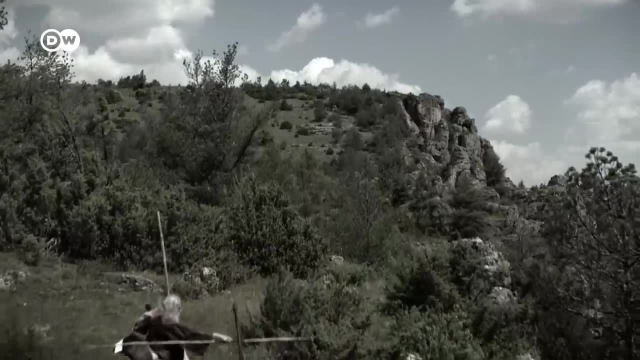 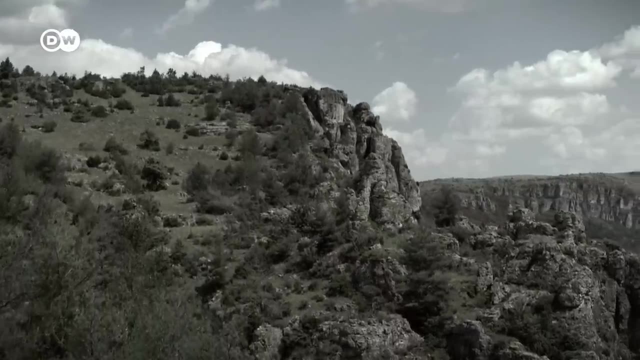 and the climate in which they lived. In the most part, the environments in the Neanderthals were very harsh. There were also many visitors to the place. The climate in which they lived in was extremely harsh during the late Cretaceous period. 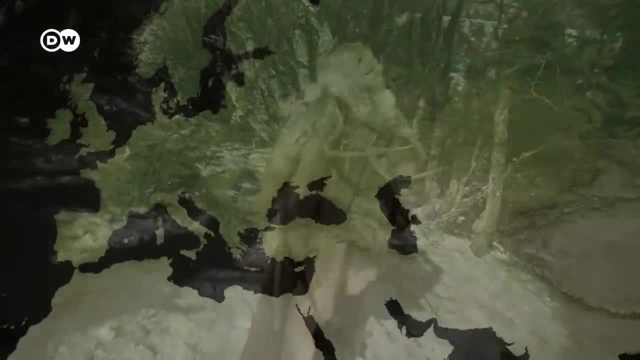 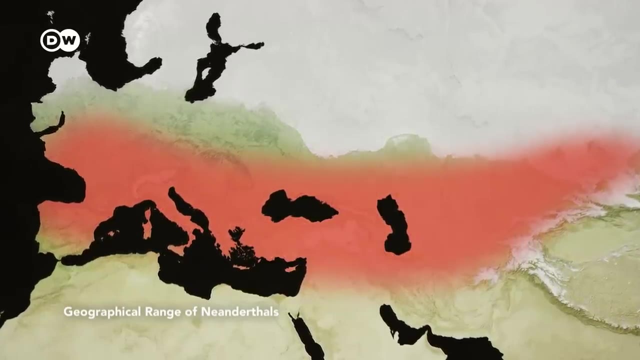 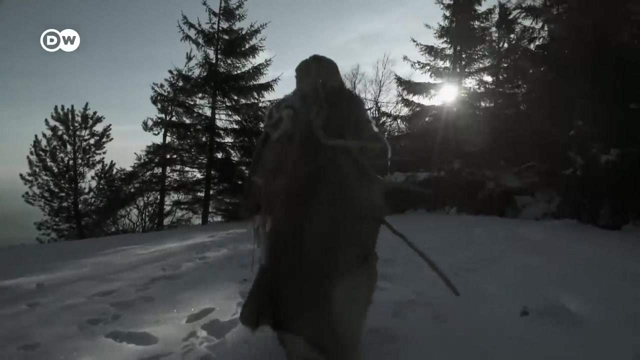 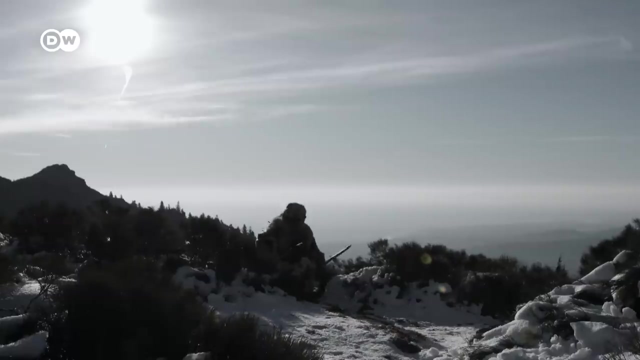 harsh during the millennia that Neanderthals inhabited the Eurasian continent. This was the Ice Age, and there were periods of extreme cold, with temperatures dropping to minus 20 degrees Celsius, and sea levels were much lower than they are today. The evidence indicates that the Neanderthals adapted well to these particularly difficult conditions. 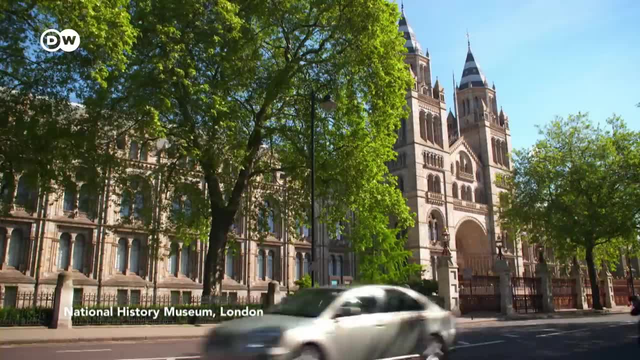 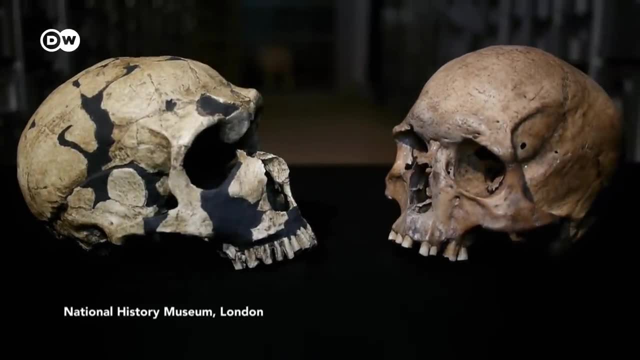 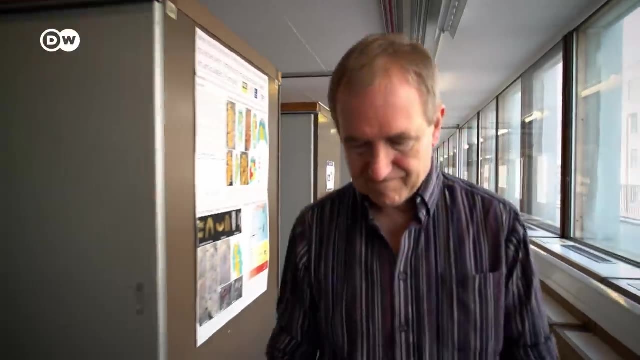 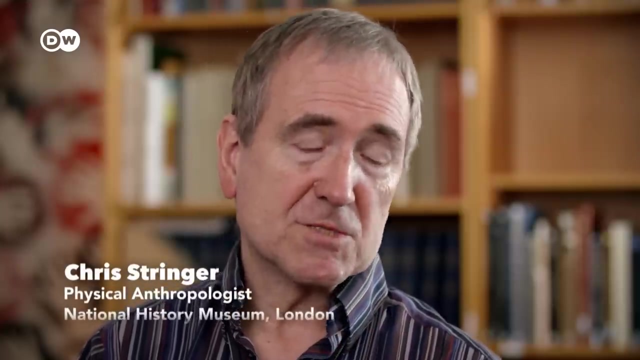 The Neanderthals were very much like humans. Paleoanthropologist Professor Chris Stringer of London's Natural History Museum specialises in the physical and anatomical development of early humans. The Neanderthal face is very different to the shape of a modern face. 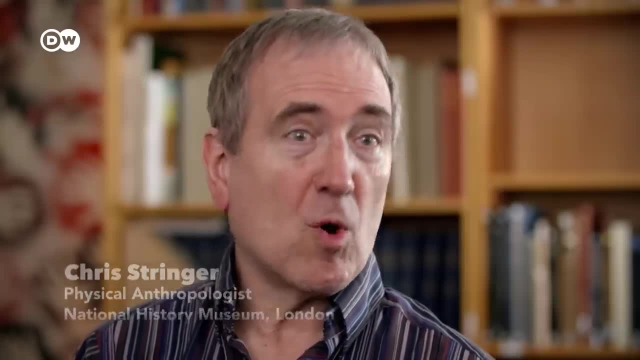 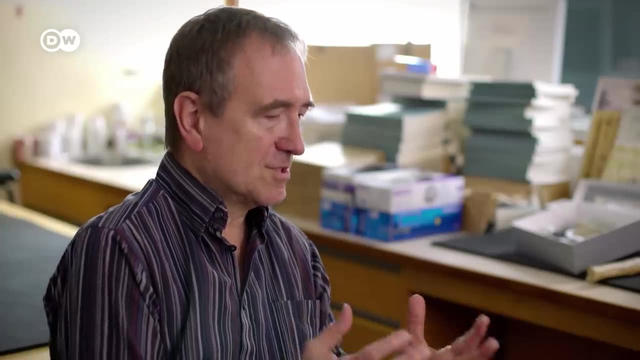 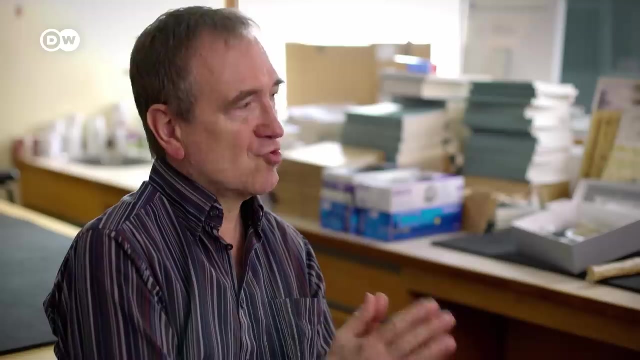 and many arguments about how that face evolved and why it evolved, And I think that's the reason why the Neanderthals were so popular. I think the view now is that certainly that face it's partly to do with cold adaptation. So we know Neanderthals evolved in conditions that were largely colder and drier. 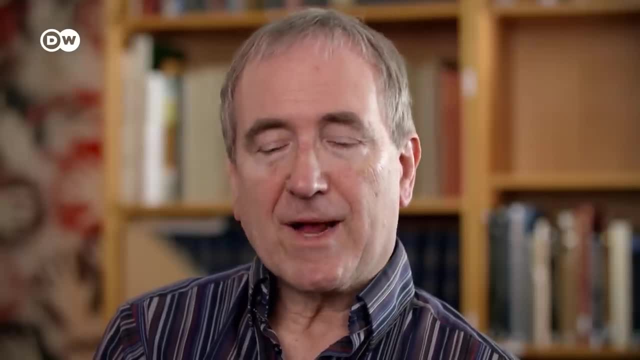 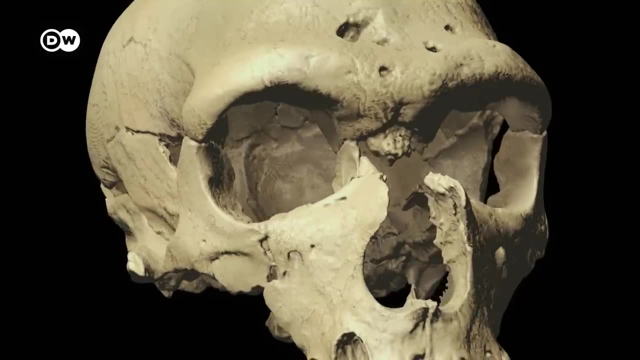 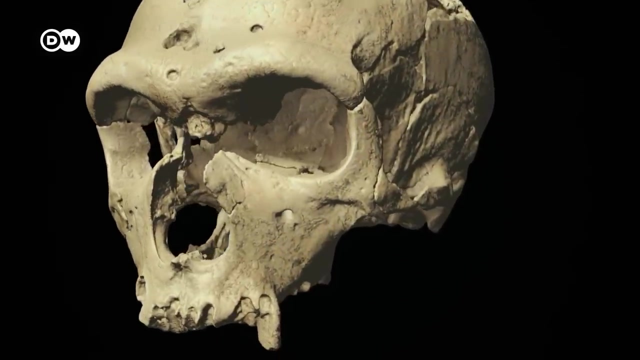 than the present day in Europe, And it's likely that that face was particularly the nasal area, because the nose is very large and it's pulled forwards. It has a very large internal volume, So partly it seems that it's there as acting like a radiator. 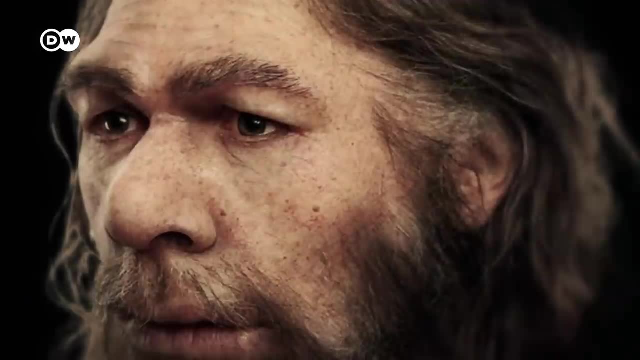 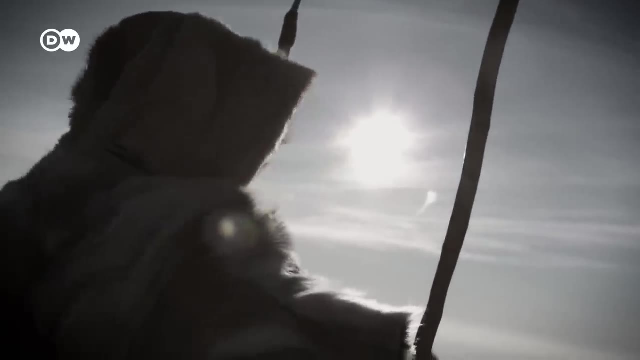 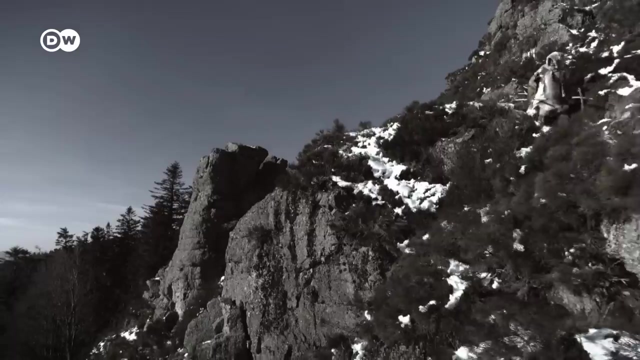 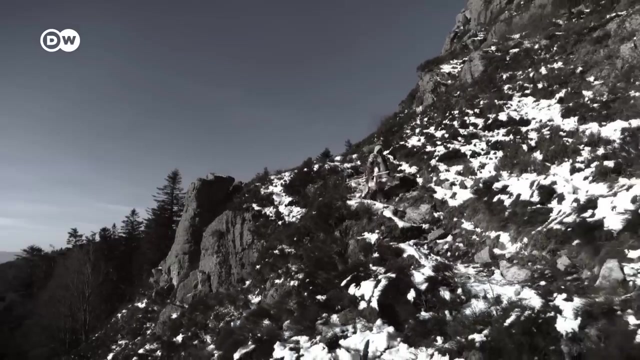 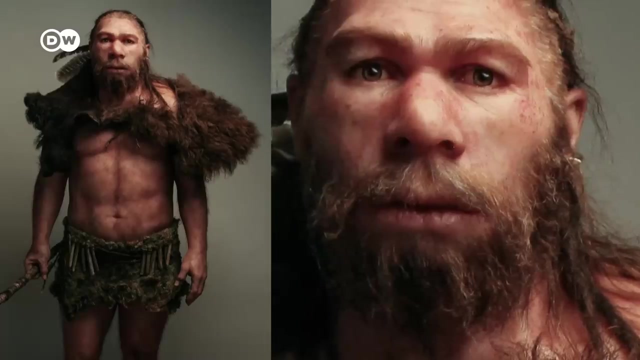 It's warming up and humidifying the air that's coming in. And this was true for all of these ancient humans. All of them really have larger nasal apparatus than modern humans do. But Neanderthals take it to another level: They really are pumping a huge amount of air through their noses. 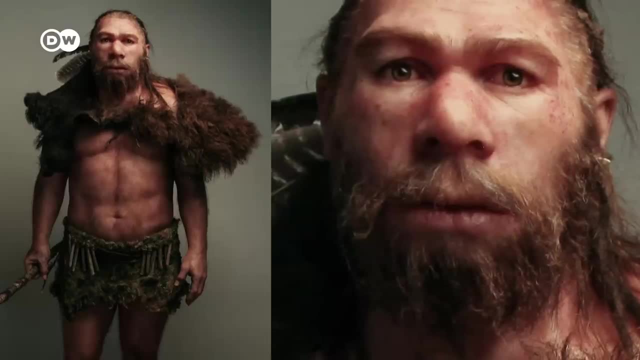 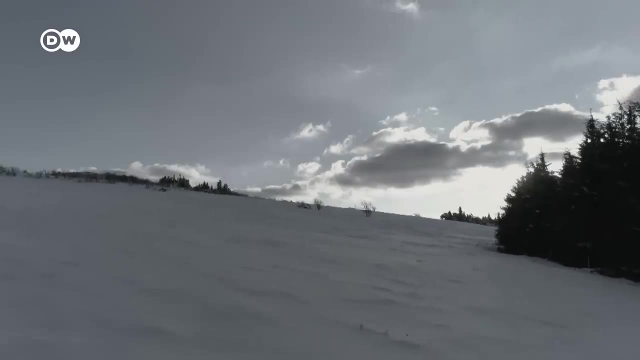 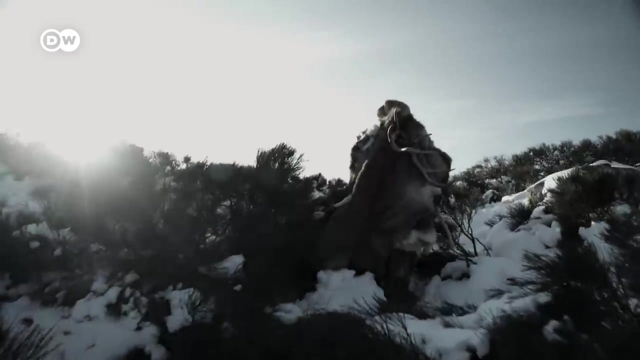 And they've got huge lungs, barrel chest. They need to oxygenate their blood. They're burning more energy to stay warm as well. These physical characteristics helped the Neanderthals survive in an inhospitable ecosystem. They also developed an importance. 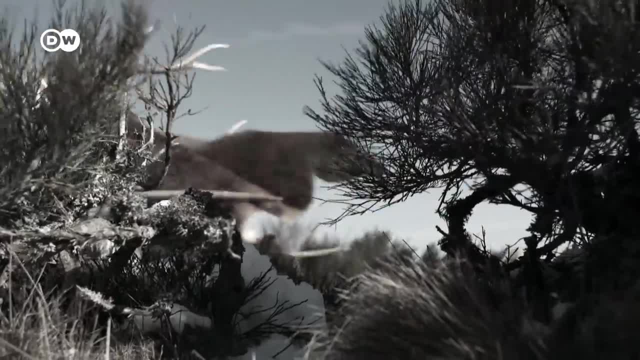 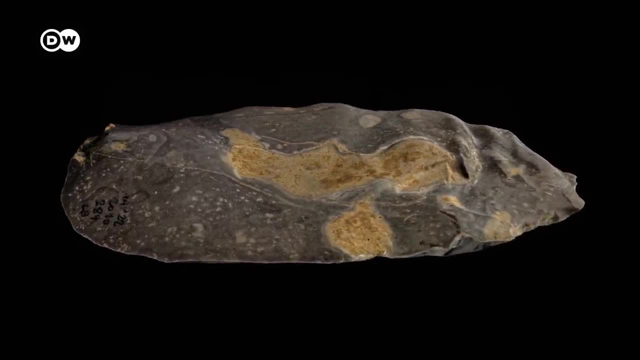 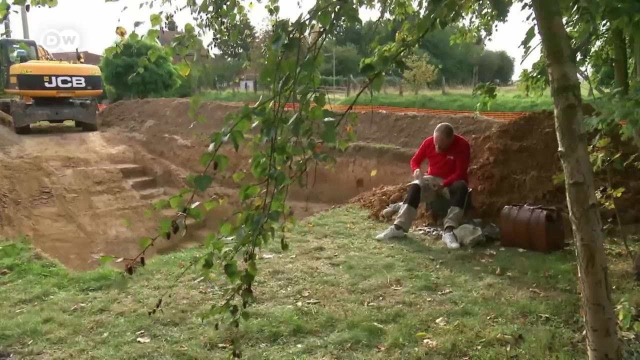 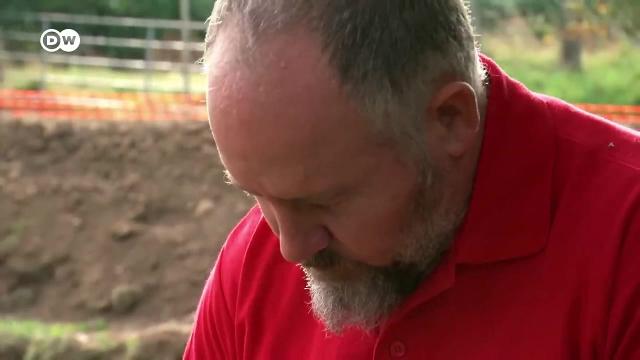 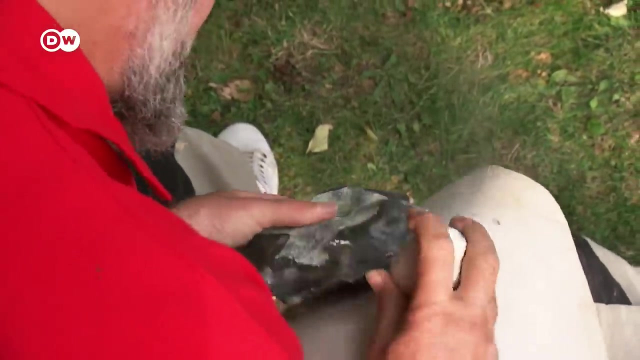 skill making tools out of flint and other materials. This was groundbreaking technology. It's known as the levallois technique and involves using a rock or bone to chip off thin, sharp-edged flakes from the core material. Here, archaeologist Vincent Lascour demonstrates the technique. 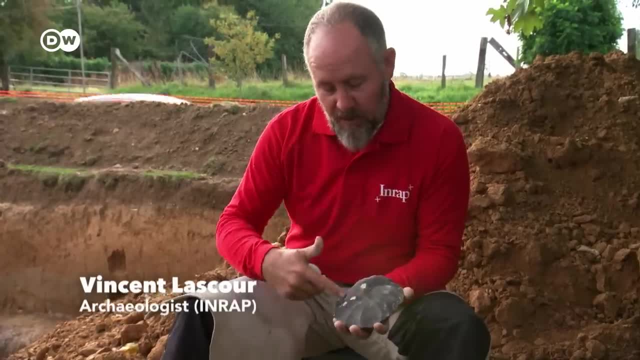 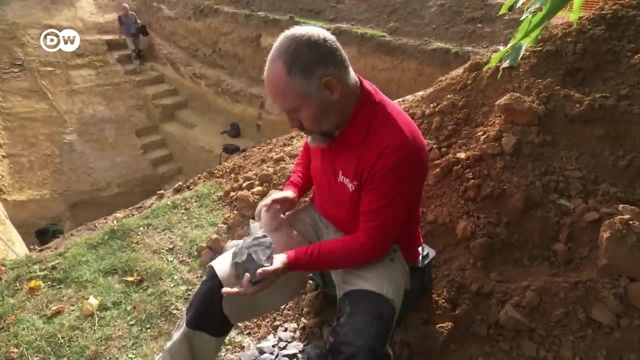 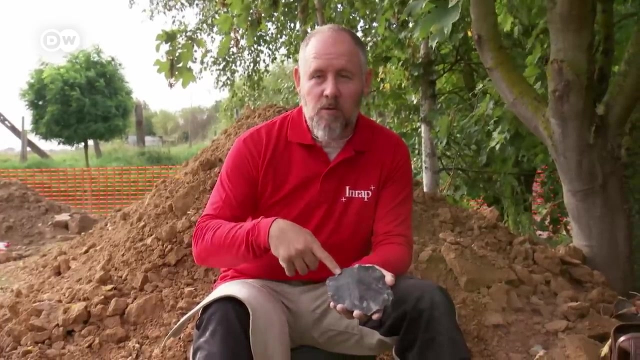 I'm shaping the core And then I'll remove pieces that could be used as tools. This is what's called a levallois point. It runs along these ridges. Now I'll break off a piece. It's a long, slow process. 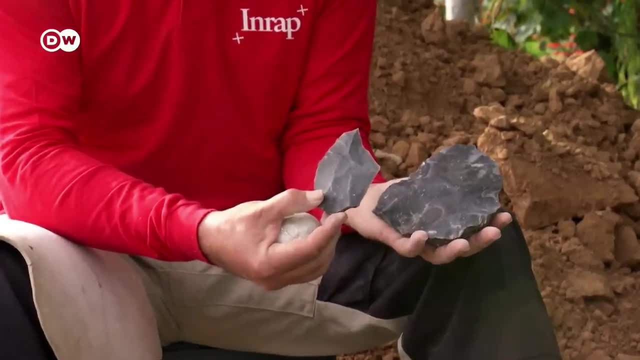 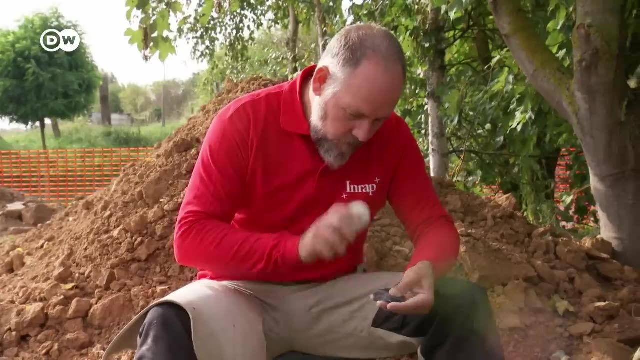 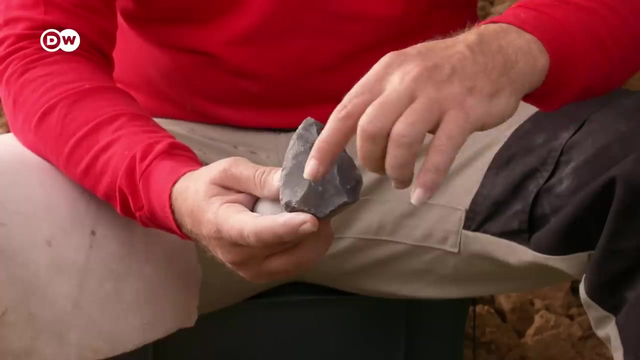 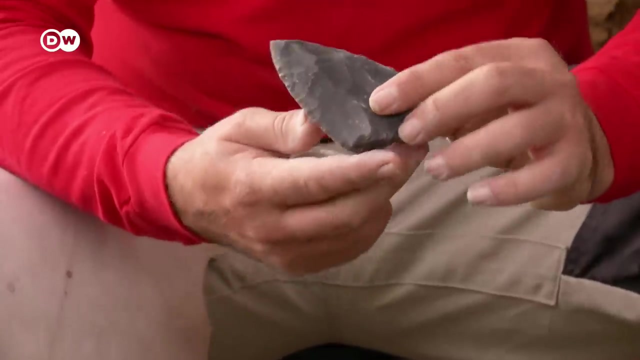 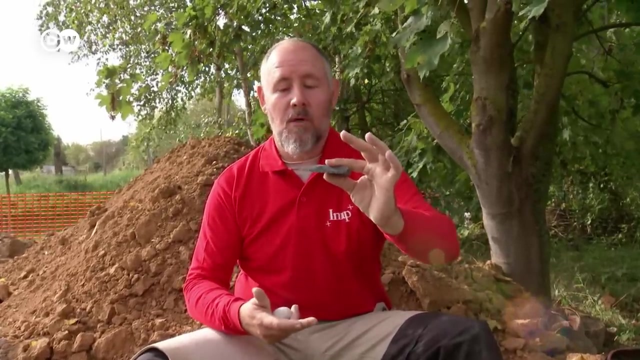 Now he has to sharpen the edges. Here you can see the distinctive features of this process: The two ridges that come to a point. the beveled cutting edge. This concave ledge could be used to attach the pointed flake to a spear. 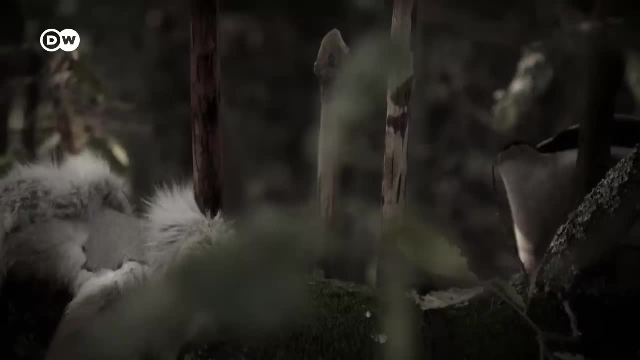 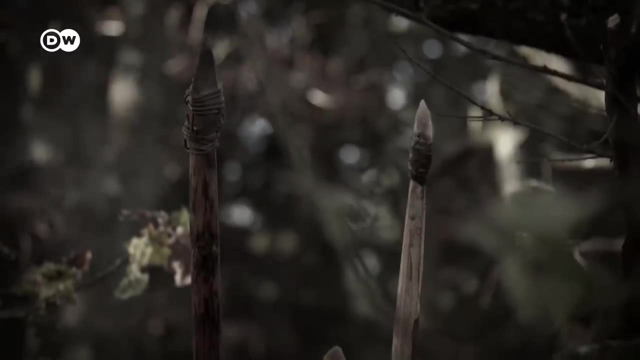 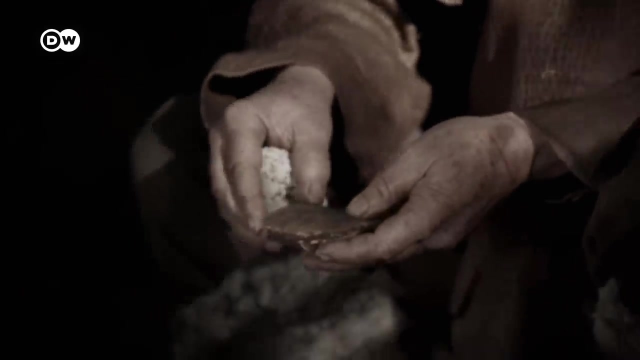 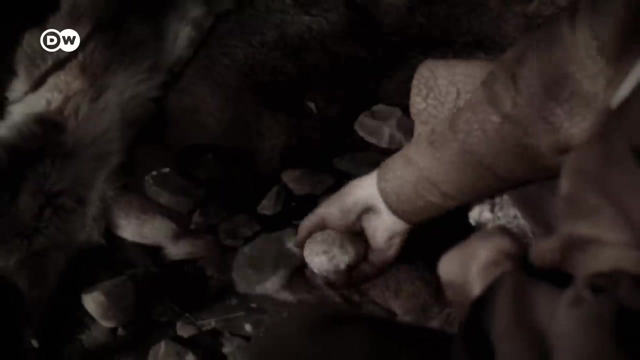 The levallois technique helped Neanderthals create weapons to hunt large animals that would provide them with meat for food and skins for clothing. This allowed the Neanderthals to spread across the continent continent despite the cold weather. They were also able to adapt to brief interglacial periods that were marked by significant increases. 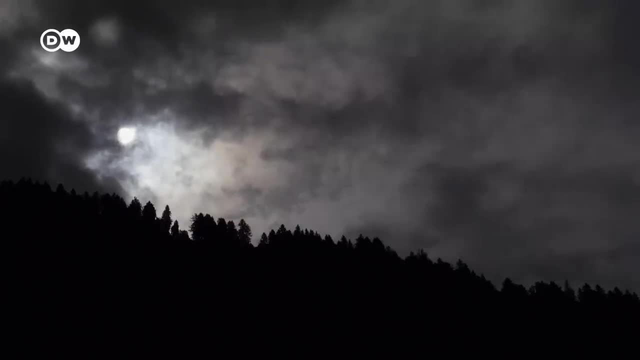 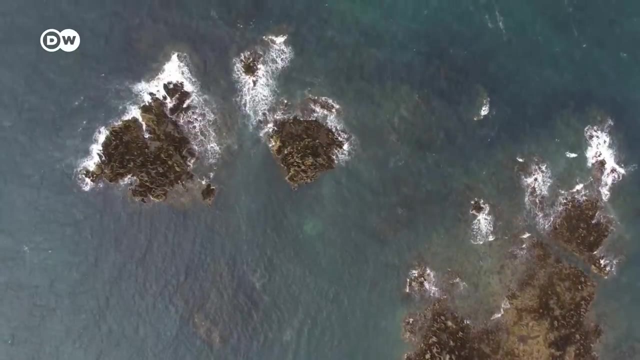 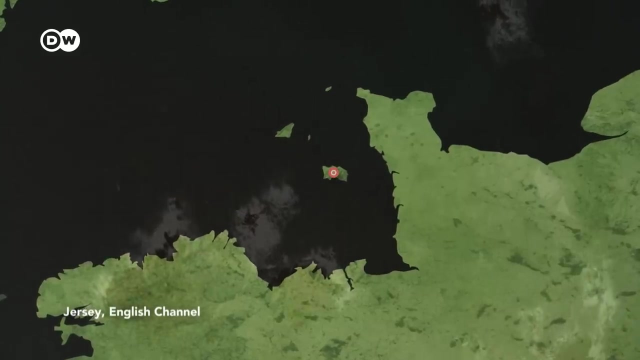 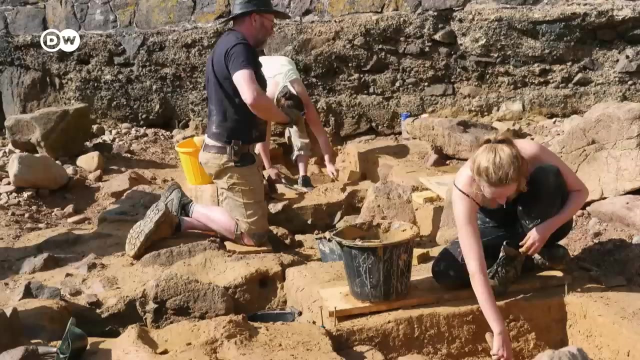 in temperatures. There are only a few sites where experts have been able to study thousands of years of Neanderthal history. One of them is on the island of Jersey in the English Channel. Excavations over the course of the last century have revealed new details on the lives of 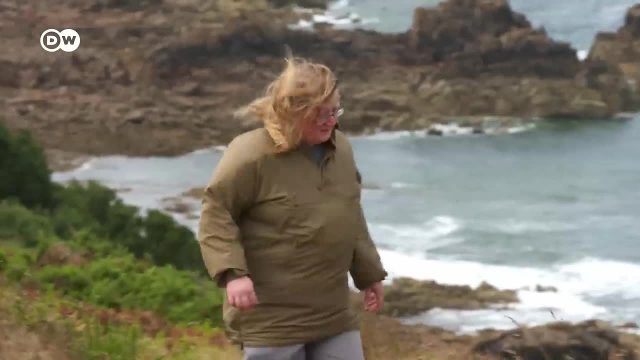 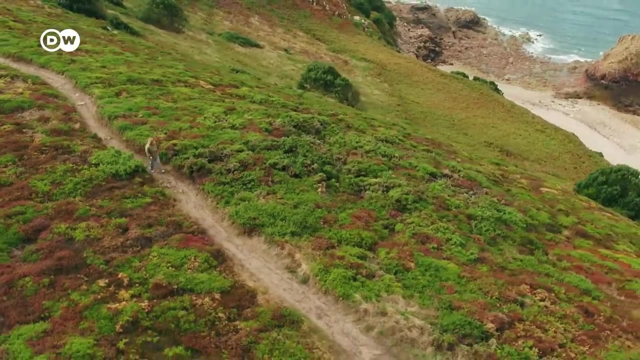 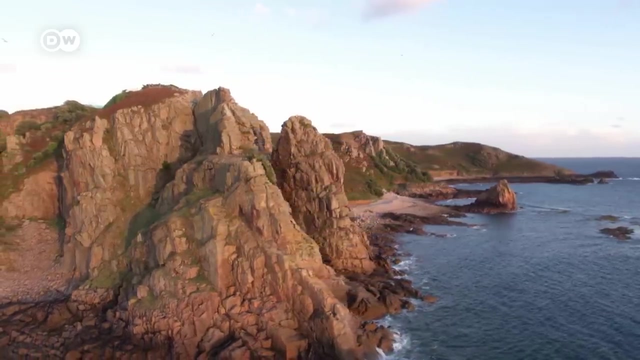 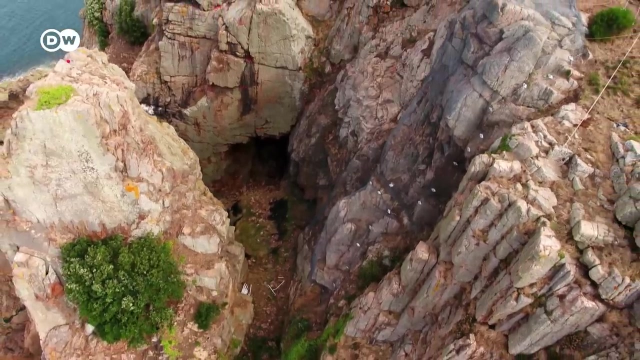 these early humans. Archaeologist Becky Scott is a researcher at the British Museum. She and her colleagues have spent several years studying the Neanderthal site at La Côte de Saint-Bréant. The sediment's preserved within the fissure begin accumulating at least 240,000 years. 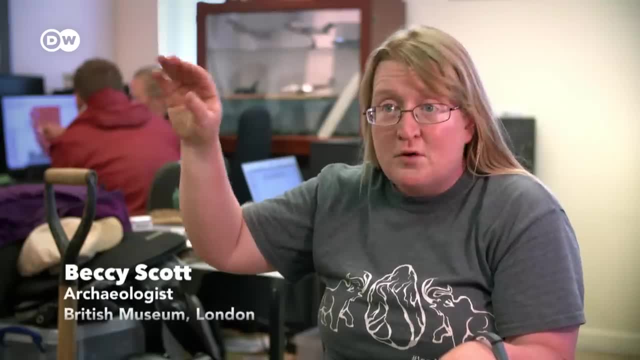 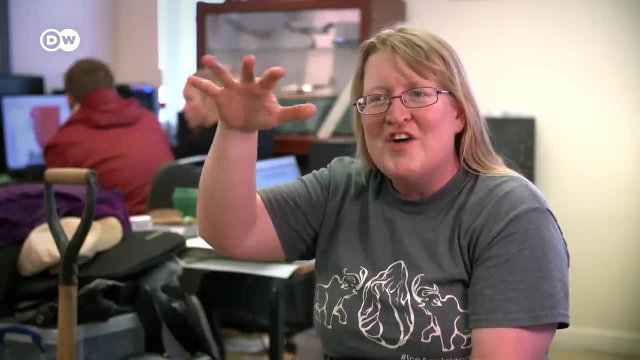 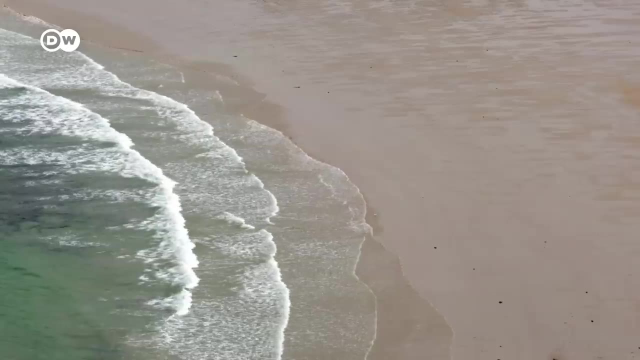 ago through to. we have dates now of around about 40,000, and there were later sediments as well. So actually that captures that entire time span, But what it also captures. What it also captures is huge changes in climate and environment. 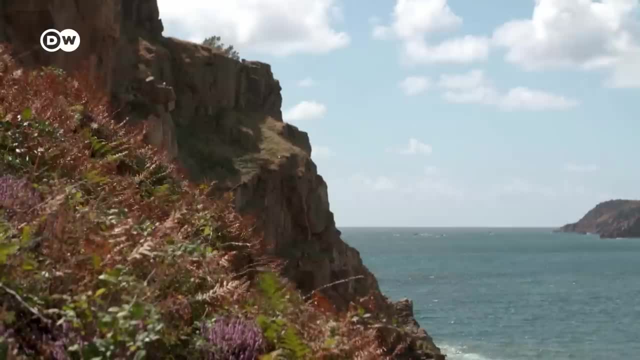 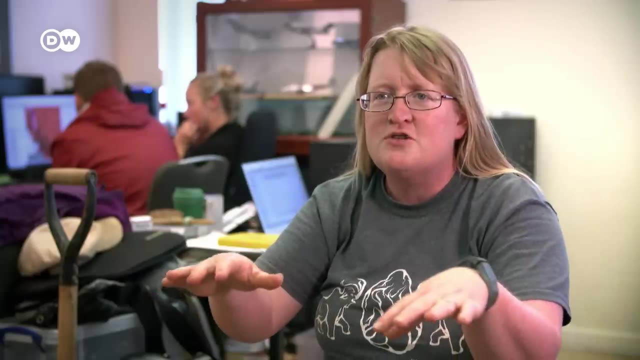 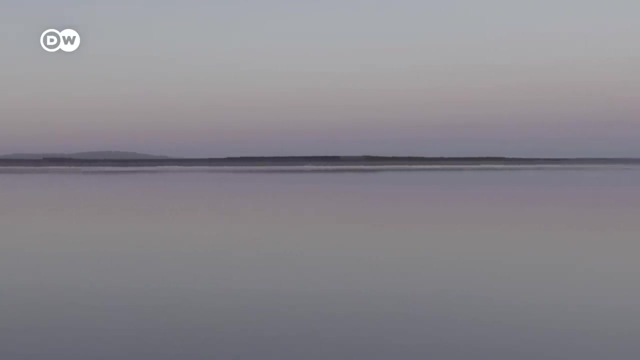 So there are times when it's warm- you know, it's nearly as warm as today- and the sea is quite close. There are other times when it's cold. we're dipping down into a glacial period and the sea is locked up a long way north of the site and a completely different landscape's exposed. 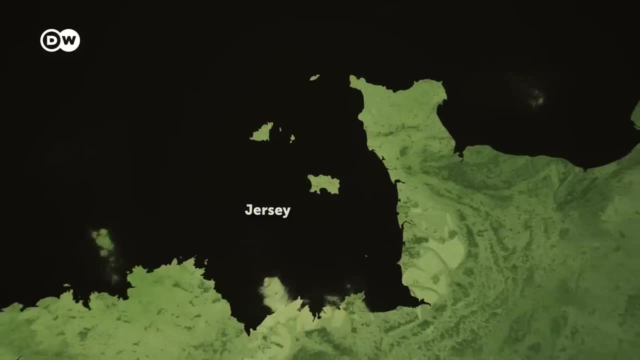 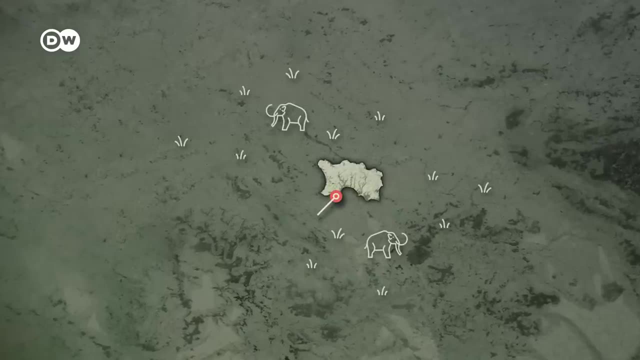 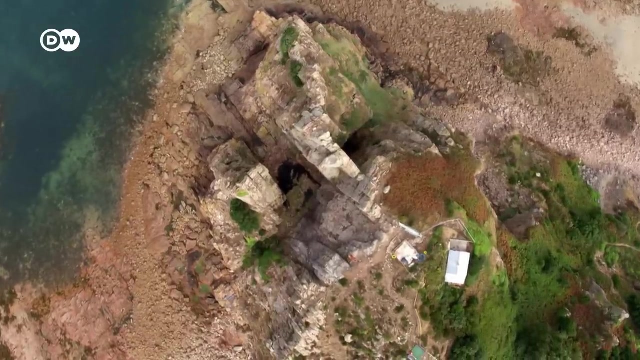 In prehistoric times, Jersey was not an island. It was part of the European mainland. One of its most prominent geographical features is a rock formation that towers 150 metres over a broad plain. Neanderthals may have used it as a lookout post. 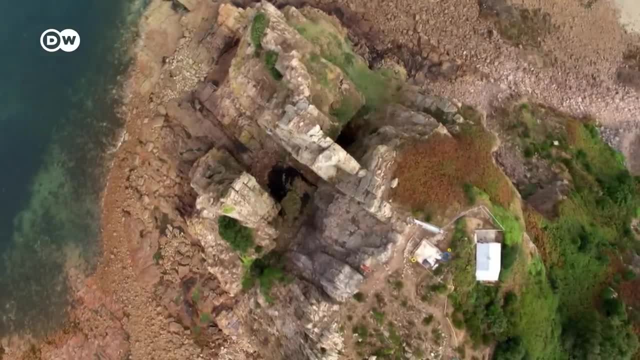 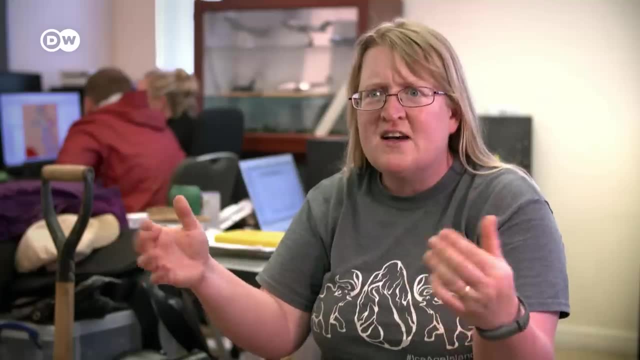 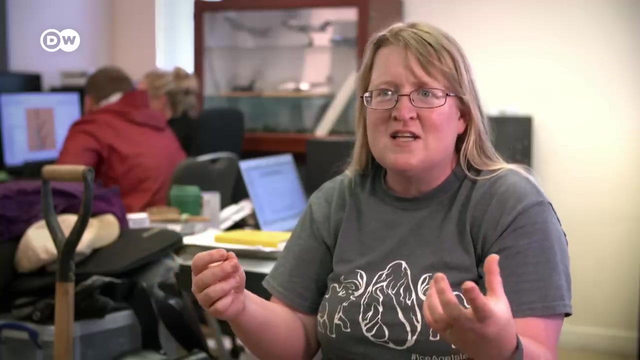 For Neanderthal people. that view gives them control of that. So you can maybe imagine somebody sat up there, perhaps directing other groups, perhaps spotting maybe other people coming through, maybe herds of animals coming through. So by getting up they're actually able to control and work with their landscape in a 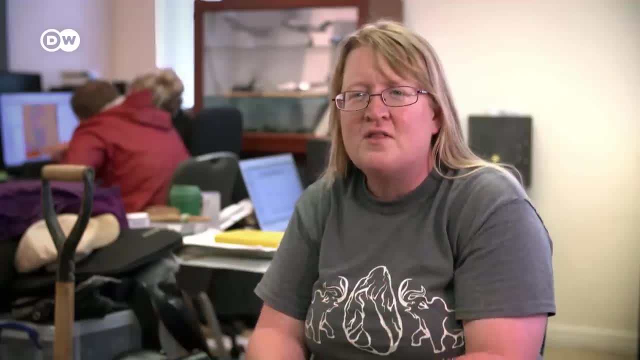 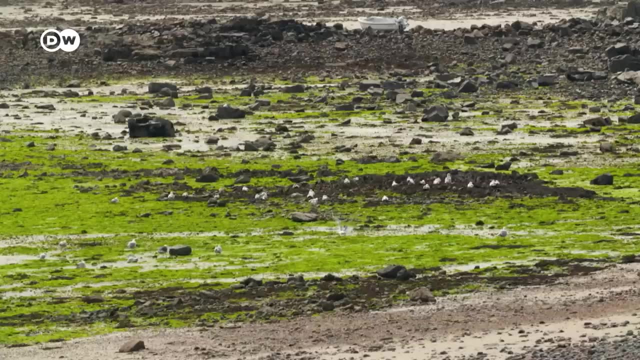 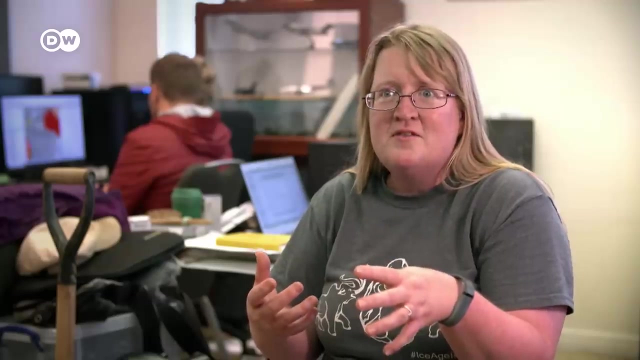 way that you can't when you're just down low and moving through it. Scientists mapped out the ocean floor around the island to find out what the area might have looked like in prehistoric times. A few years ago, my colleague Richard Doolittle, who is a geologist at the University of New 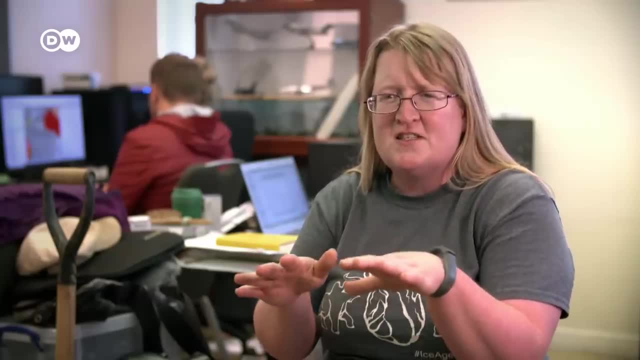 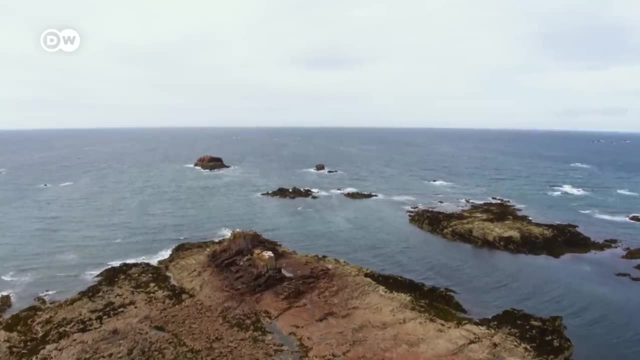 York told me that there was an island there. Richard Bates and Martin Bates actually started to conduct a bathymetric survey of the bay that surrounds Lakot and up to five kilometres off shore. so that was painting in the landscape that we can't see. 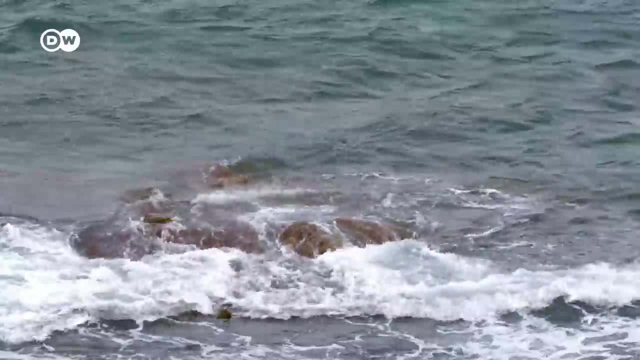 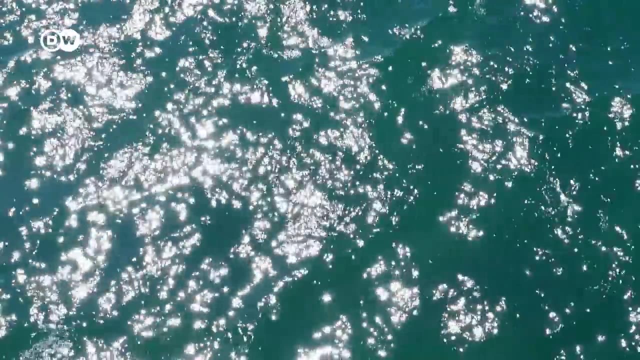 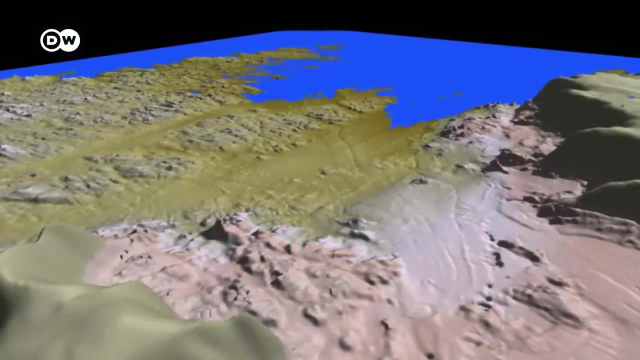 So there's little bits of it that are still visible, as skerries and reefs and eroded sea stacks. The Bates brothers' investigation showed that the seabed was not very deep. They also found canyons where Neanderthals could trap bison wild cattle known as aurochs. 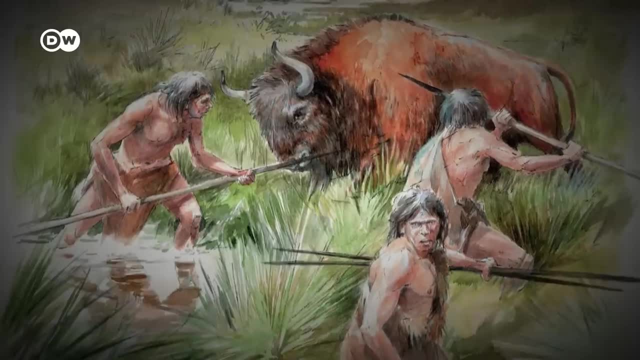 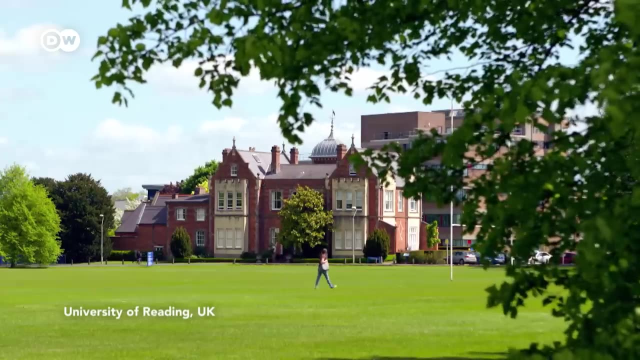 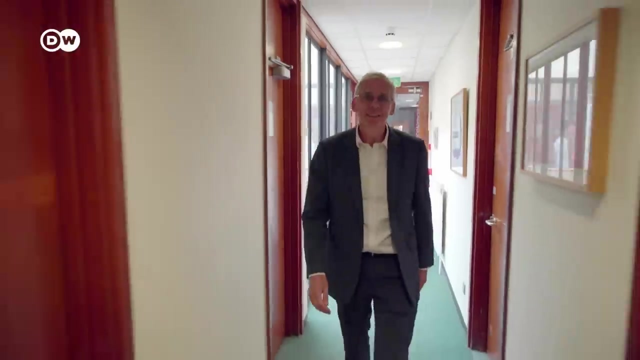 or mammoths. Here at the University of Reading, archaeology professor Stephen Mithen has been researching how early humans learned to develop survival skills and adapt to their environment. Stephen Mithen, Archaeology Professor, University of Reading, New York, USA, I think in many ways the Neanderthals'. 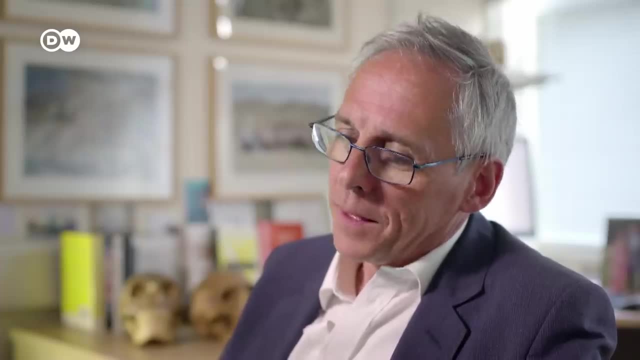 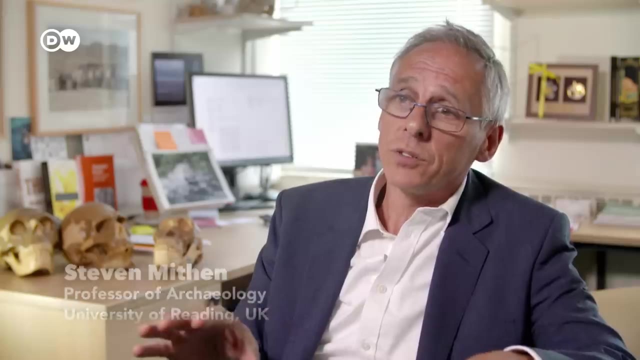 were wild people, but I mean wild in the best sense of the word. They were very sensitive, emotional, caring people, but they were engaged in the wilderness, the wilderness of visage, tundras, of interglacial forests, of coasts, and had a great understanding. 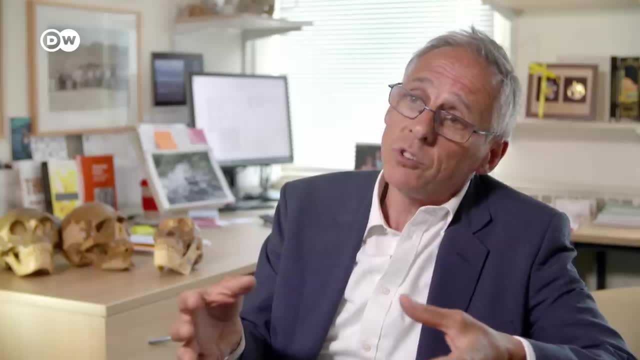 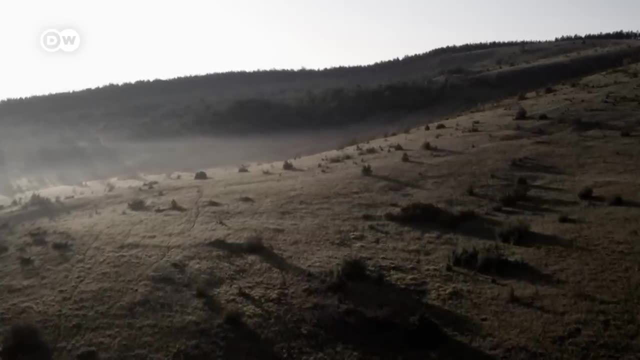 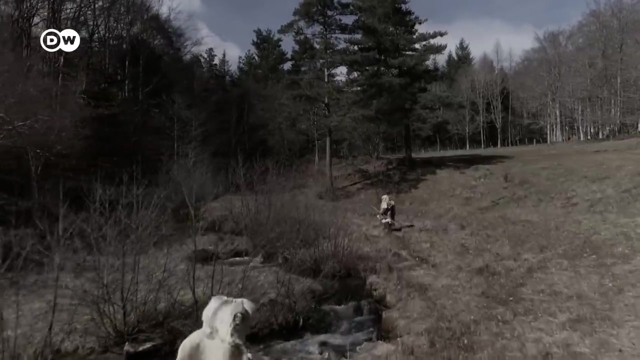 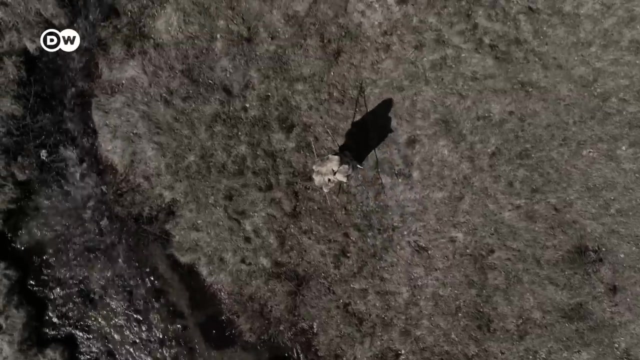 of nature and were very much part of nature in the way that we're not today so much. Rivers and streams were vital to the Neanderthals' survival. They used these bodies of water to help find their way through dense interglacial forests. 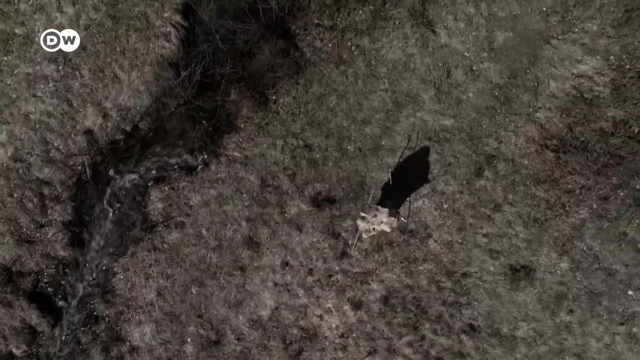 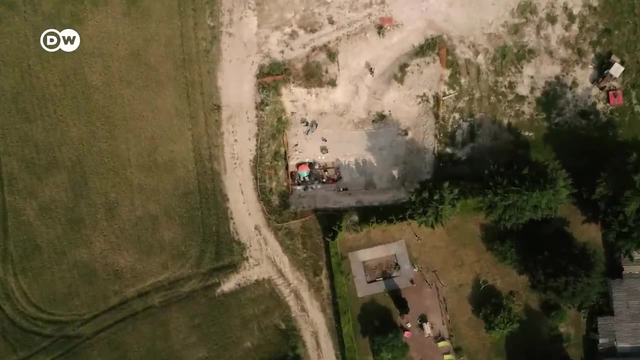 They also hunted animals who gathered there to drink. Excavations at Cahors in northern France revealed evidence of big game hunts that took place there an estimated 120 years ago. The Neanderthals' survival was the most important thing. 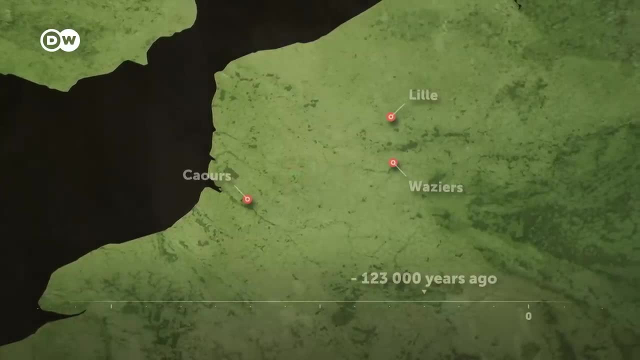 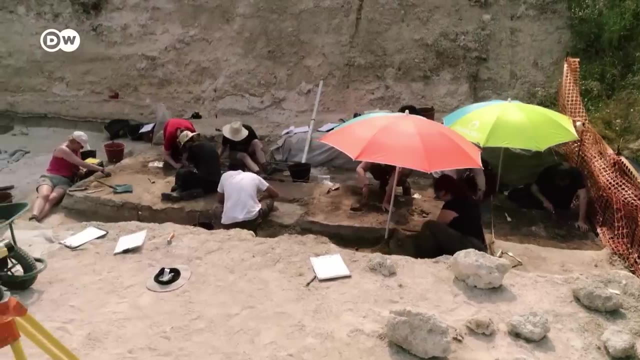 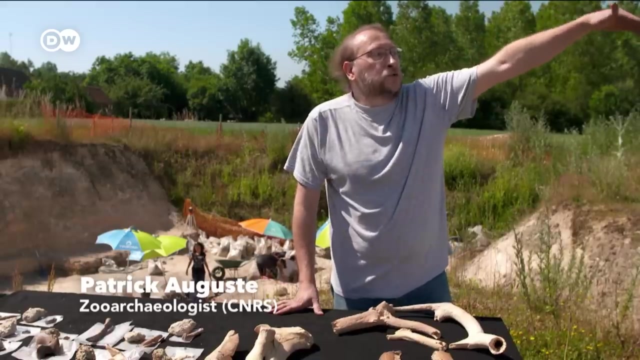 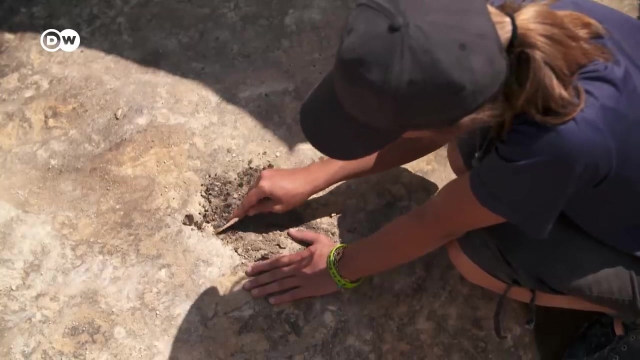 The animals were probably killed on the riverbank. At that time the river was about 10 meters from here, not where it is today. The ground was soft, which made it difficult for the animals to move around. It would have been too dangerous to hunt them on open, hard water. 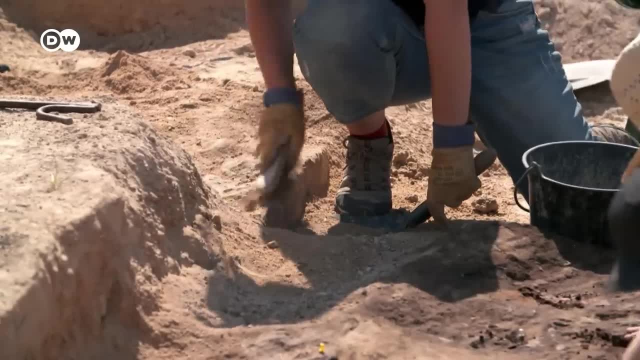 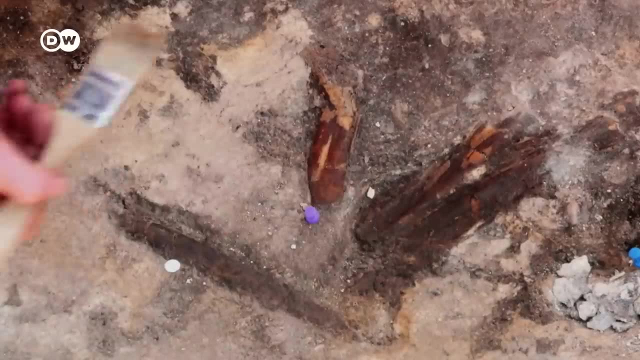 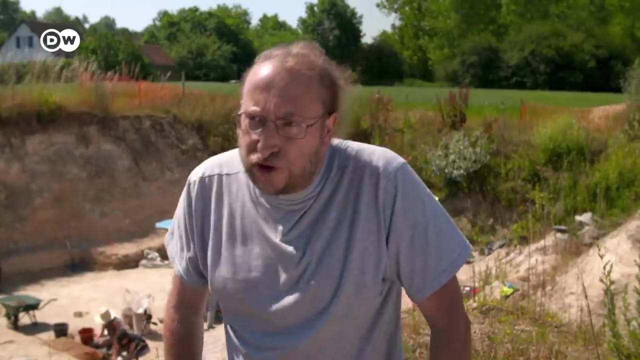 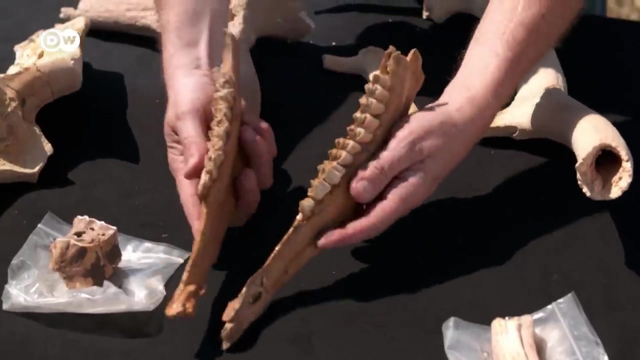 The lives of the Neanderthals were focused on hunting. They developed skills that eventually made them the most dangerous predators in the region. They were expert hunters. We usually associate Neanderthals with sites where the remains of medium-sized animals have been found — various species of deer and reindeer. 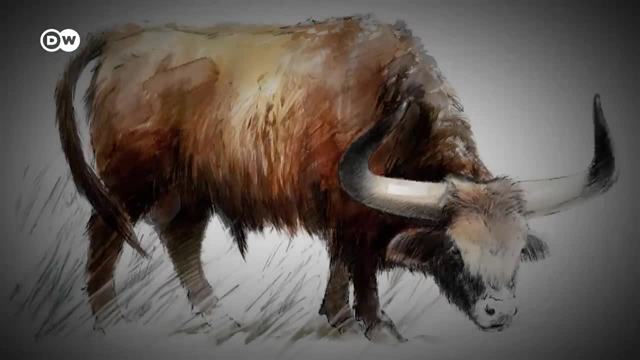 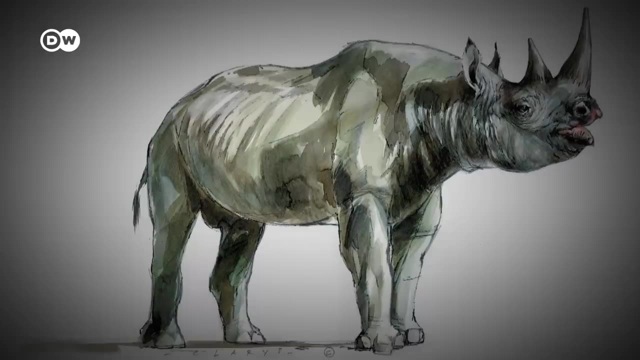 But they were also apparently able to kill wild cattle- which is the reason why we're so happy to see them here- which were nearly two meters tall. The woolly rhinoceros was also huge. They were very aggressive and dangerous animals. 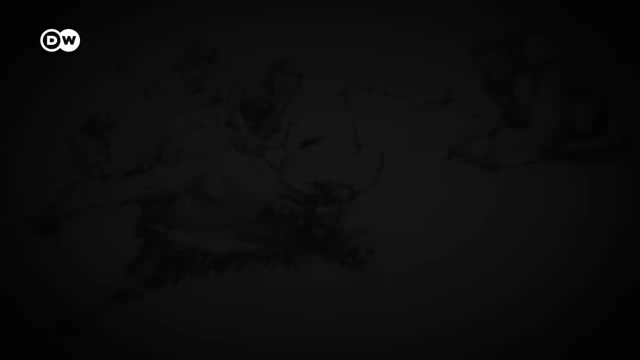 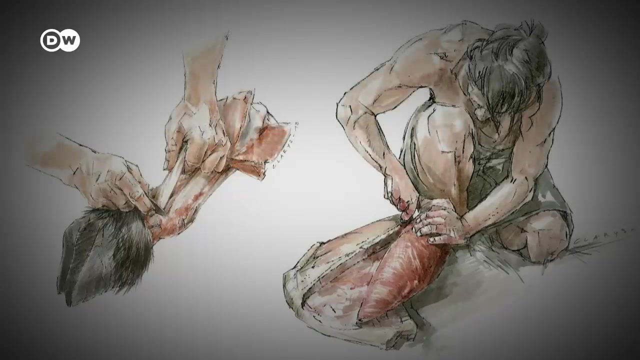 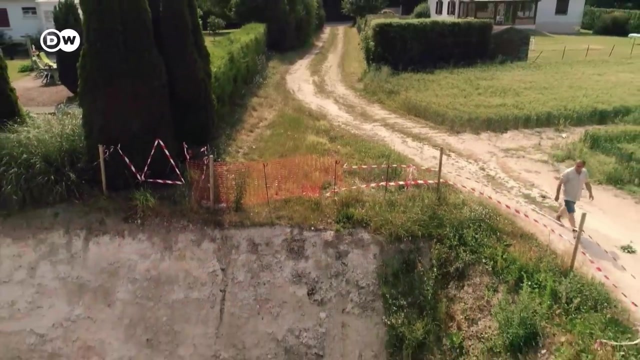 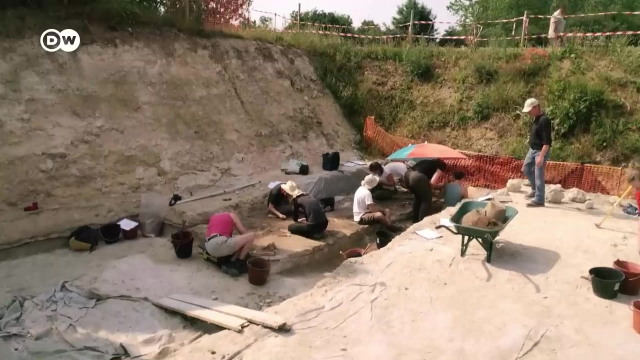 But they also provided a rich source of food, including meat and bone marrow". Excavation director Jean-Luc Locht says the site has yielded important new information on how Neanderthals adapted to their environment, And this has changed our perception of these primitive humans. 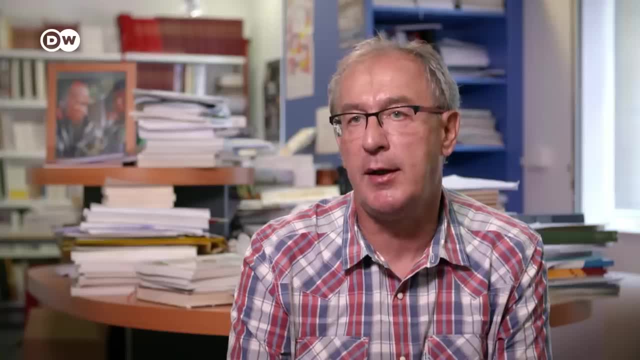 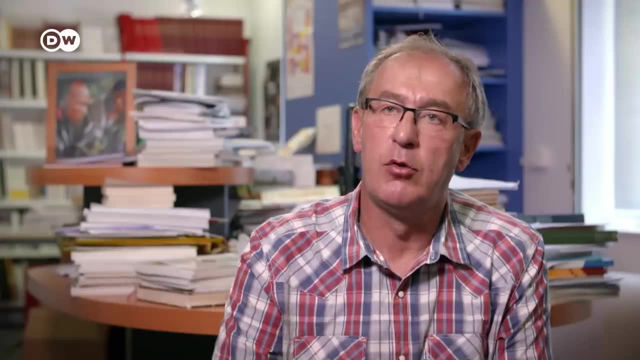 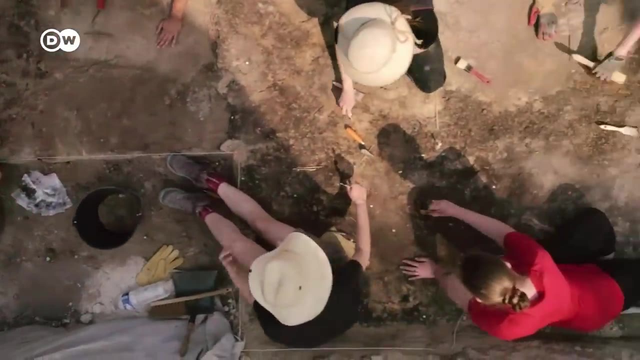 Before the Kaur site was discovered in 2002, experts believed that Neanderthals could not adapt to interglacial environments. It was thought that they inhabited only the colder steppe zones and moved out of our region during interglacial periods. 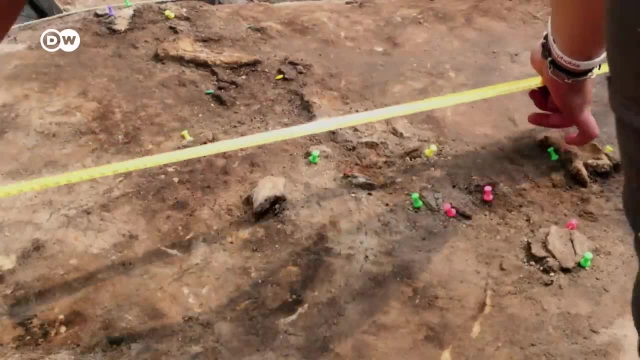 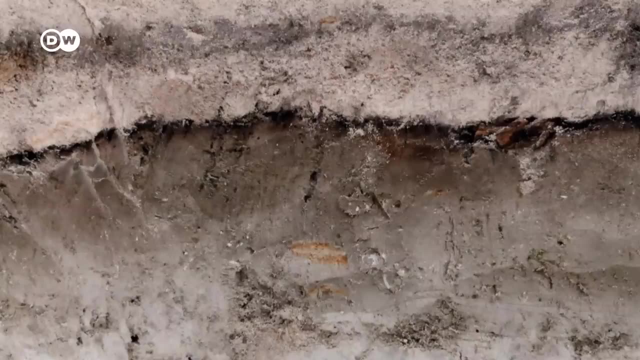 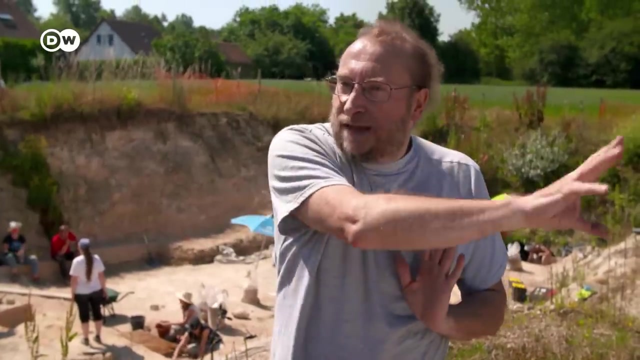 Evidence from the Kaur site indicates that Neanderthals spread their activities over several locations. For example, the current excavation was set up at a place where these early humans butchered the animals they'd killed. This was an intermediate site they used for slaughtering. 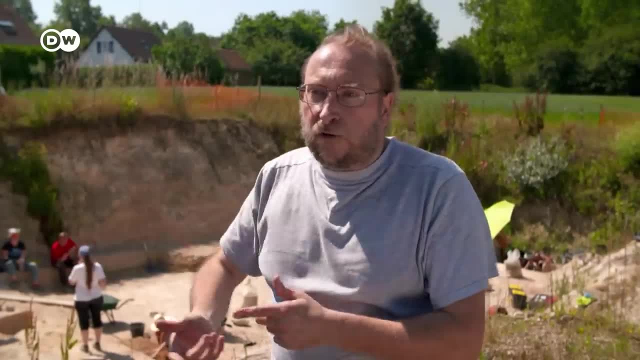 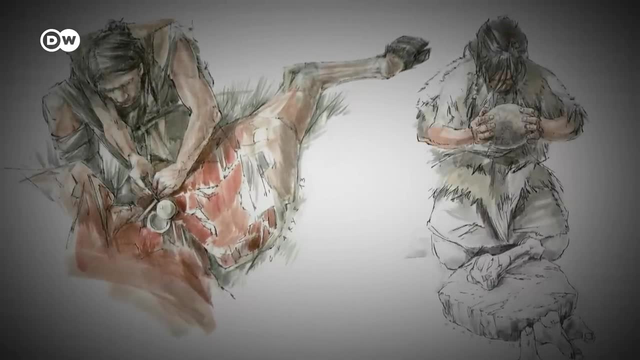 They killed the animals somewhere else and then brought the carcasses here. Afterward they probably took the meat to a base camp that was a little further away. We've recovered a lot of the meat from the site, but we're not sure if the animals 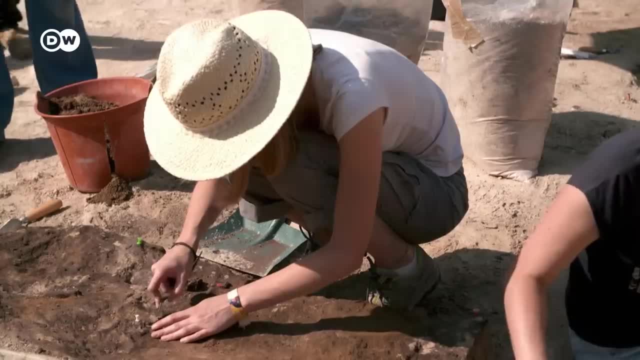 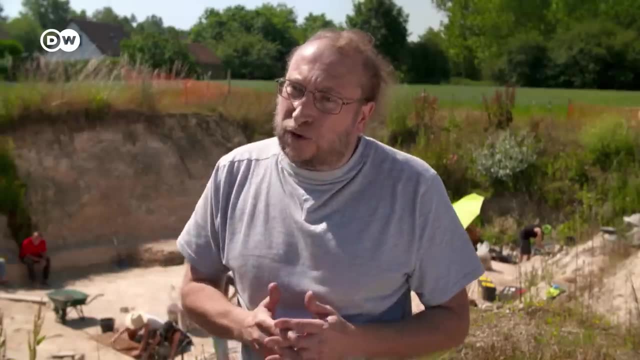 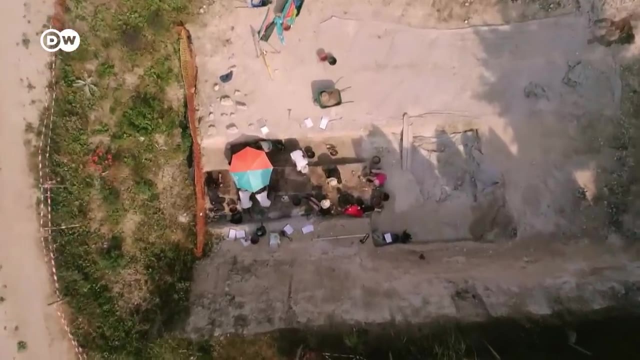 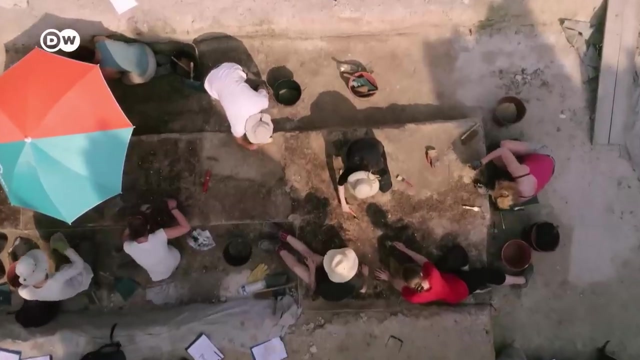 survived. We've recovered items that indicate that these people made their weapons very quickly, without a lot of extra work. The idea was to complete the hunt in what was, for them, a short period of time. Scientists have now determined how these sites were used and how long they were occupied. 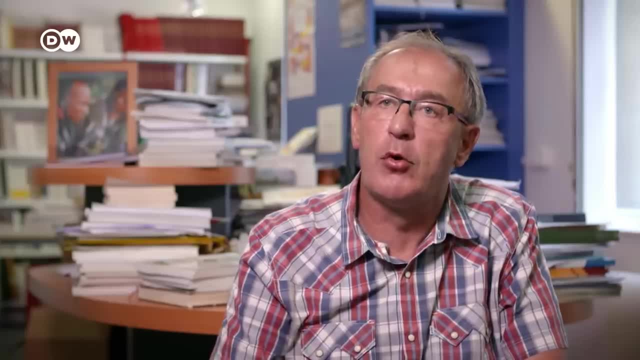 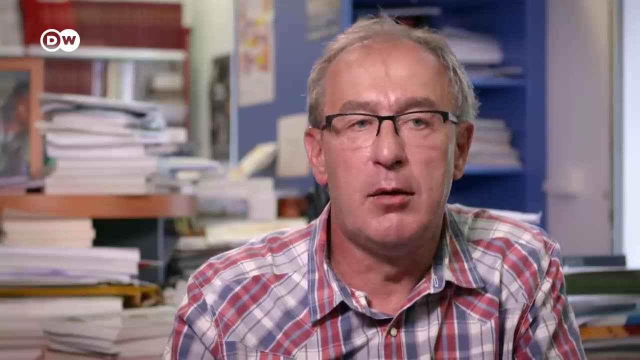 The oldest layer is around 124,000 years old. The most ancient layer is around 124,000 years old. The oldest layer is around 124,000 years old. They went there twice a year. The newest stratum, not better, which is around 121,000 years old, was used for 10 months. at a time, It's clear that Neanderthals were able to adapt successfully to their environment by restricting their activities to specific areas. They were nomads, but they lived in a rather limited region where each site fulfilled fulfilled a specific function, like extracting raw materials or slaughtering animals. 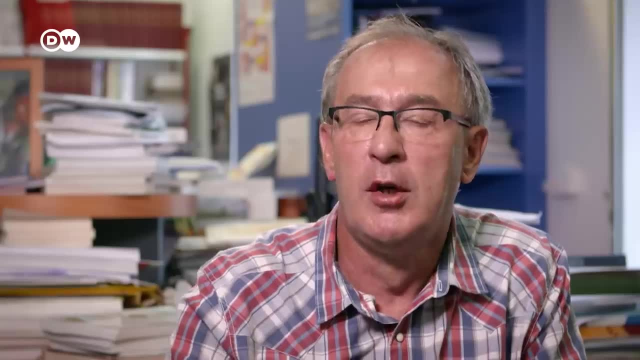 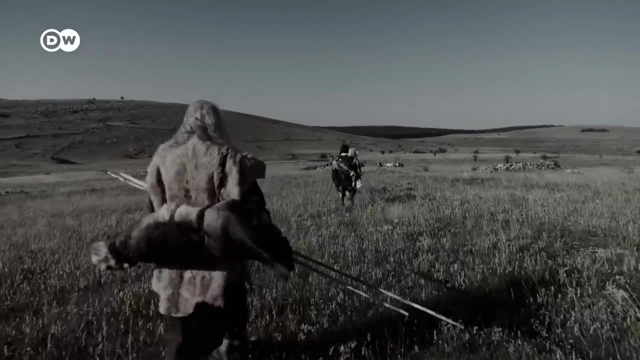 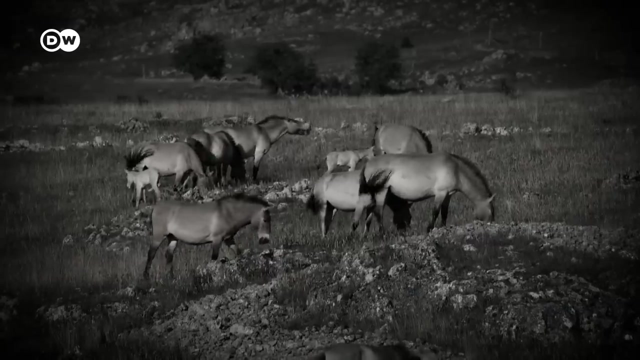 And they created living spaces in sloped areas that protected them from high winds. They knew how to make good use of these narrowly defined areas". Materials recovered from the Kaua site highlight an important feature of Neanderthal culture — their nomadic way of life. 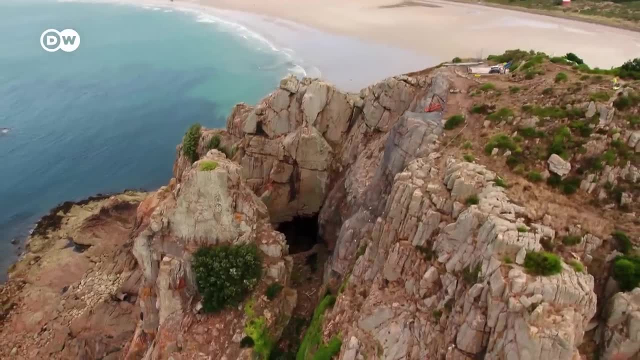 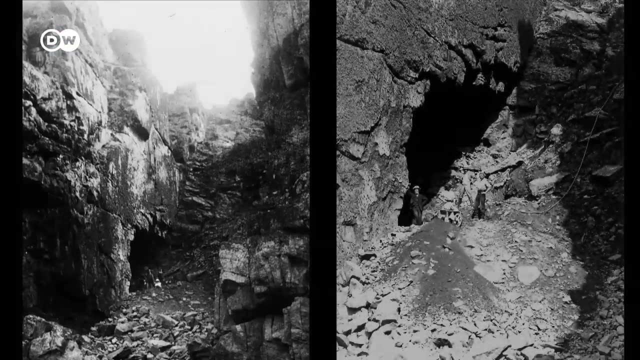 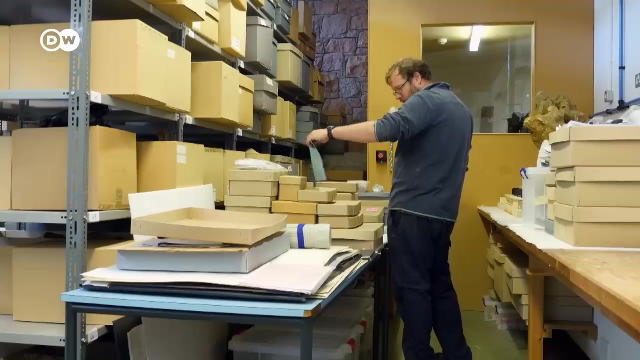 This phenomenon has been confirmed by evidence found at the La Courte site on the island of Jersey. The first scientists who visited the site at the turn of the last century discovered the remains of numerous woolly mammoths. Most of these items ended up in private collections. 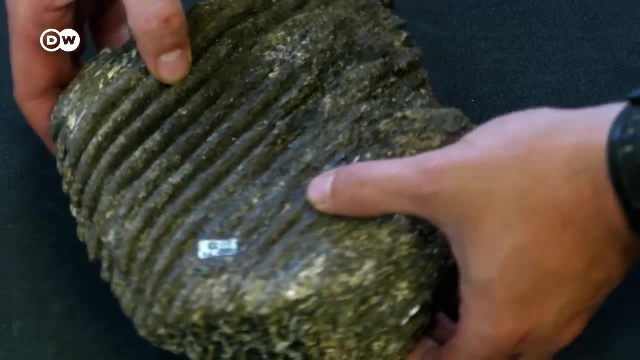 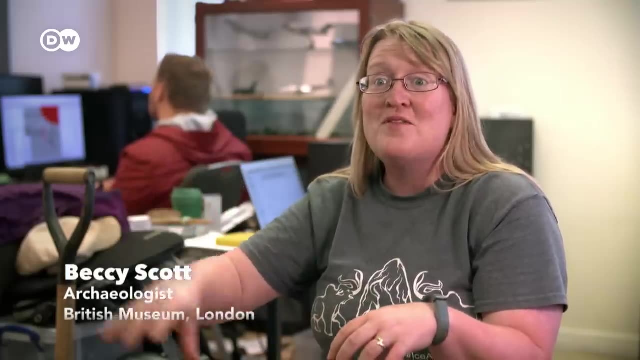 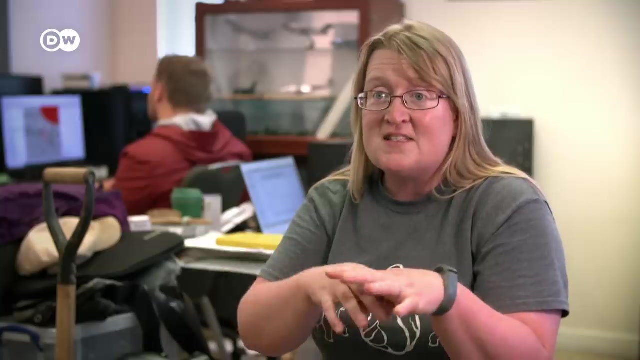 This tooth is the only one that remains in the hands of scientists. We don't know precisely how Neanderthals are found, But we assume that they're probably hunting numbers of them in that landscape, or maybe also scavenging them as well. 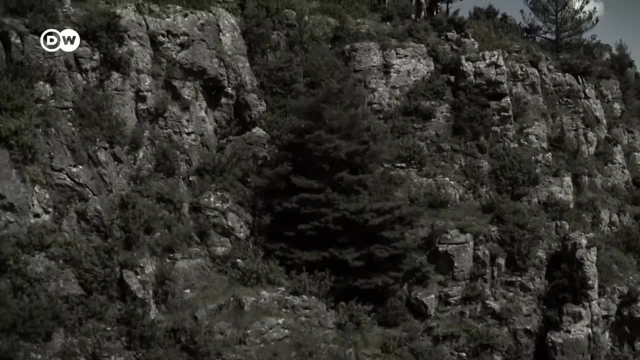 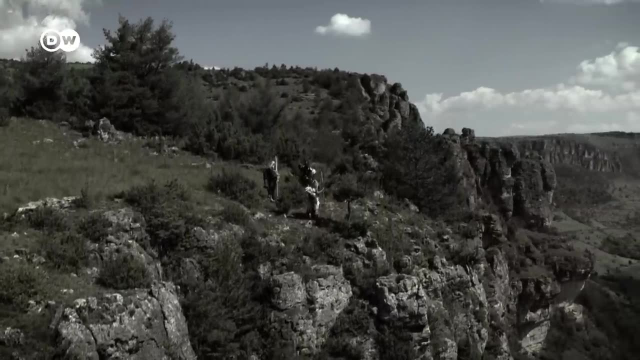 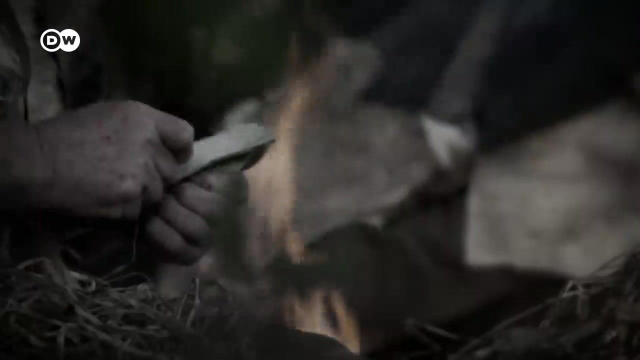 But they're certainly not bringing them in any great distance. The Neanderthal hunters trapped their prey in the rugged Jersey landscape and then used flint-tipped weapons to kill them and flint tools to butcher them, But no items made of flint have been found on Jersey. 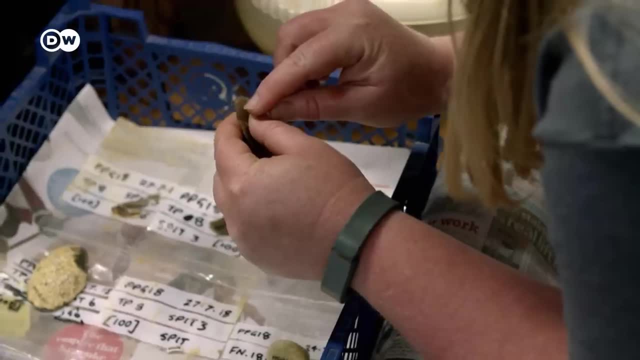 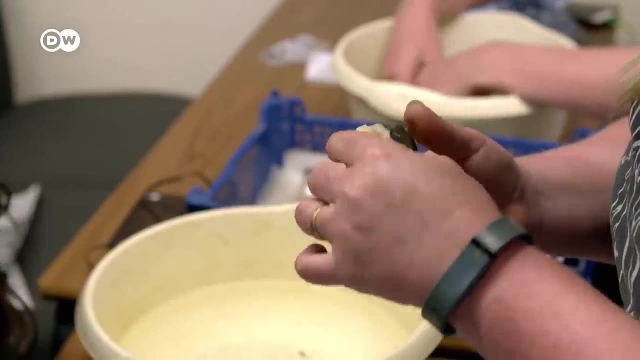 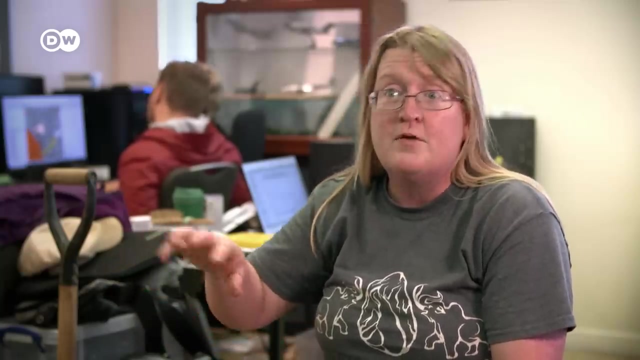 So where did these essential tools come from? We know from the flint that's carried in that the journeys people are making are from maybe 20,, maybe 30 kilometres away from out around Guernsey Alderney. where fresh flint. 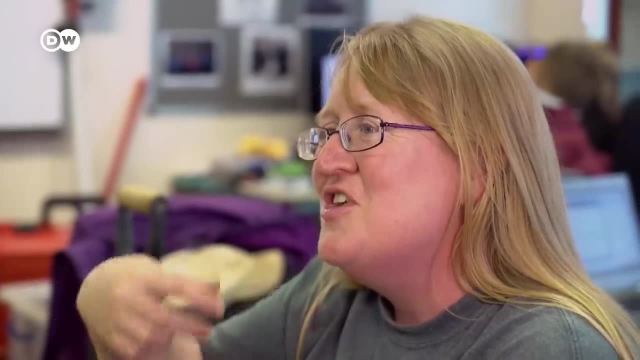 outcrops To make those journeys. you're trying to find an important instrument, I think, if you're not going to be able to make these tools for the future, you're tracking in, maybe over a couple of days. You're carrying your toolkit with you. 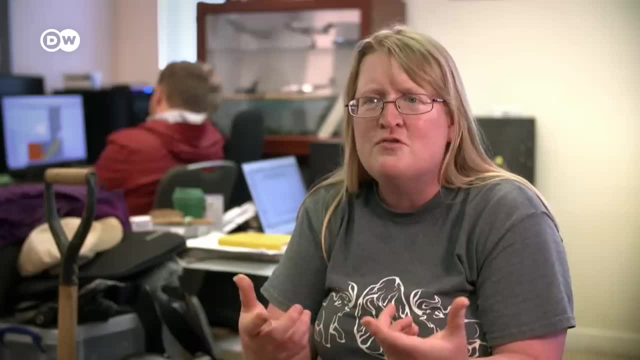 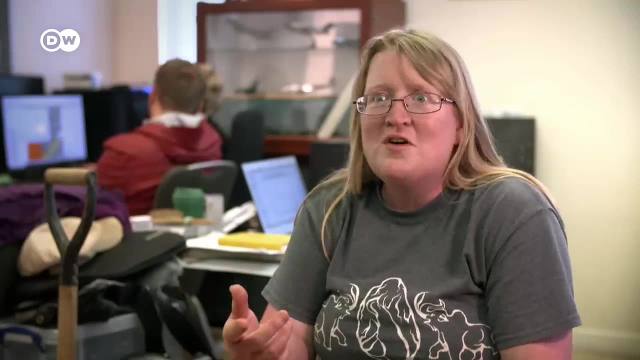 You're working it down as you go And you're not replacing it with local raw materials, So it's like these are deliberate moves to get to places that you know are there. It sort of gives us an insight into Neanderthal geographies. 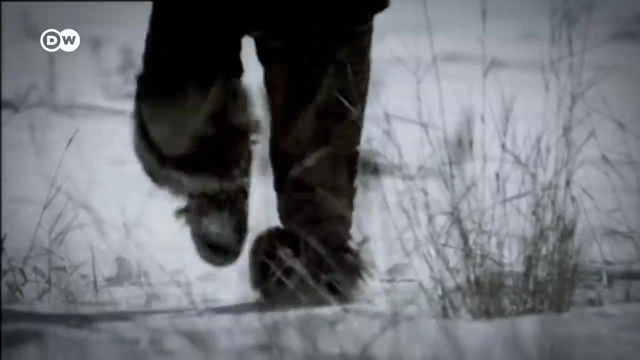 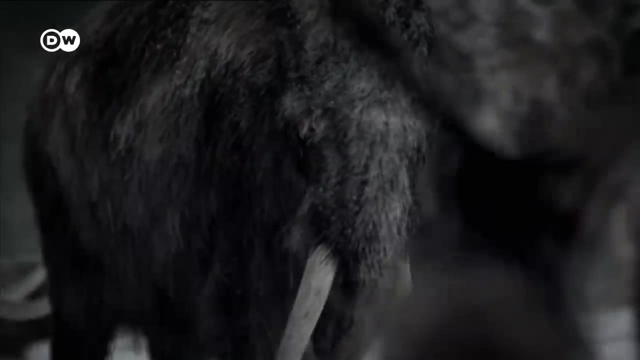 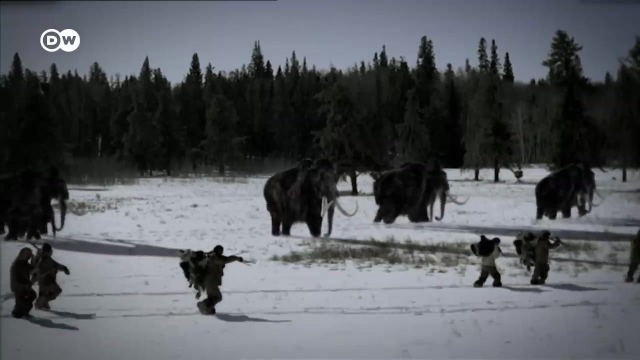 the ways Neanderthals are mapping their world, really. I think Materials excavated at Kaua and Lakot indicate that Neanderthals learned to plan their activities, such as hunting, in areas where they lived. This level of sophistication does not. 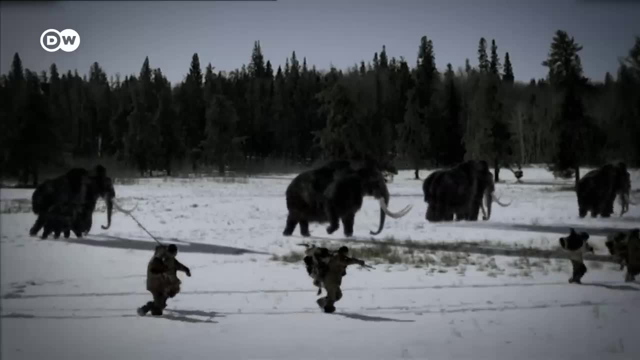 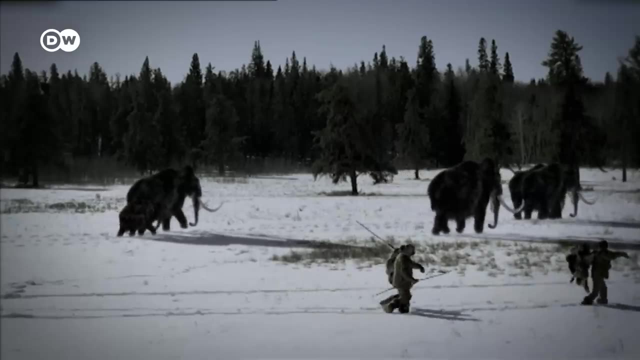 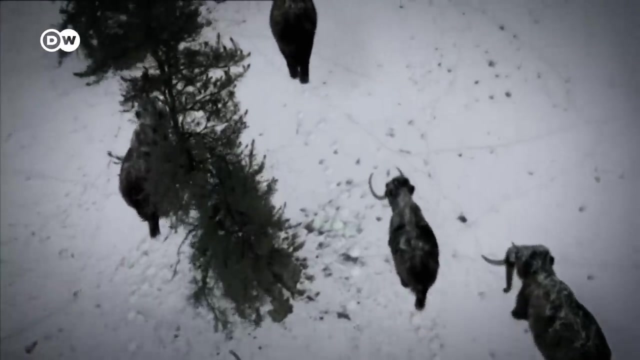 correspond to the stereotype of Neanderthals as crude, low-browed cave dwellers. I think, unquestionably, Neanderthals have undertaken some planning in their activities. We know that they're hunting big game. We know they're hunting mammoths, bison. 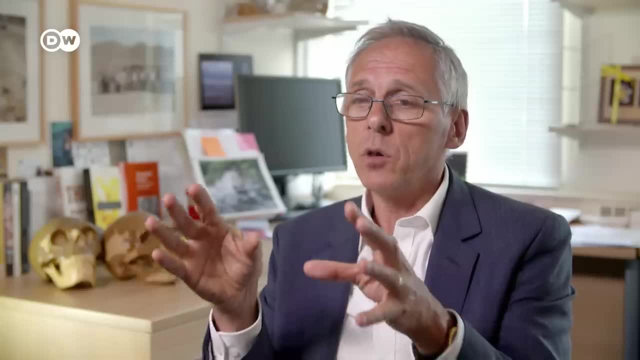 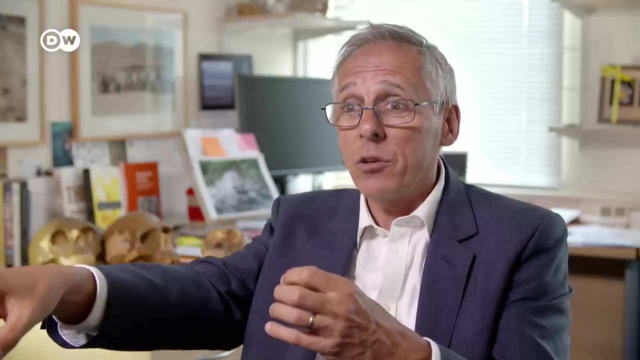 and horse. Now to do that, you have to do some planning for that, because it's got to be a group, cooperative activity. You need to anticipate where the herds are going to be, exactly how you're going to hunt them. 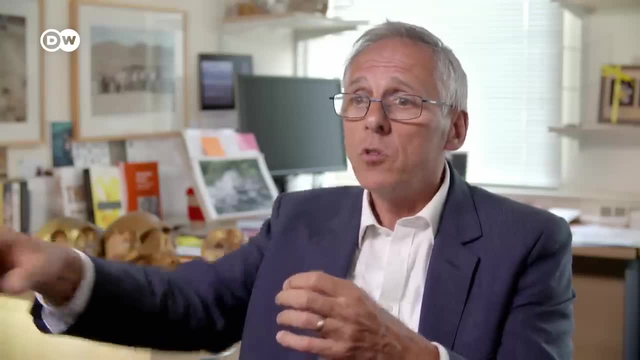 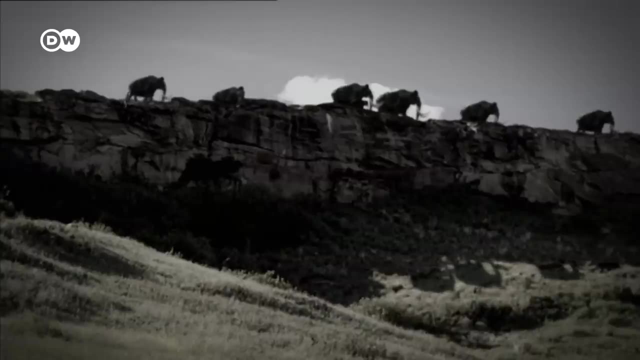 You then also need to plan how you're going to distribute the food and butcher it. So clearly there's got to be planning there. We can just see that from the basic archaeological evidence that we get. Planning allowed the Neanderthals to optimize key activities like hunting. 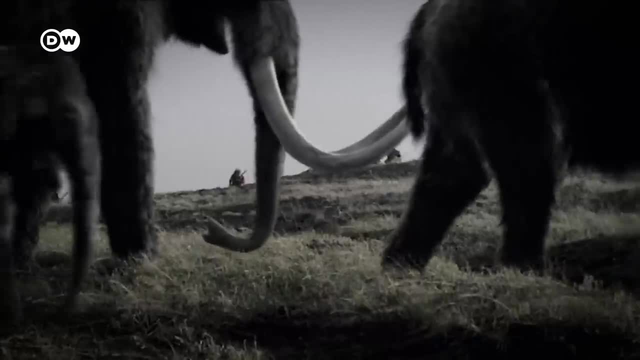 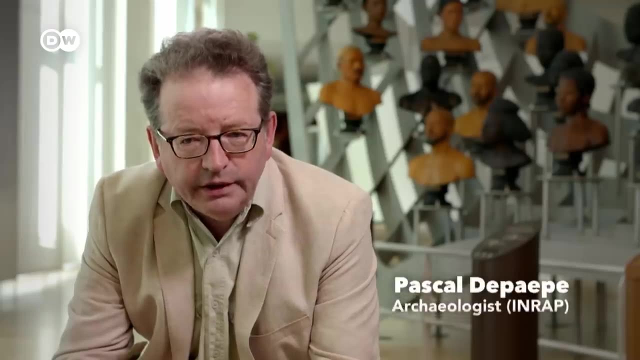 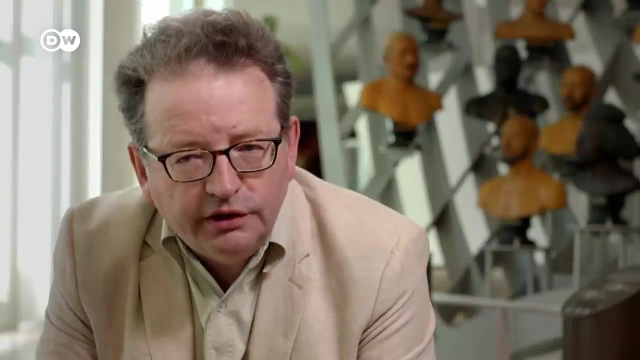 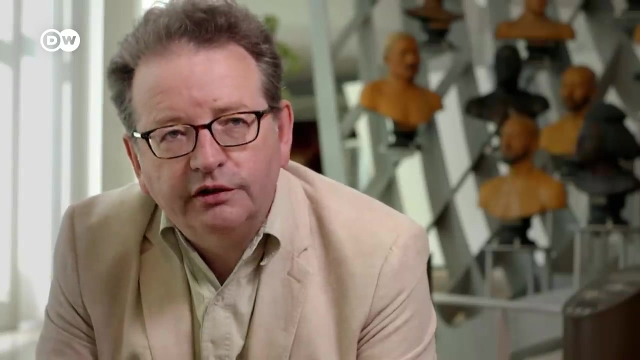 This was an important development, because there were so few of these early humans. It appears that they lived in small groups with perhaps 20 or 30 people. A large clan might have two or three families. These small groups moved over relatively large areas. In all, there were only a few tens of thousands of people in an area the size of Europe. It's unusual that such a relatively small group of people scattered over such a large area kept coming back to places that were far less spectacular than the cliffs of Jersey. 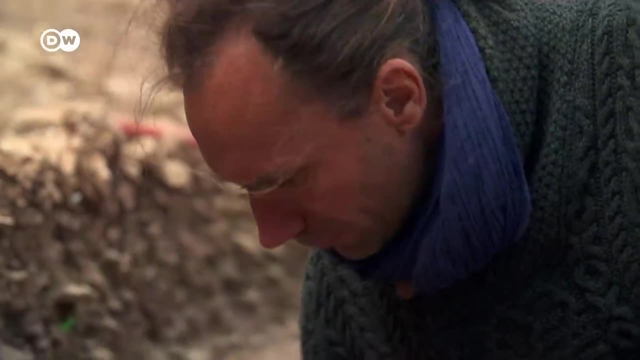 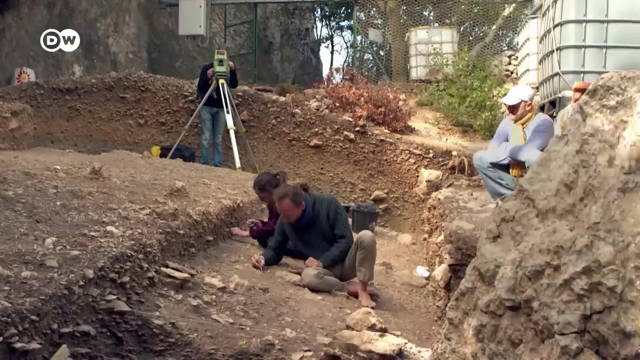 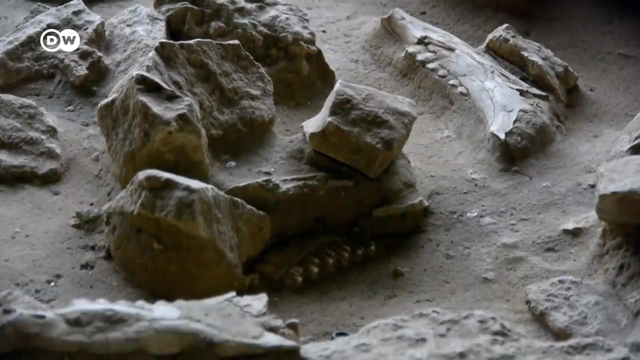 In southern France, excavation work continues at Grotte Mondrane, a cave-like structure on the Rhône River that served as a Neanderthal shelter. Ludovic Slimac is the project leader. He says that the evidence they've found here indicates: 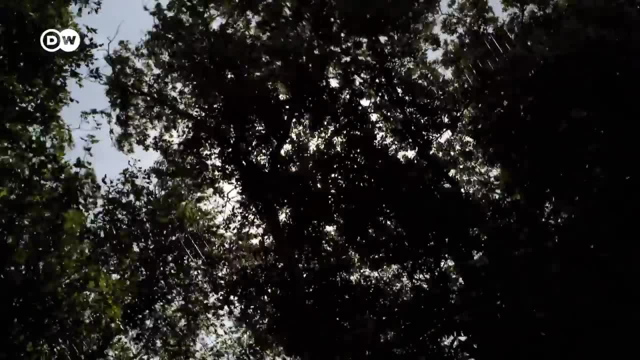 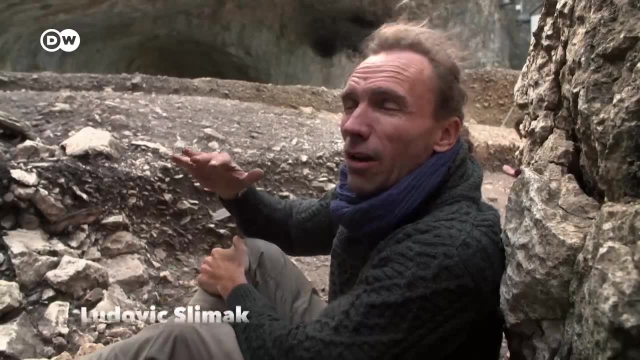 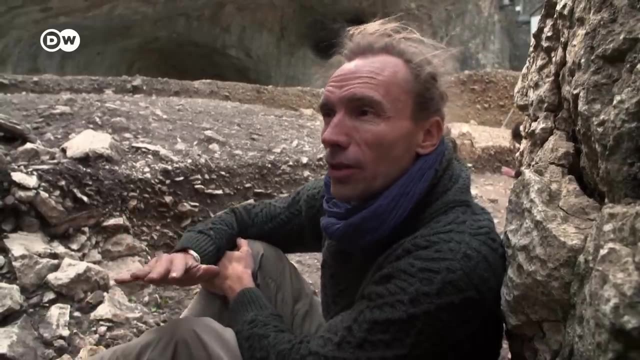 that this was an important stop on many Neanderthal migrations. La Grotte Mondrane faces due north towards the Mistral River, which deposited sediments in the cave over thousands of years. Humans first arrived here 120,000 years ago. 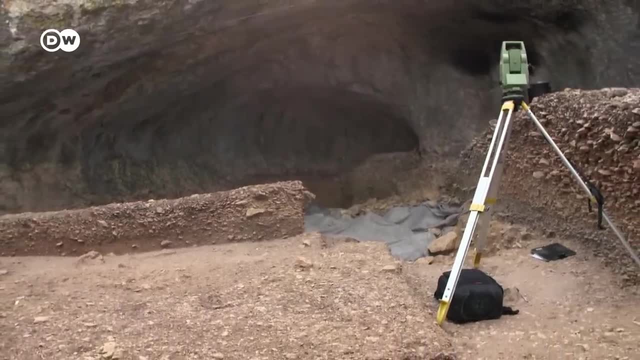 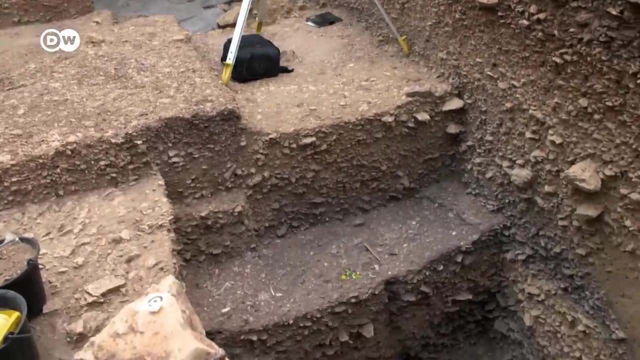 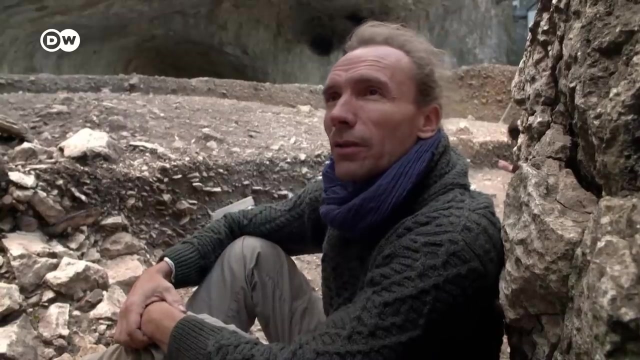 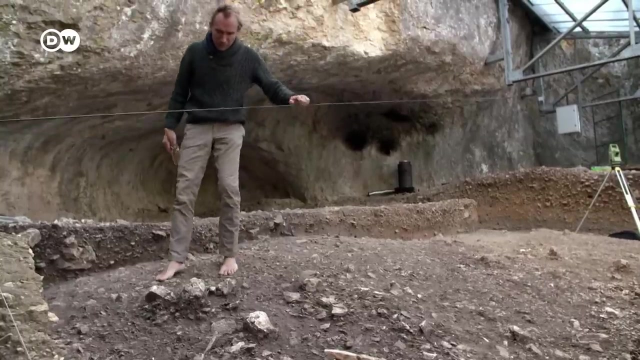 We've recovered items from the cave, but we don't know where they are. It's a marvelous archaeological repository that covers the period from the first settlements to the extinction of the Neanderthals 42,000 years ago. It's the only one of its kind in the world. 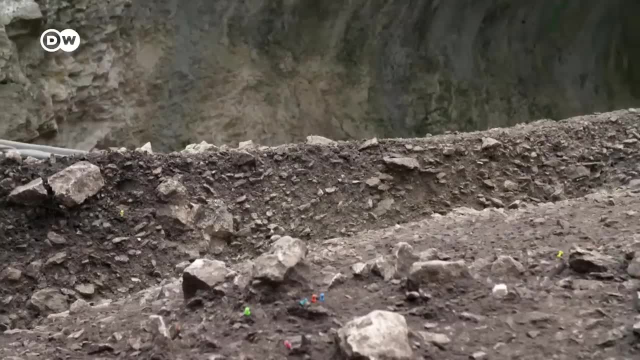 In these layers of sediment, Slimac and his team have found a lot of evidence showing that Neanderthals lived here. This is the first settlement in the Neanderthals' history. This is the first settlement in the Neanderthals' history. 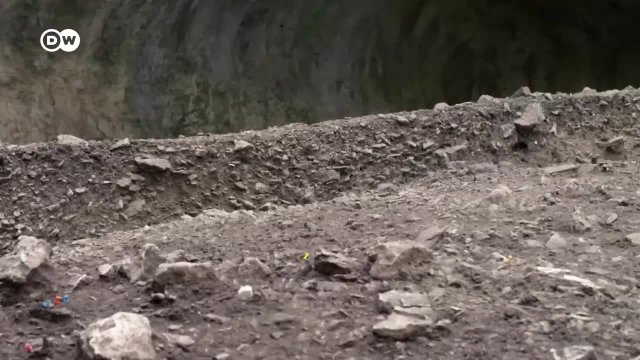 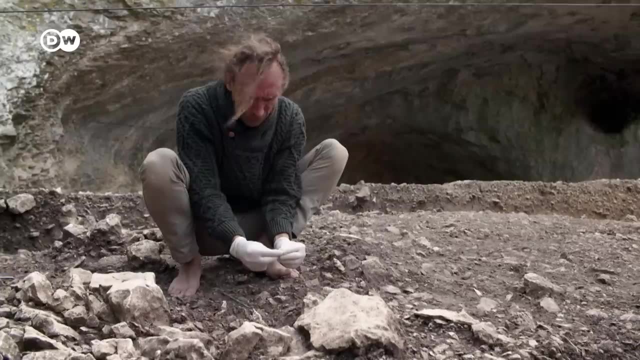 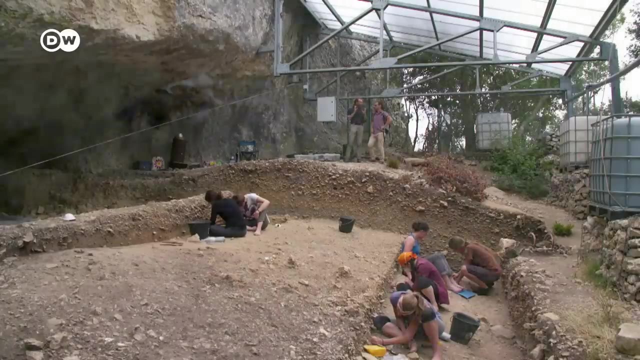 This is the first settlement in the Neanderthals' history. They stayed only briefly, sometimes just a few days, But they apparently came back again and again throughout the course of their existence. Archeologists have discovered gaps of several decades where no Neanderthals appear to have been present here. 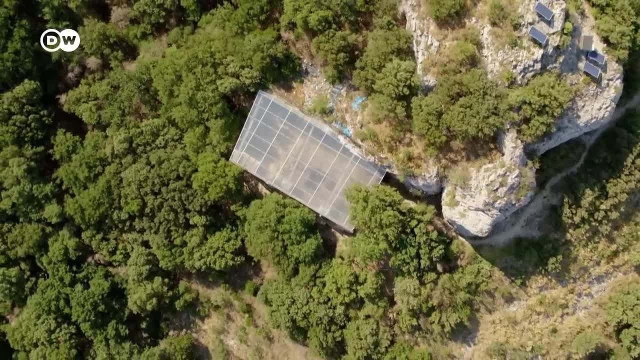 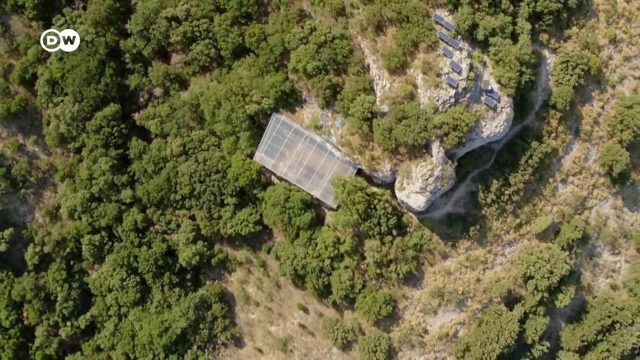 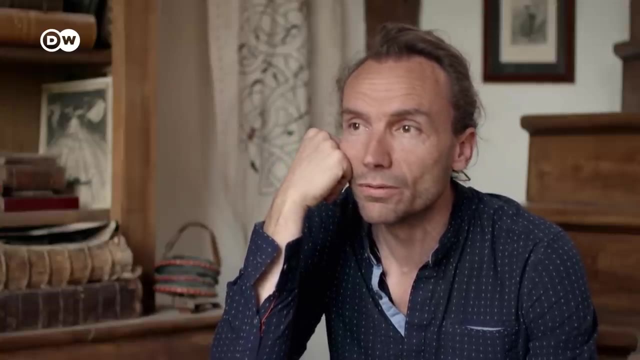 Slimac believes that over 80,000 years, the Mondrane Caves were occupied frequently by nomads, nomadic groups. What makes a Neanderthal a nomad? Did they follow herds of animals Like horses, bison or reindeer? 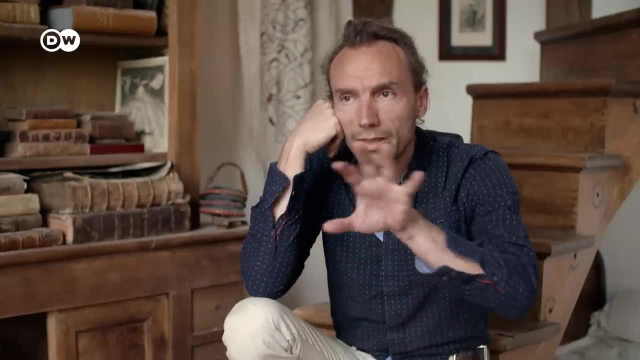 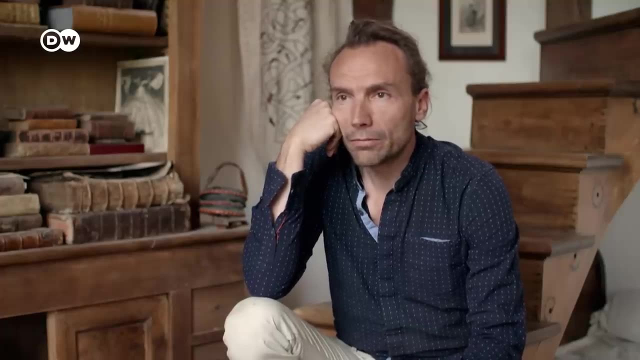 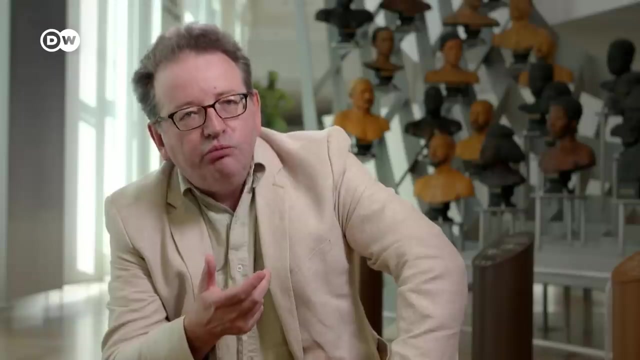 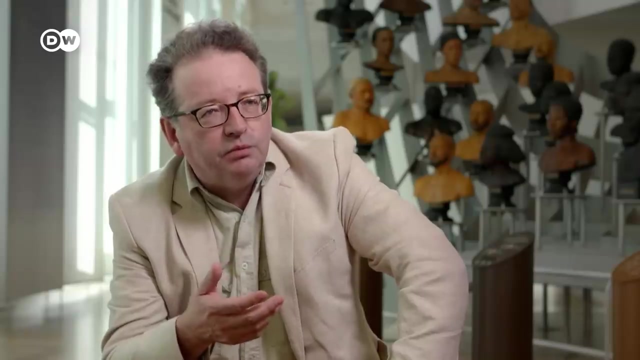 I think that they had good reason to migrate. When we talk about nomads, we mean populations that are thoroughly familiar with a specific area. that could be relatively large. Groups of Neanderthals apparently met regularly in specific places. For example, once a year they'd gather to exchange information and members of their 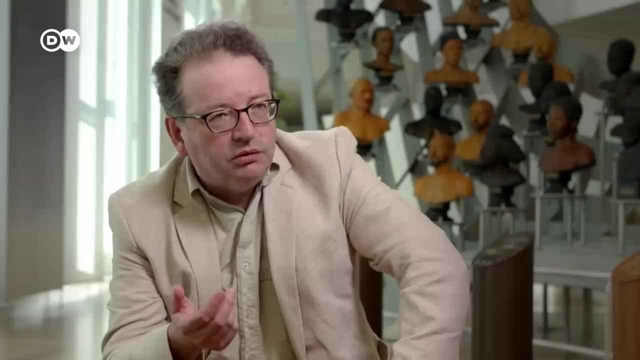 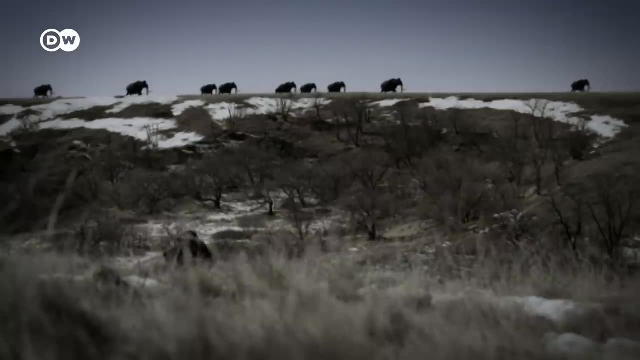 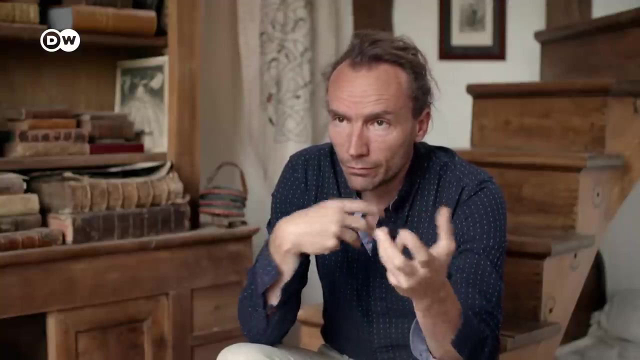 group, especially young people. There's evidence from the Sidrón cave in Spain that Neanderthals also exchanged women at these meetings. They lived together in small groups and reproduced amongst themselves, And that could cause genetic problems. A healthy gene pool needs constant imports and exports of material. 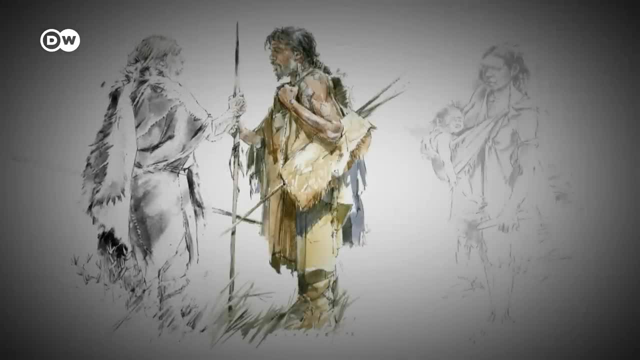 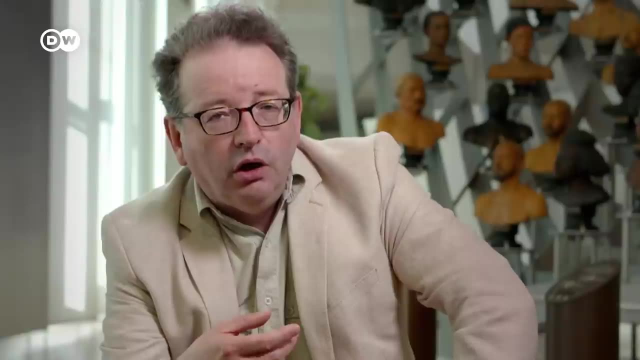 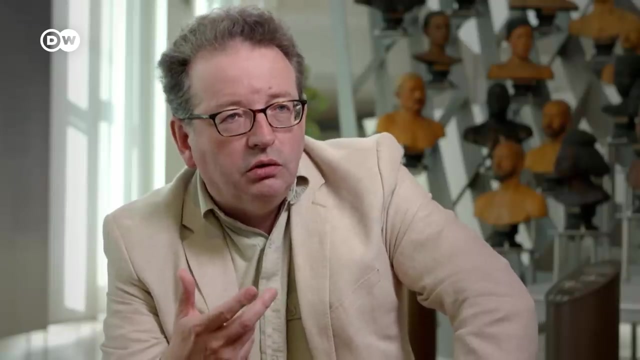 So, for example, I might exchange my sister for someone else's. This would help to enhance the group's genetic continuity. A typical gathering place was La Côte des Cendres-Lades. Various groups met there over tens of thousands of years for the specific purpose of population exchange. 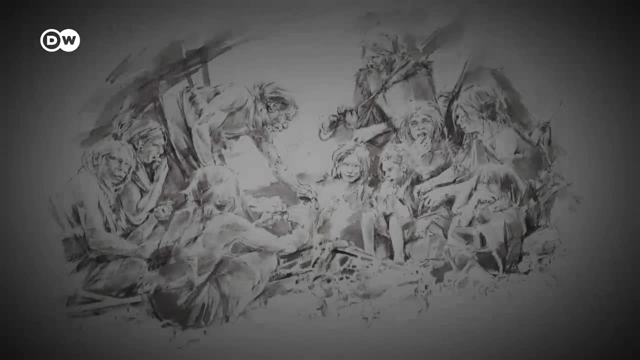 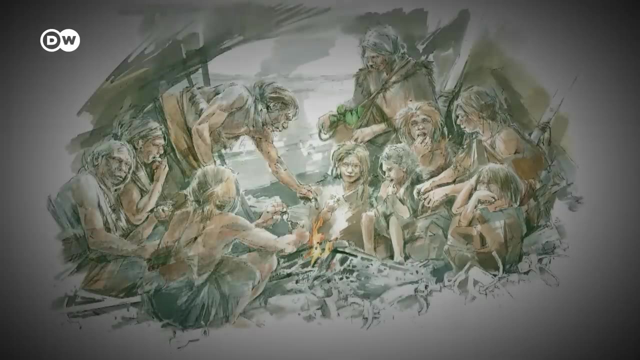 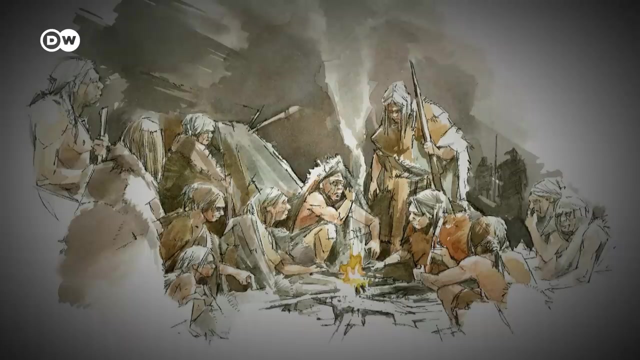 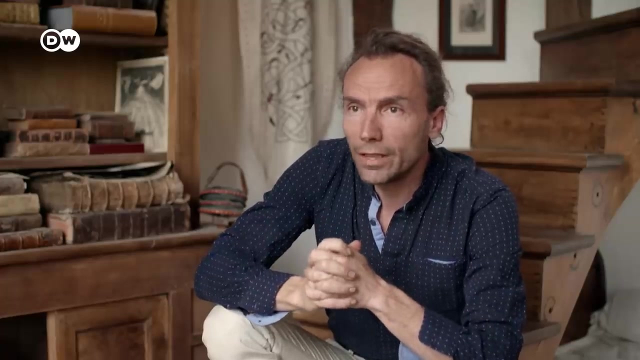 We didn't have an cow. The survival of the tribe was essential. That's also why groups of Neanderthals met, often to hunt migrating wild animals. DETAILS FROM LARGE HIGH LIGHTS. We found evidence that certain objects were transported from far away or in a completely 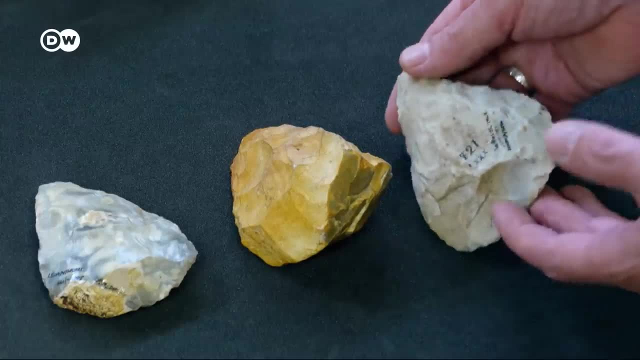 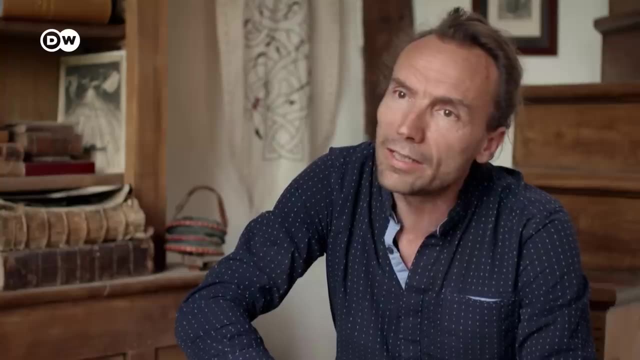 different direction, For example, flints that came from three hundred kilometers far, 300 kilometers farther east, or 300 kilometers farther west or 150 kilometers farther north. It's not possible that one group would cover such a large area in its annual migrations. 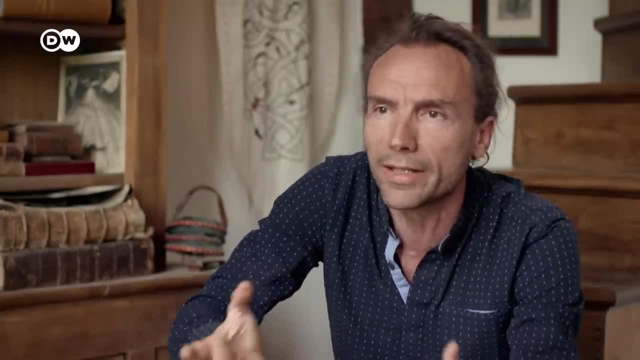 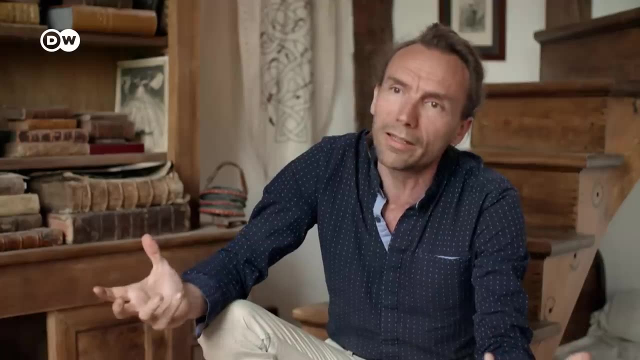 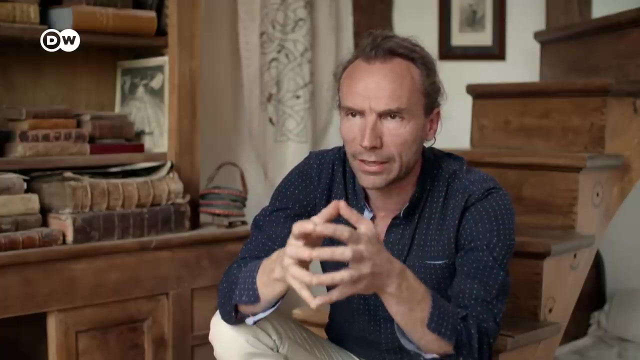 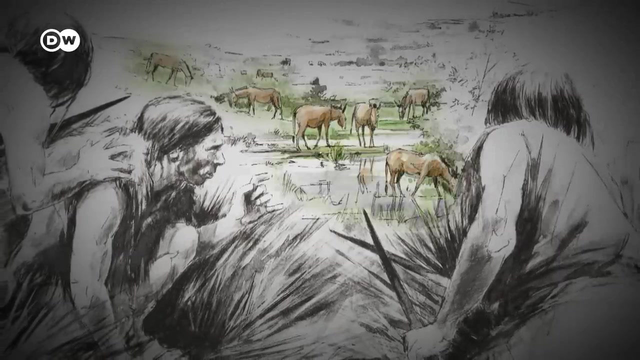 That's thousands of kilometers and it doesn't fit an annual cycle. The evidence indicates that there were several groups and each had its own territory, And once or twice a year they'd meet at one place to engage in common activity. These meetings would produce the desired results only if the various groups could communicate. 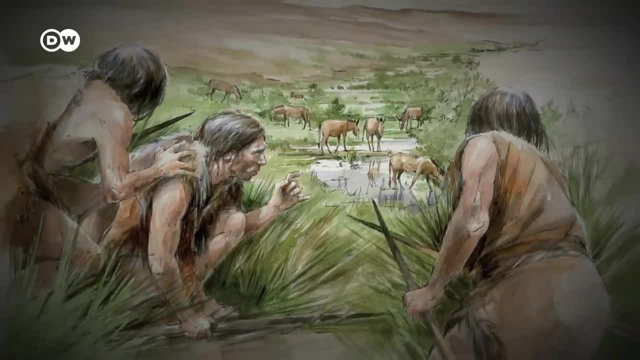 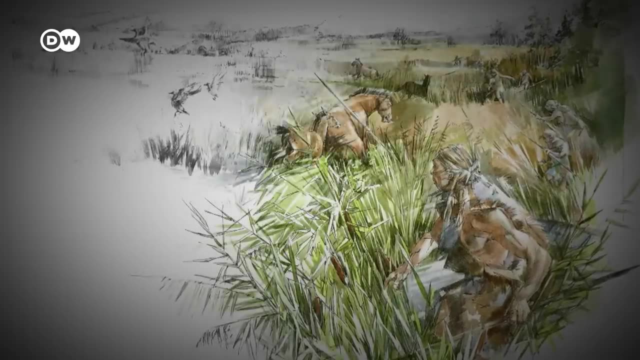 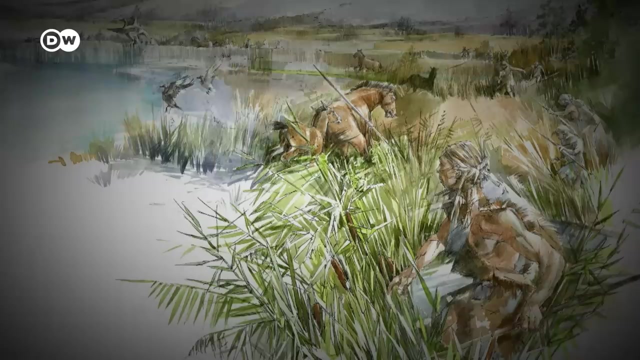 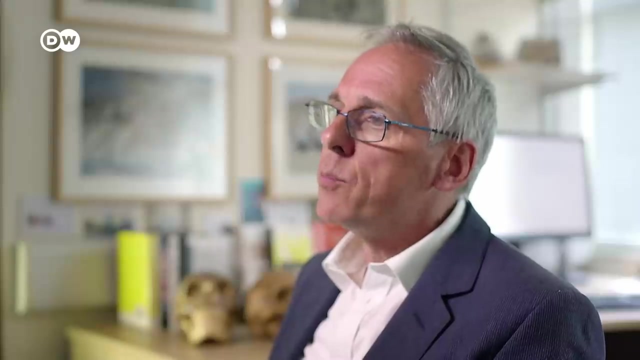 with each other. This raises the possibility that Neanderthals had developed rudimentary language skills … …. … I think to be able to anticipate and plan your social activities, your hunting activities, your foraging activities, must imply a pretty sophisticated system of communication. 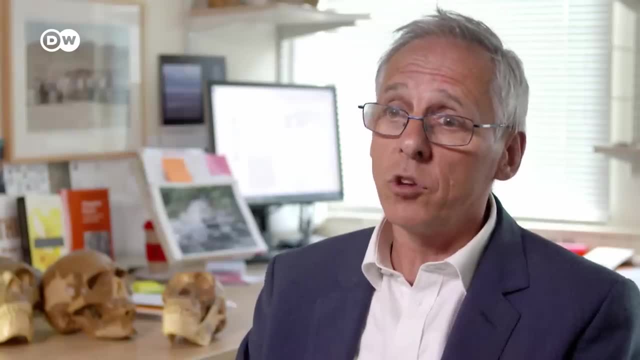 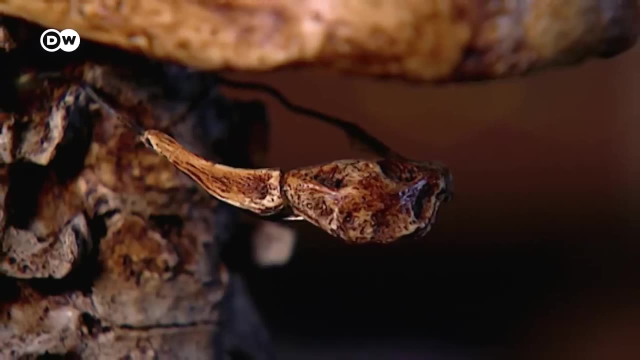 It doesn't mean it's necessarily a compositional language like we have in terms of words and grammar and so forth, but it means a very sophisticated form of communication. Scientists have been studying what sort of language the Neanderthals use to communicate. 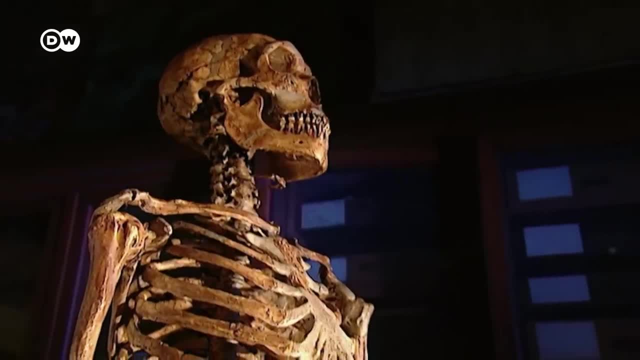 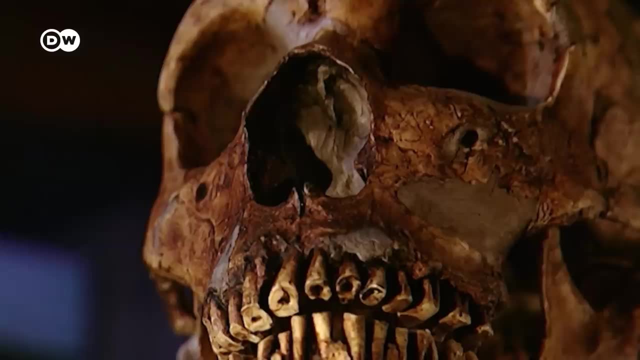 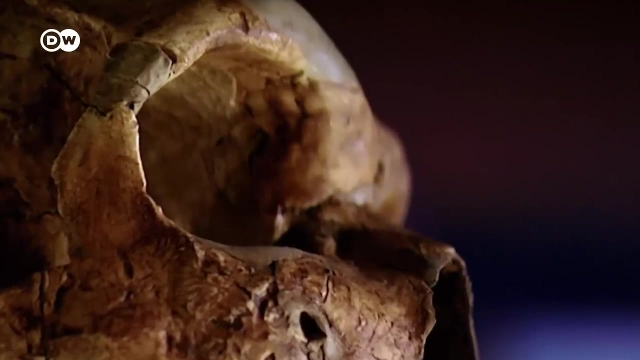 … … … … … … …. In any case, these ancient humans do seem to have had the physical capability to speak … … … … … … … … …. We can reconstruct the basic shape of the Neanderthal vocal apparatus, and it seems. 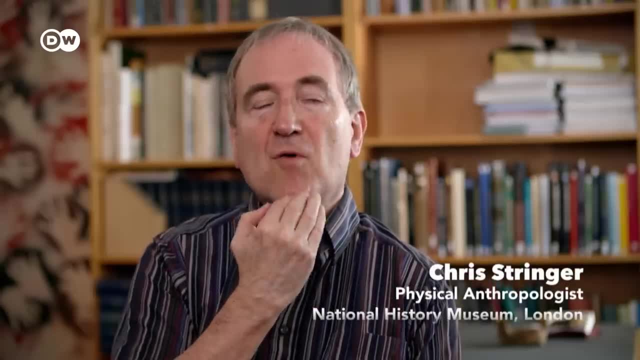 to be fundamentally similar to ours, but maybe the voice box was a little bit higher in the throat, which would suggest the voice was a bit higher pitched. It doesn't quite go with the butcher's voice, but I'm not entirely sure if that's not a. 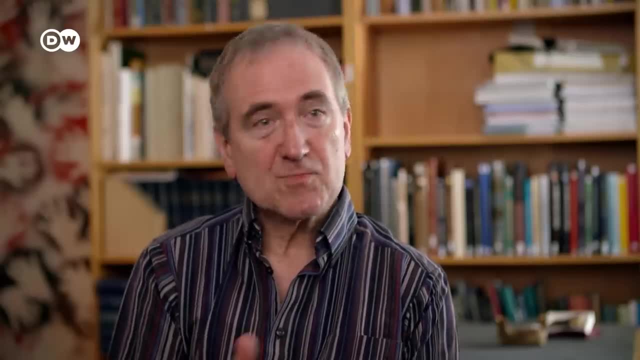 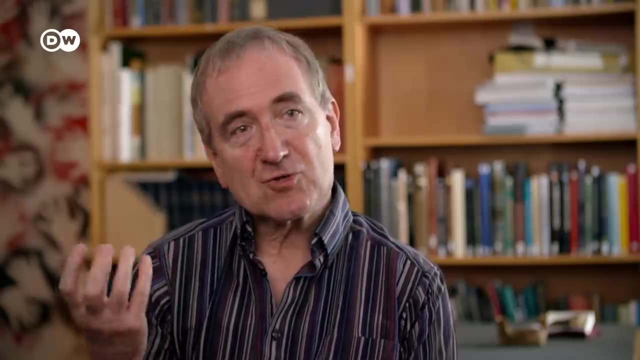 problem butch Neanderthal image of them having higher voices. but maybe they did. But we know that the ear bones of Neanderthals seem to be functioning like ours do for sound transmission, the same range of frequencies, so their hearing certainly would have given them the same capabilities. 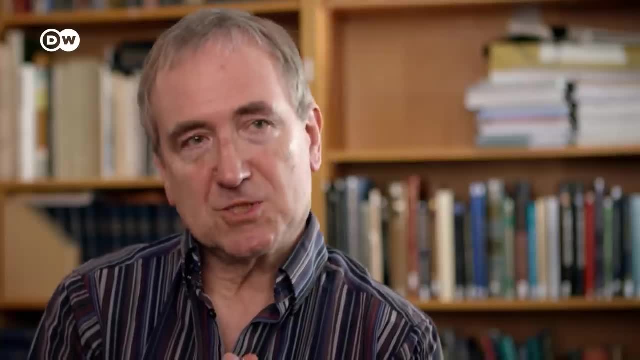 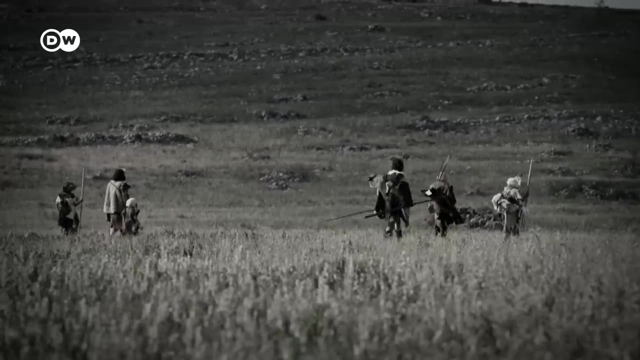 as we have in terms of hearing language. So I think all of that suggests Neanderthals had a basic language. They'd be talking to each other, they had speech capabilities. So it seems likely that Neanderthals were able to communicate with each other, But did. 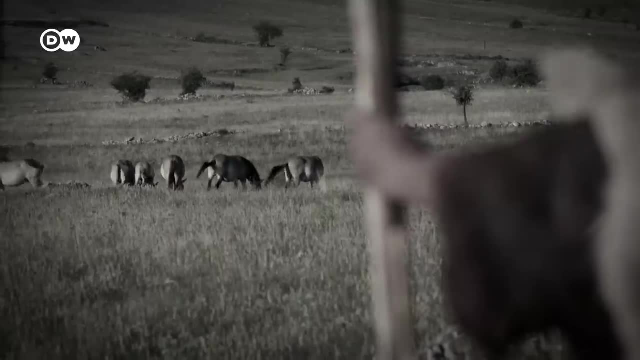 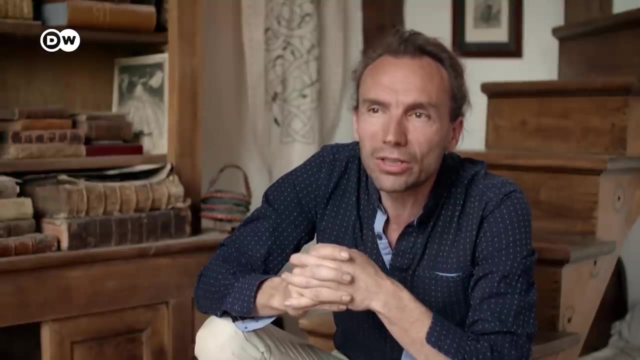 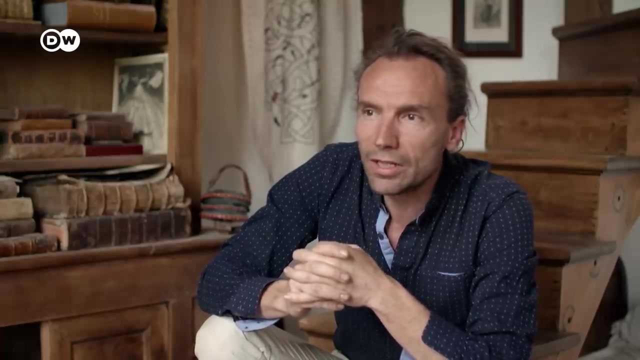 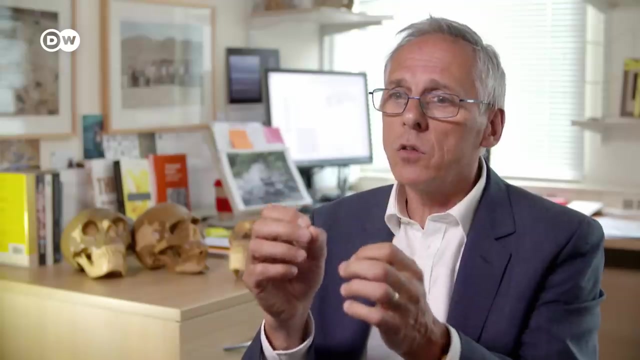 they use language in a form that modern humans would recognize. They did communicate, so they did have language capability. It was a complex and sophisticated form of language that allowed groups to exchange information with each other, And that was crucial to their survival. The crux of Neanderthal language is that it was a complex and sophisticated form of language that allowed groups to exchange information with each other, And that was crucial to their survival. 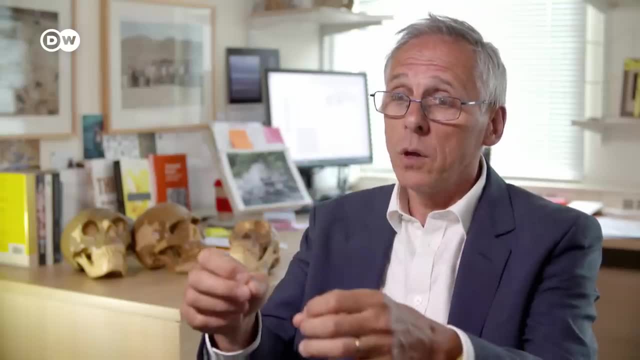 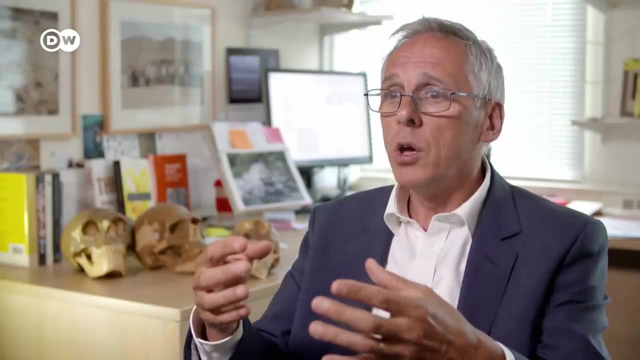 While making the game, they had a complex command: vampire system, human databases�rá. they used words in the way we use words, And those words were then combined with complex grammatical rules or syntax to be able to convey complex ideas or narratives: information. 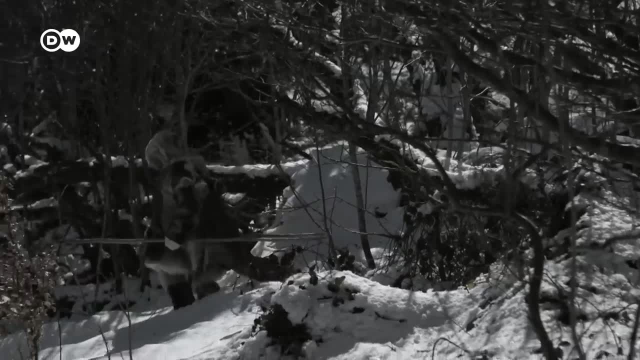 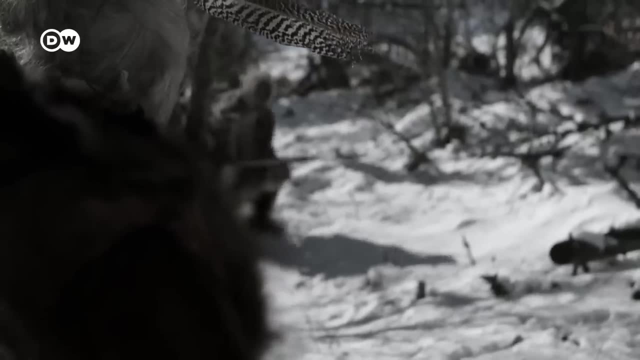 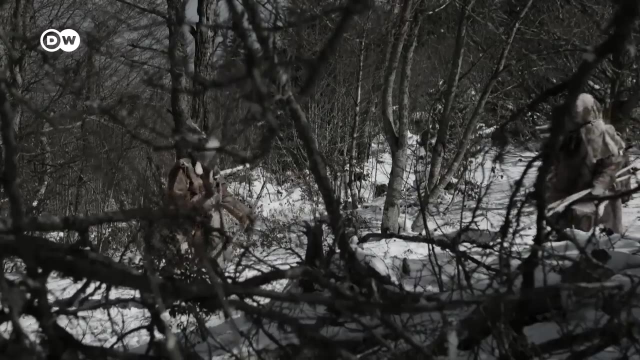 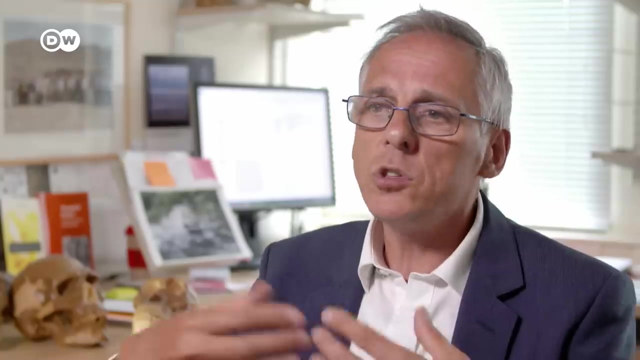 Now, I suspect not. Still, Neanderthals were able to communicate among themselves, but what reading not make form, did this language actually take? I think musicality is really important. Musicality is hugely important for expressing emotion. It's hugely important for social bonding as well. If you go off hunting a bison, we're. 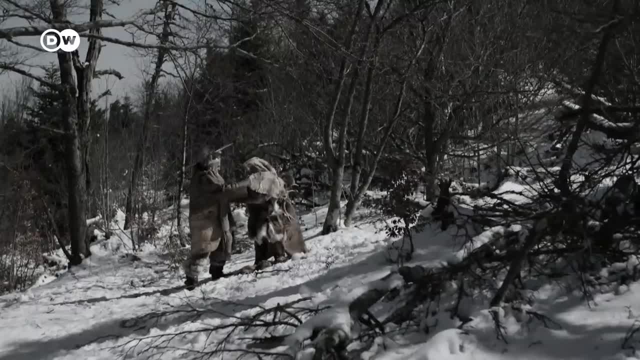 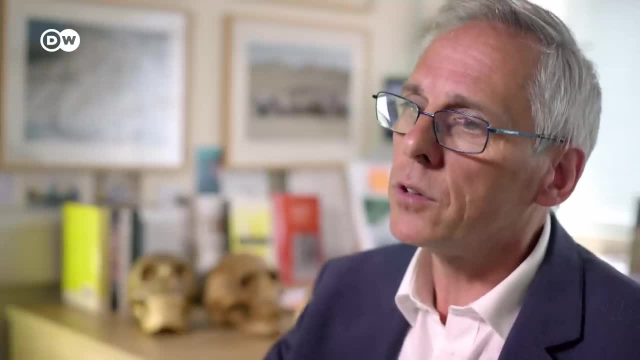 working as a team. I'm going to be absolutely confident that you're going to throw your spear just at the right time to hit that bison, because if you don't, I'll get trampled to death. So how are we going to build up that trust if we haven't got words? I think we 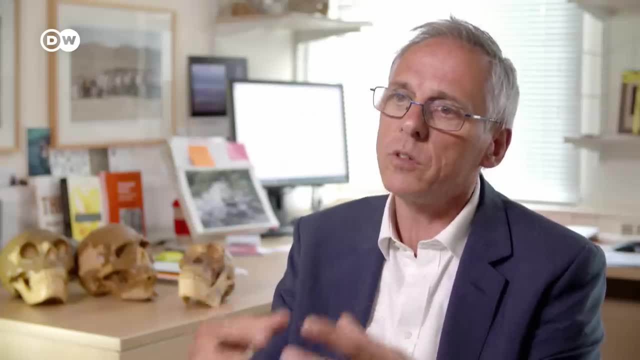 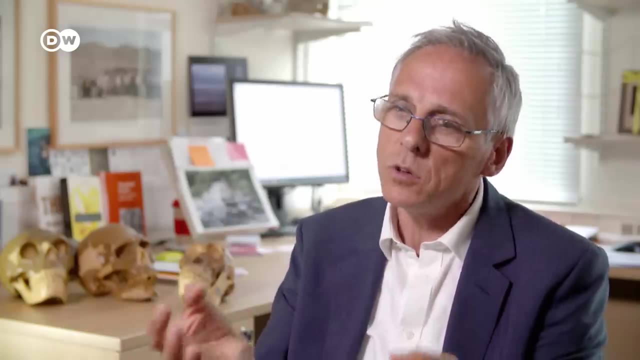 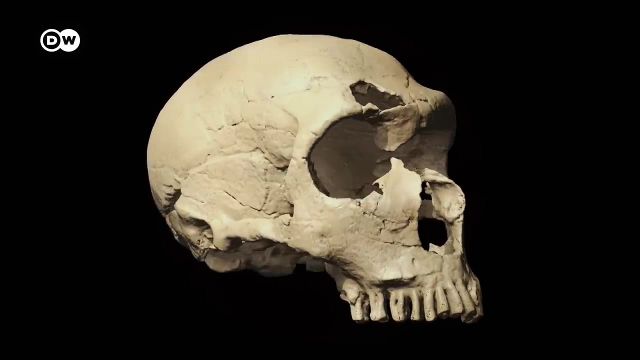 sing and dance together, and I think we still see that in the modern world. Singing and dancing together builds up trust, builds up that common bond, that sense of a group That must be critical to Neanderthal survival. Scientific analysis of Neanderthal brain cases and comparisons with those of modern humans. 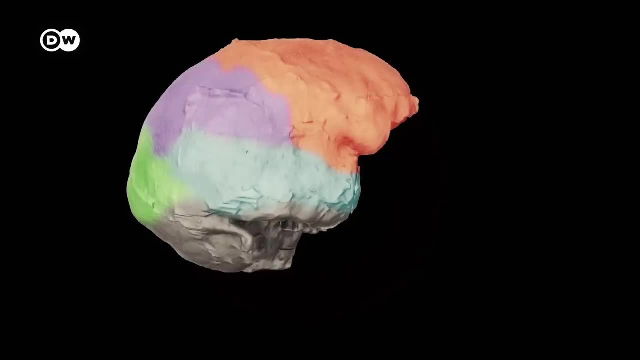 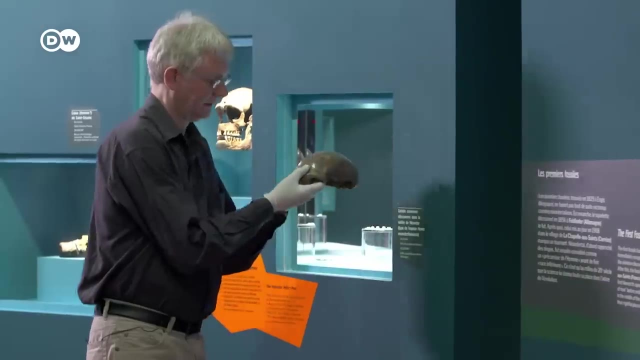 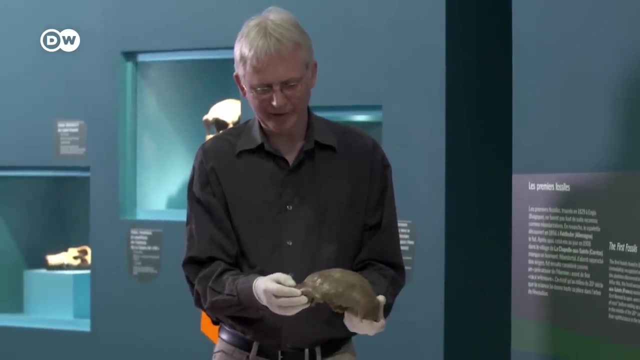 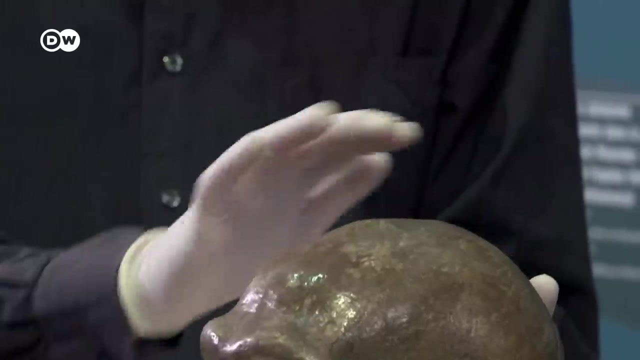 may help scientists to better understand the speech capability of these prehistoric people. The brain case of Neanderthals is very different from that of anatomically modern humans, For example, a flat forehead and strong brow ridges, an elongated, flat skull. This is a robust 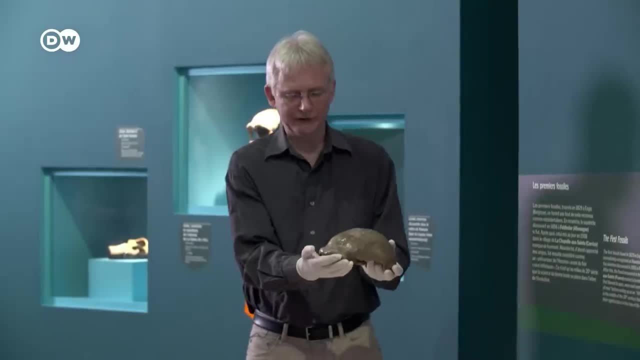 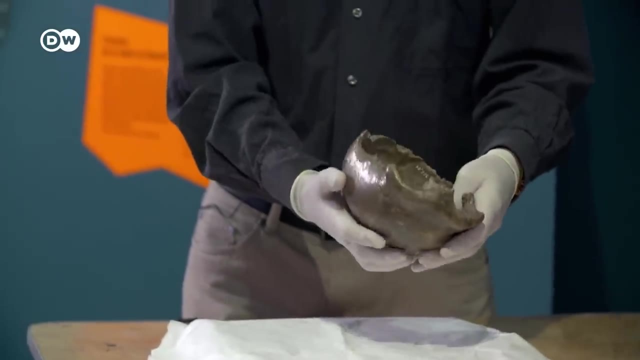 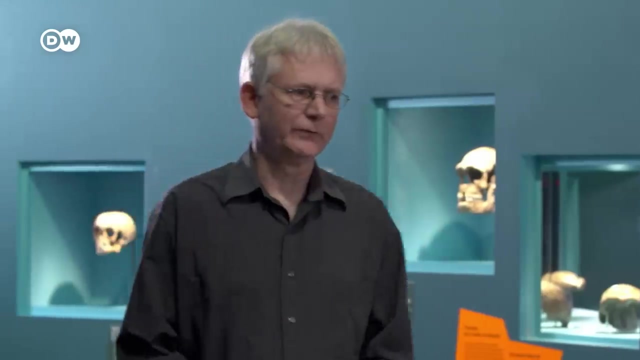 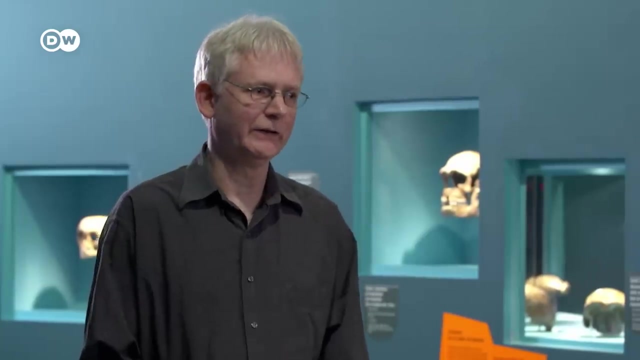 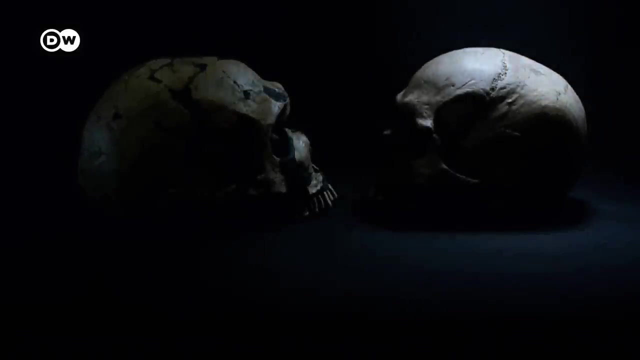 male. He died at an age of 42 years. The shape of the brain is very typical and is unique under the fossils of the world. The morphological structure of Neanderthal brain cases is strongly different from that of anatomically modern humans, but the internal structure isn't well known yet. 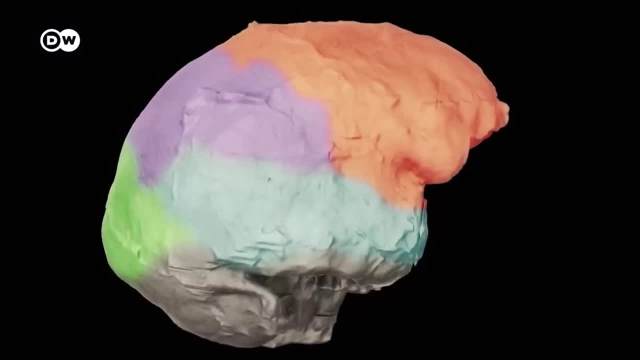 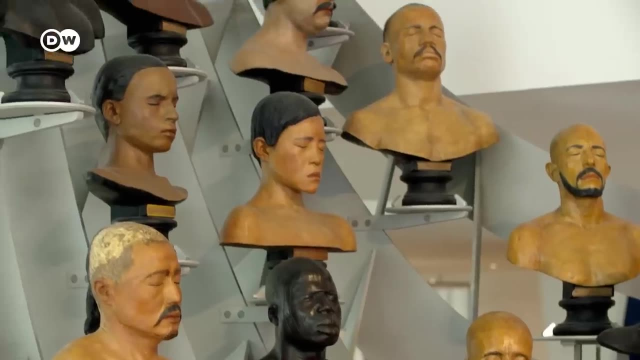 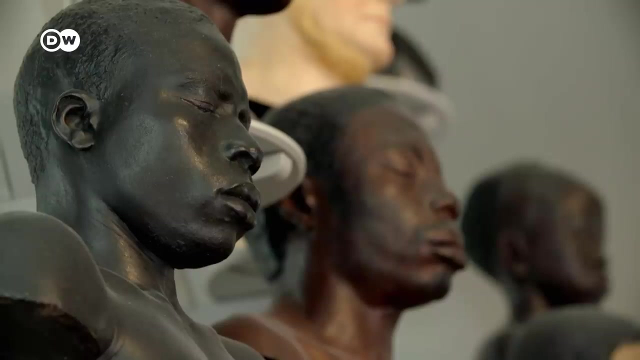 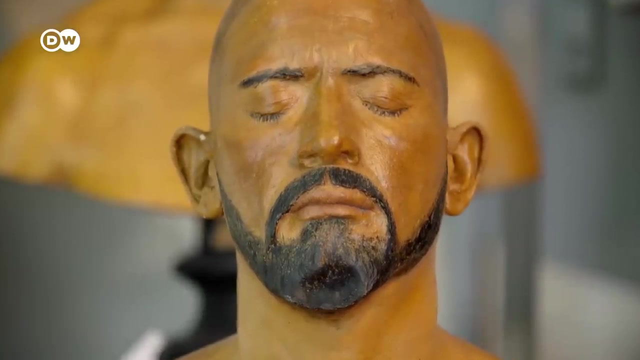 We may never be able to create an anatomical profile of the Neanderthal brain, But scientists can use their knowledge of modern human brain structure to study that of these prehistoric people, especially their cognitive abilities, Because when we talk about cognition- my cognition, it's partly a factor of my brain, and that's 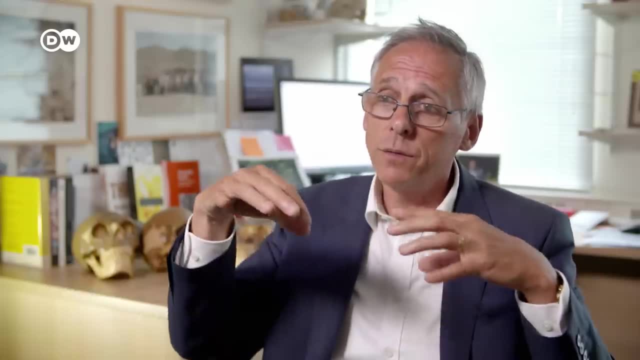 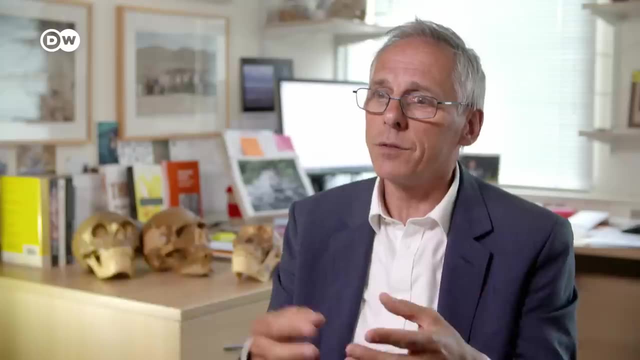 partly a factor of what I've biologically inherited and partly a factor of my development environment. the other support around me. You know I'm not very clever unless I've got a smartphone in my hand these days, or a ruler or a book and so forth. 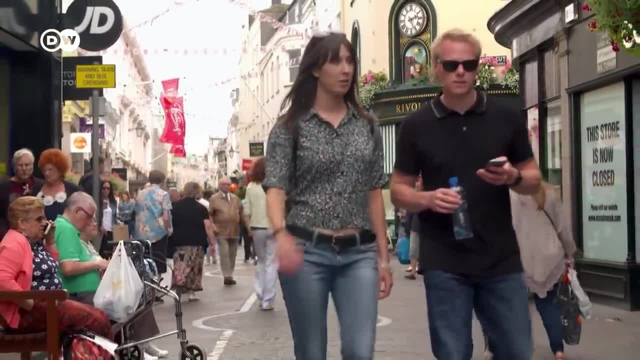 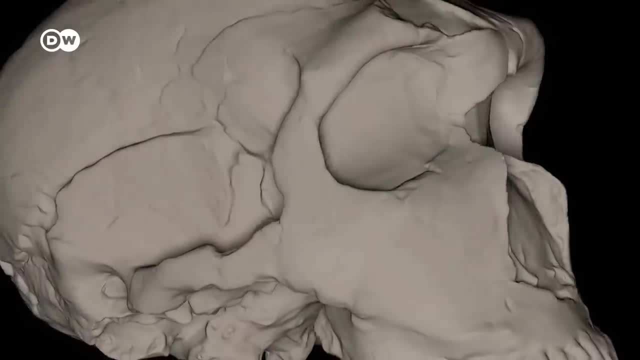 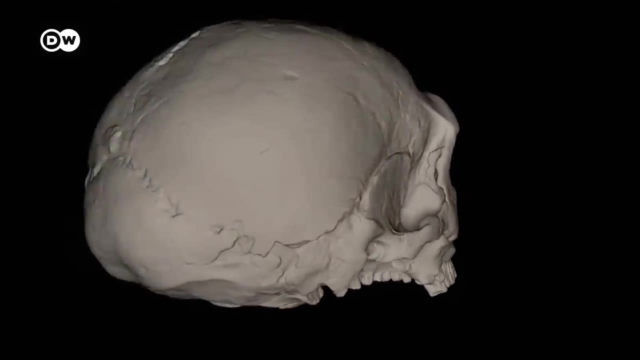 So cognition is really a combination of your material culture. you have your social environment and your biology inside of you. So we know the Nantans had the large brains. They may have become networked differently, But without that material culture to scaffold their cognitive development. 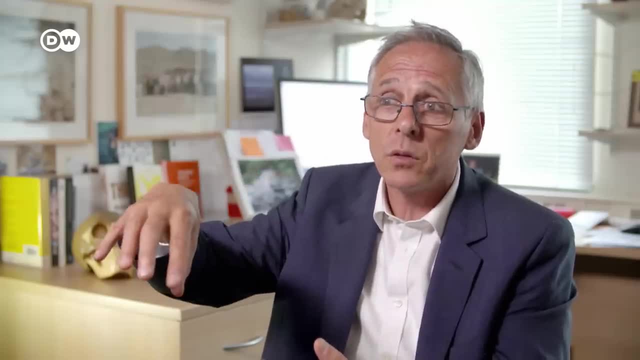 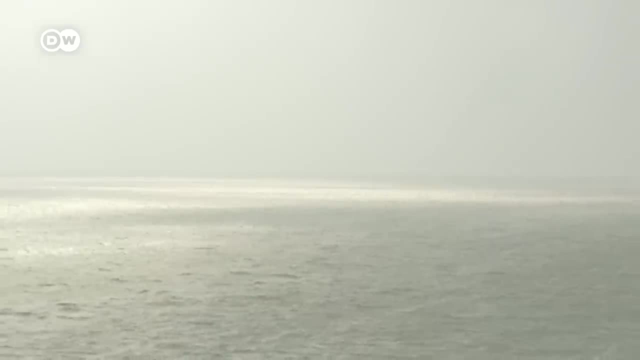 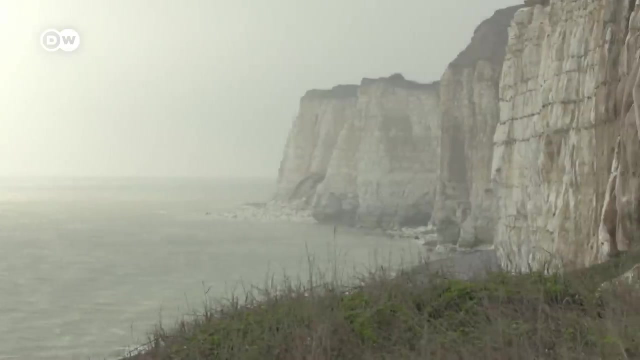 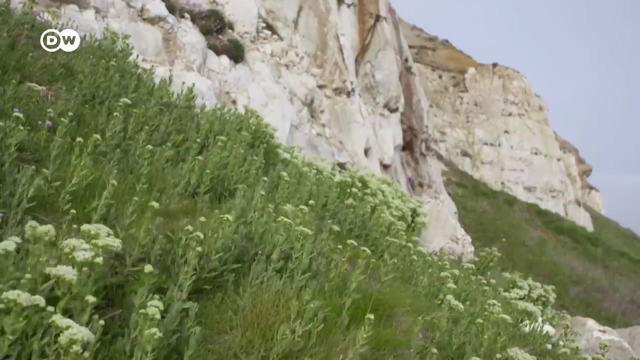 and scaffold and support their thinking, and without words to do that, I think they were inherently inhibited. But despite the limitations cited by Professor Mithun, were the Neanderthals able to develop a culture as we understand the term today? Expert opinion on this topic is divided. 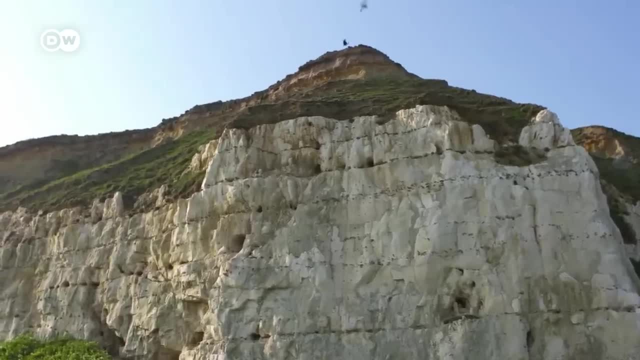 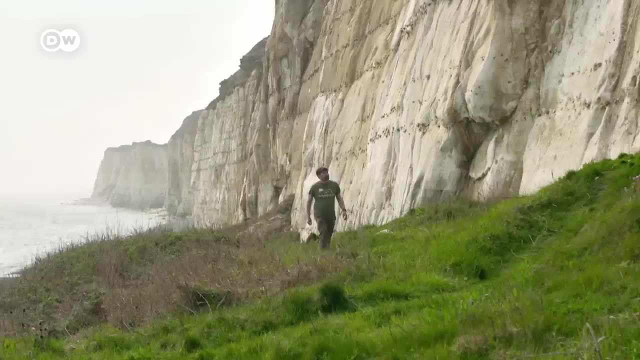 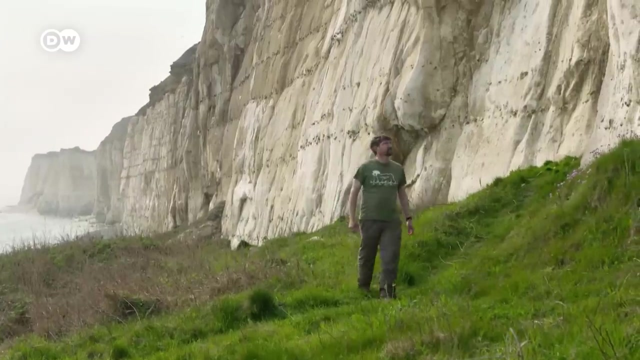 since there's no hard evidence of songs or dances, if indeed they had any. Some scientists believe that the archaeological evidence indicates that Neanderthals were capable of creating works that may be described as art. One of those scientists is British prehistorian Matt Pope. 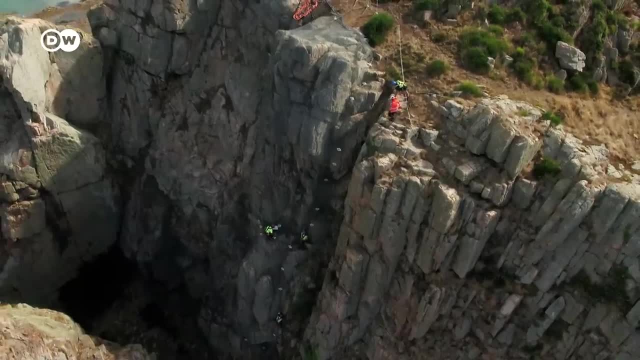 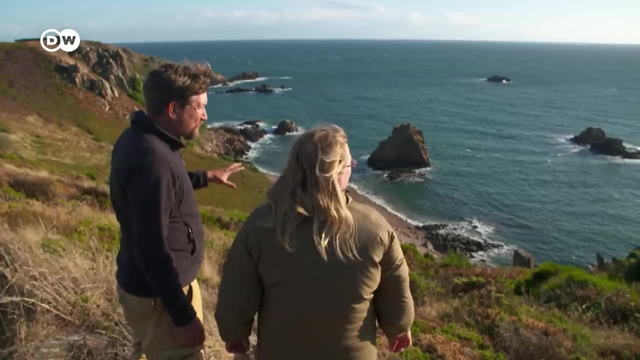 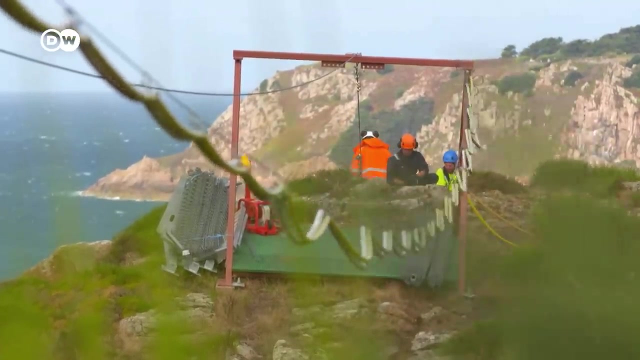 who knows the flint deposits on the south coast of England quite well. Pope is part of the team that's studying the site at La Cote de Saint-Brelade. He and colleague Becky Scott will carry out further excavations there Within La Cote- perhaps the two most famous stratigraphic levels. 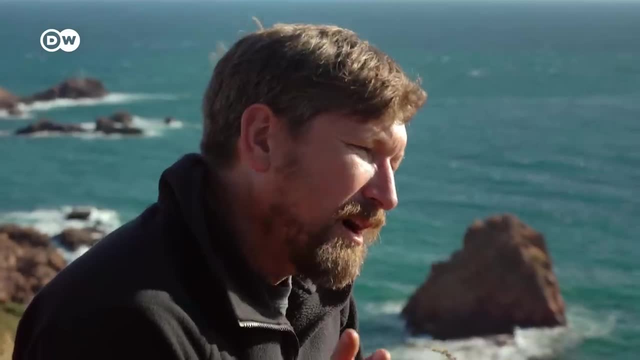 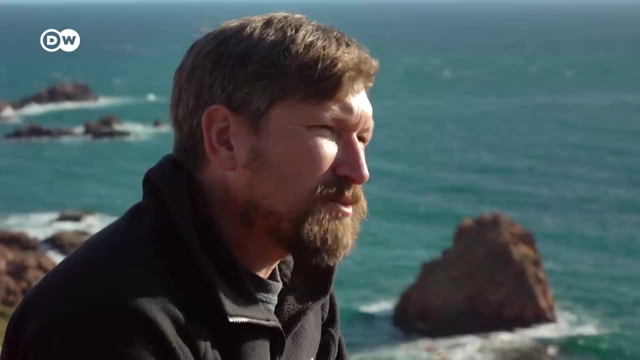 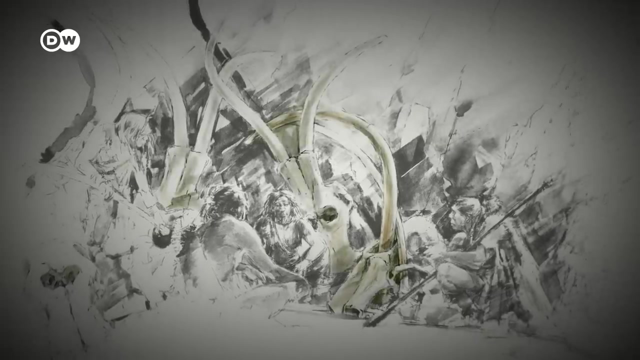 within it are the two bone heaps On the western wall of the cave. they were piling large amounts of mammoth and a small amount of woolly rhinoceros bone. They could be just the remains of butchered animals. neatly, neatly piled up in just a very ordered behavior. 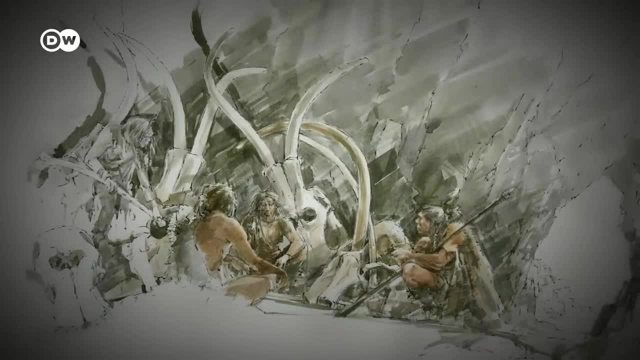 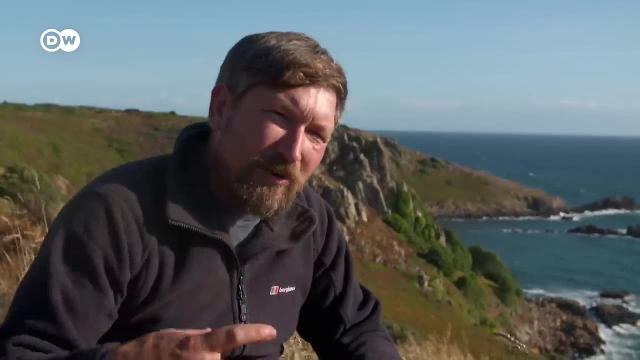 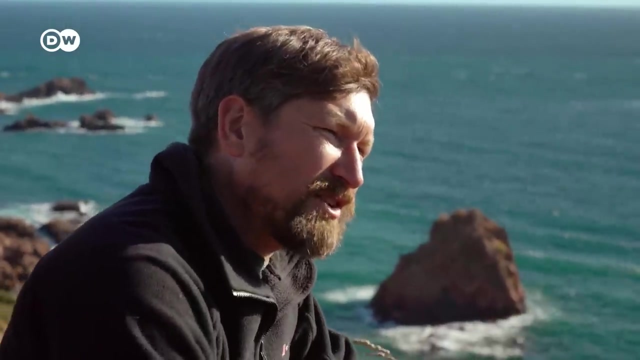 They could be stockpiling them for other uses. These bone heaps go even further in their ordering. The way the skulls of mammoth are placed around the outside of these bone heaps, the way that ribs are driven on end into the sediment, almost to fence in and constrain. 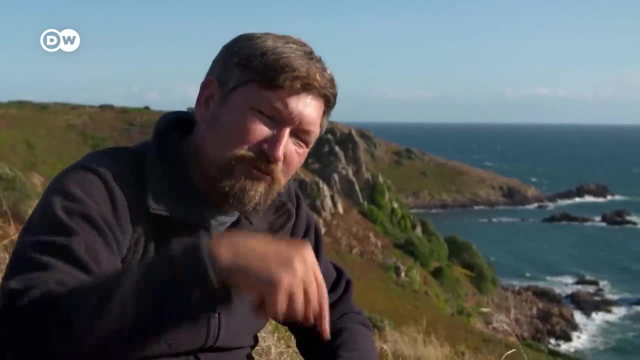 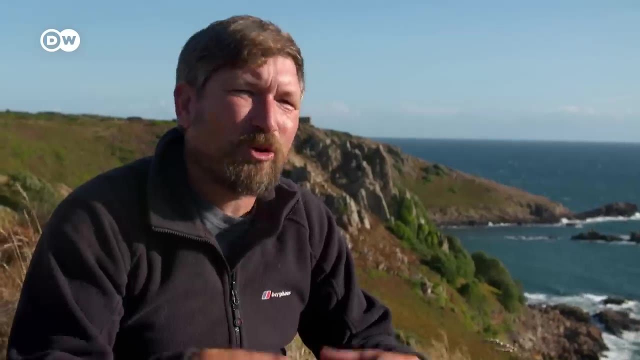 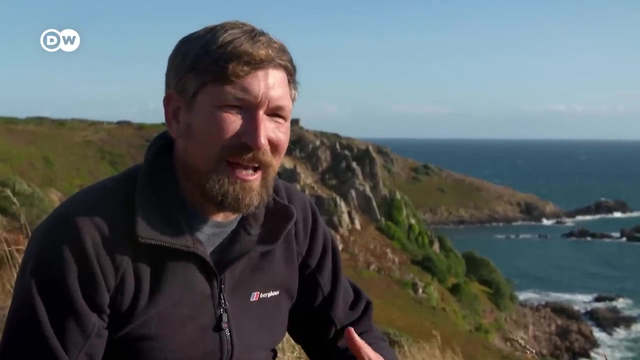 the bone heaps and in one case a rib even driven through a skull into the sediment underneath, goes beyond simple tidiness, goes beyond stockpiling material. They're creating something, Even if it's just a kind of routine, habitual behavior. 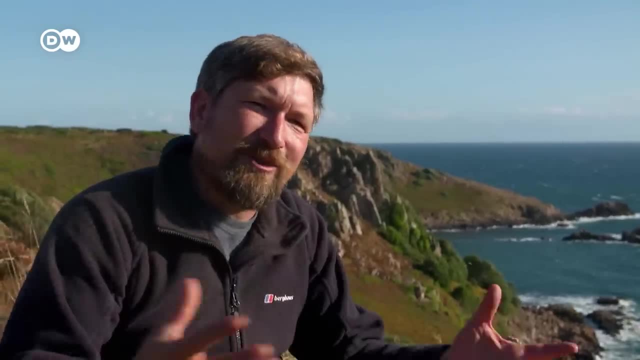 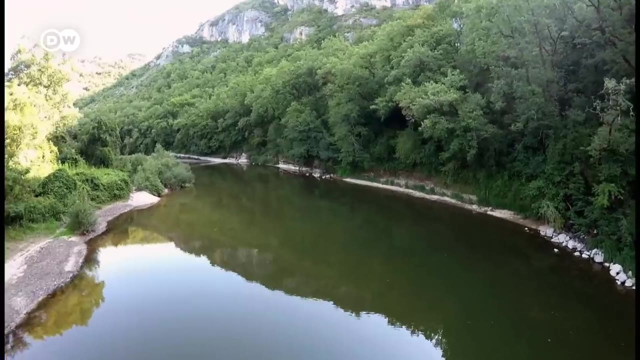 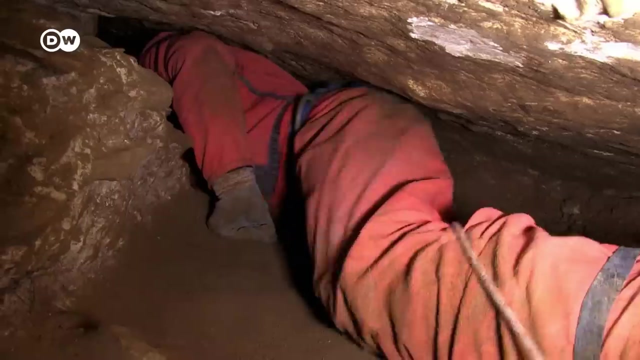 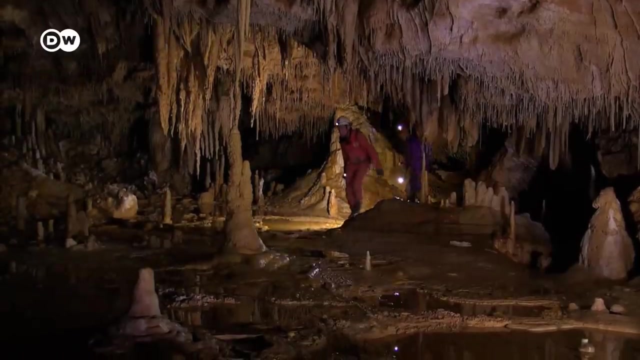 even if it has no symbolic meaning, it's still monumental what they leave behind. It would still, if you saw it today, look very, very striking. Evidence that Neanderthals were capable of planning and building structures is rare. So the discovery of the Bruniquel Cave in 1990. 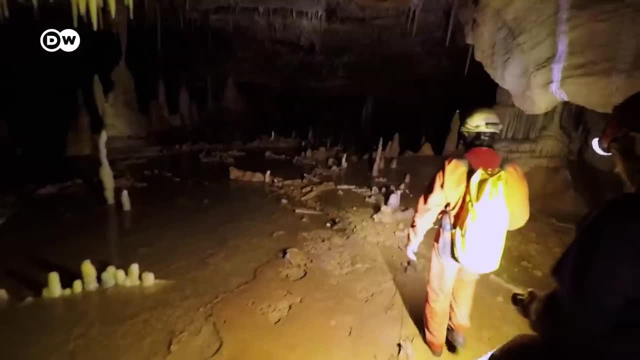 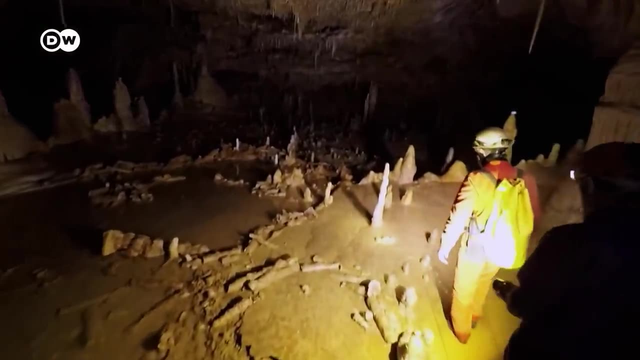 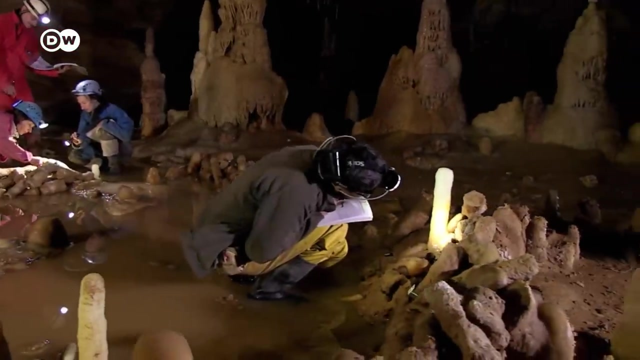 in France's Aveyron Valley caused a sensation. In a space located more than 300 meters from the entrance, archaeologists discovered several structures made of broken stalagmites. There are rings of this material, as well as random piles. The ring structures were later determined. 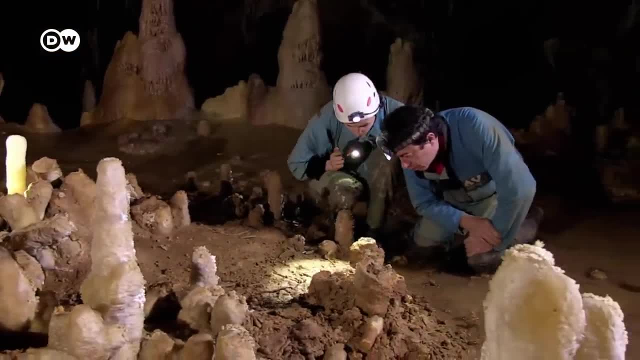 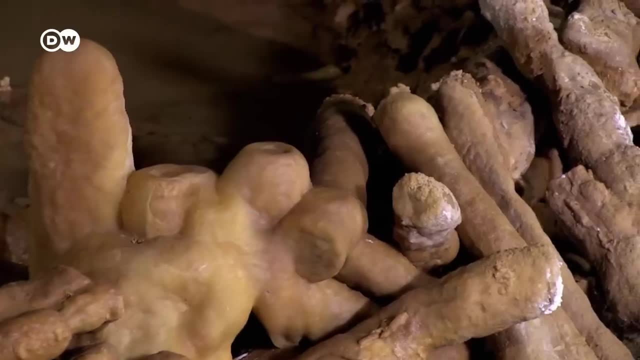 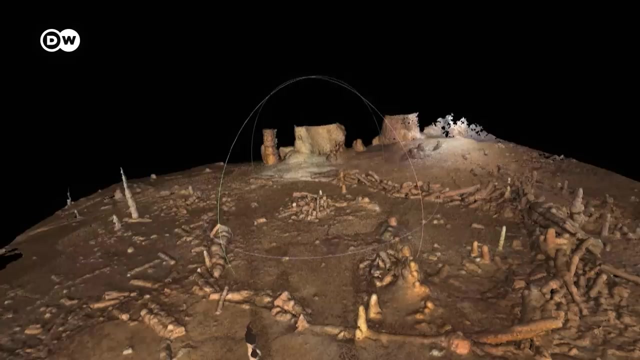 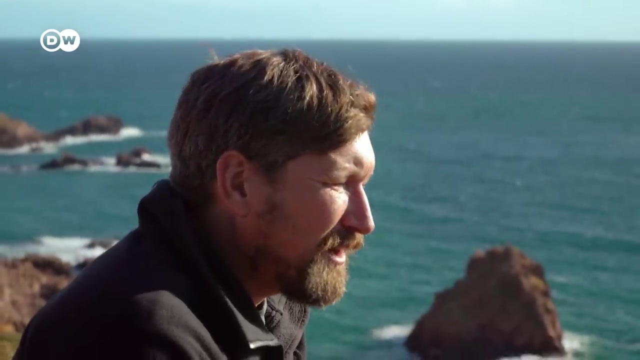 to be approximately 175,000 years old. Some scientists say that the Neanderthals who built these structures had developed a complex level of social organization. There's a parallel between the bone heaps and the stalagmite circles at Bruniquel Cave. 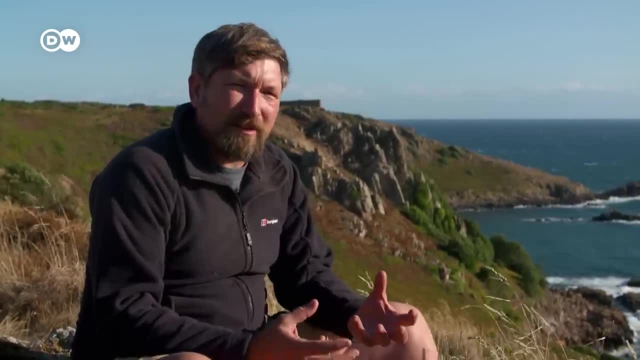 Both, in a way, are inexplicable in their own way. There's a parallel between the bone heaps and the stalagmite circles at Bruniquel Cave. Both are very, very structured. Of course, at Bruniquel it's deep in the cave. 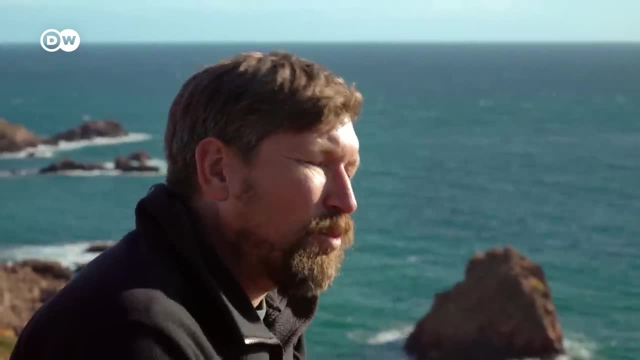 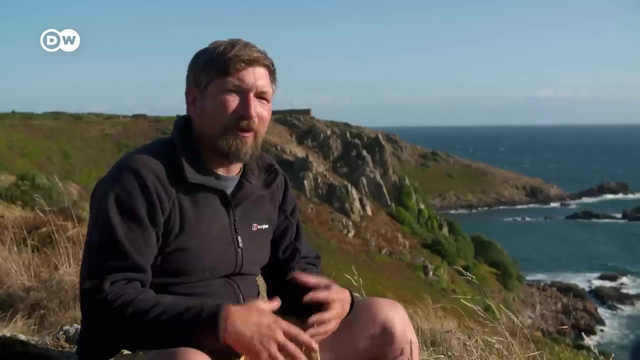 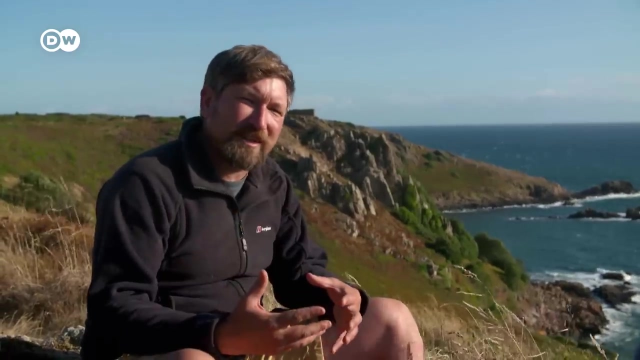 They're not using food refuse, But it shows that they're capable of working together to create structure out of chaos without any obvious function. We've got lots of words for those sort of behaviors in our own language. We can call it symbolism, We can call it art. 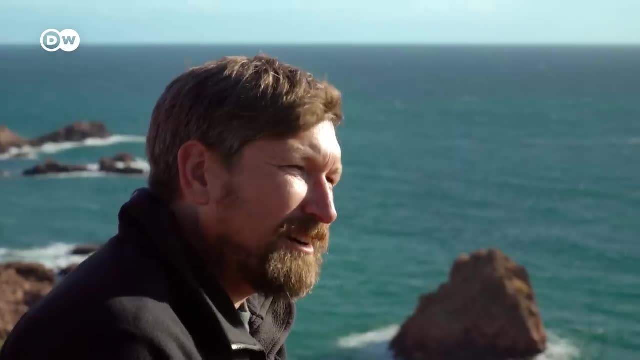 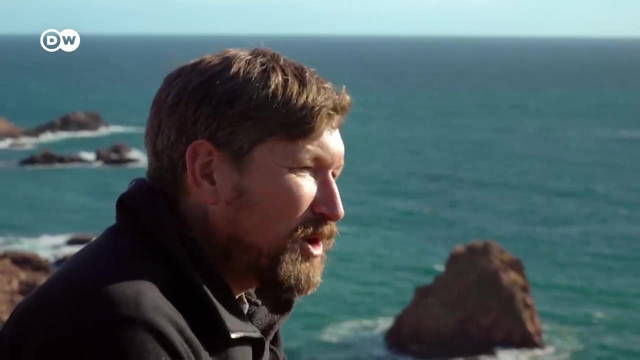 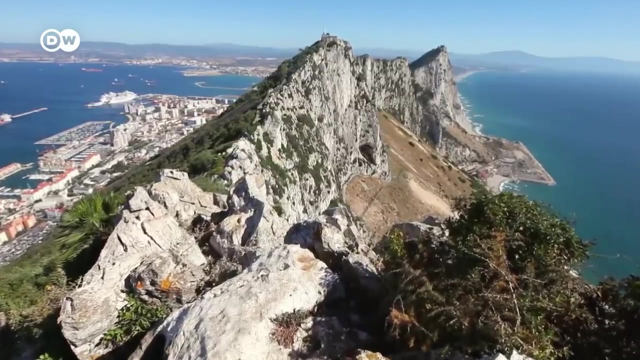 We can call it ritualistic behavior. I don't think those words are very helpful. It's just something very, very human to try and monumentalize landscape. Monumentalize landscape with our own traces and our own interventions on it. A rare indication of Neanderthal abstract expression. 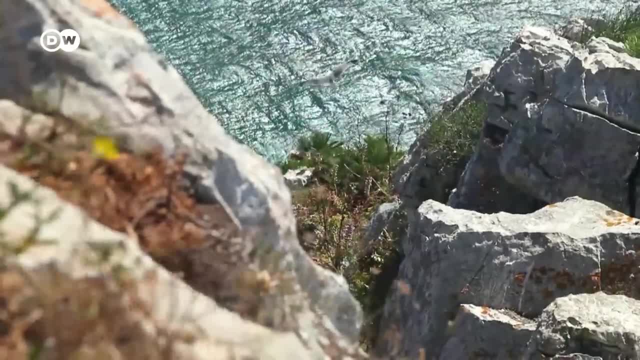 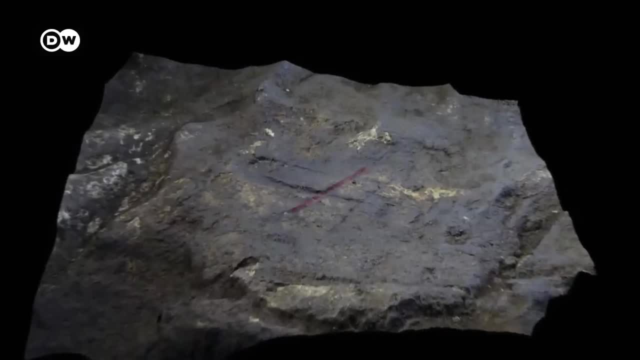 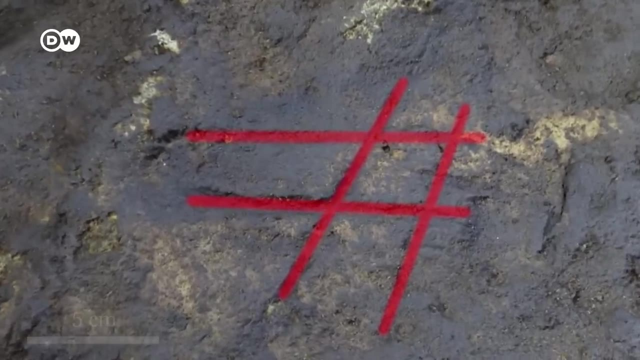 was discovered at Gorham's Cave on the Gibraltar Peninsula in 2014.. A series of intersecting lines. The press dubbed it history's first hashtag. It's not clear what the symbols mean. Some experts like Ludovic Slimac: caution against speculation. 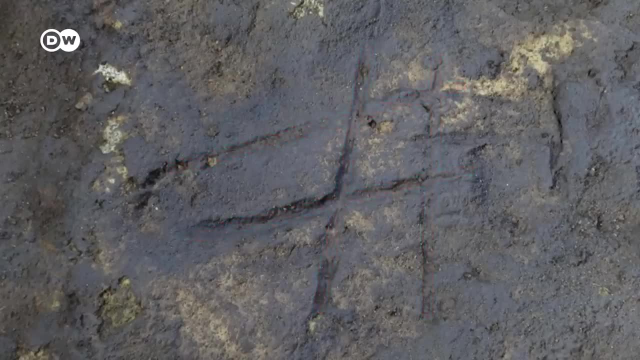 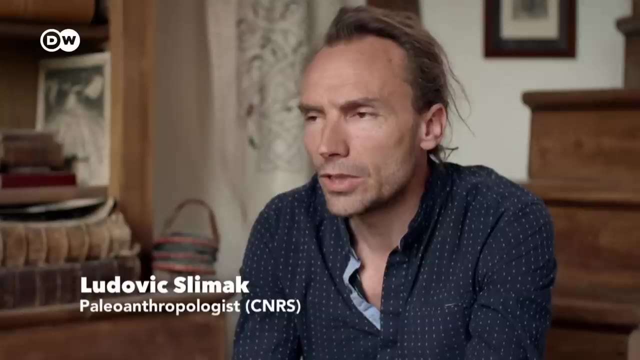 There's evidence that early Homo sapiens made jewelry. They took the teeth of carnivores that they killed, drilled holes in them and created necklaces. We've found none of that among Neanderthals: No jewelry, necklaces, beads or anything that might require drilling. 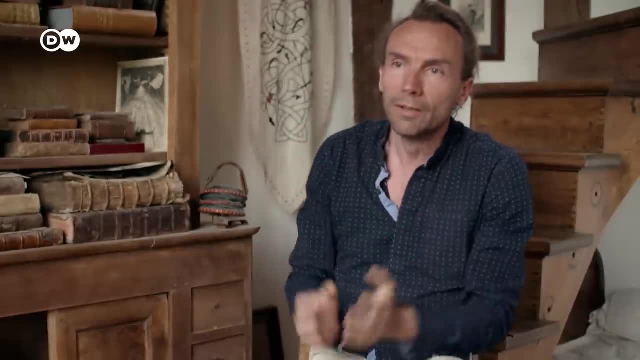 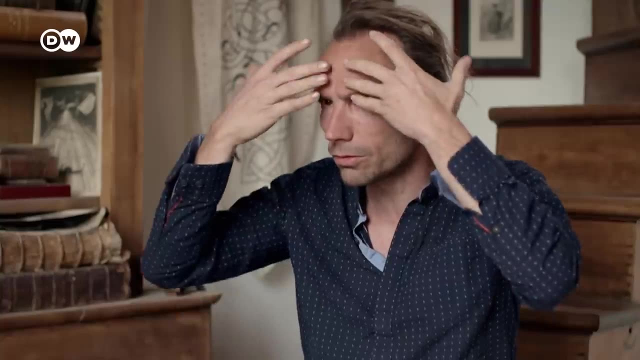 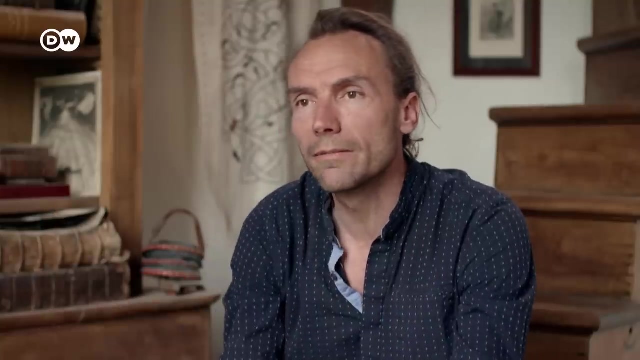 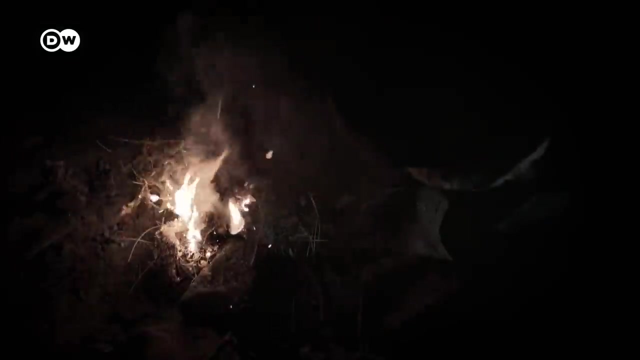 And scientists have examined countless artifacts from that period. Humans wear jewelry and clothing to show off. These items shape our mental, cultural and social universe, which we then present to others. Neanderthals simply didn't do that. Future archaeological discoveries may prompt skeptics to change their minds. 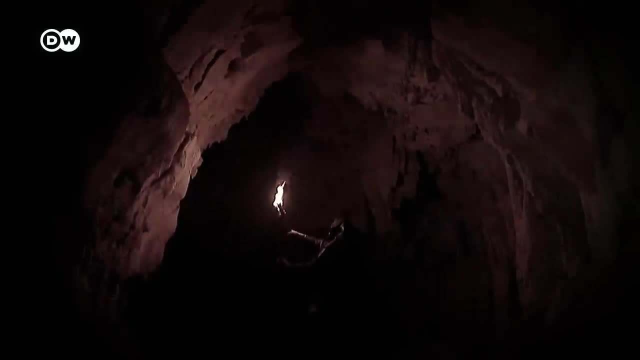 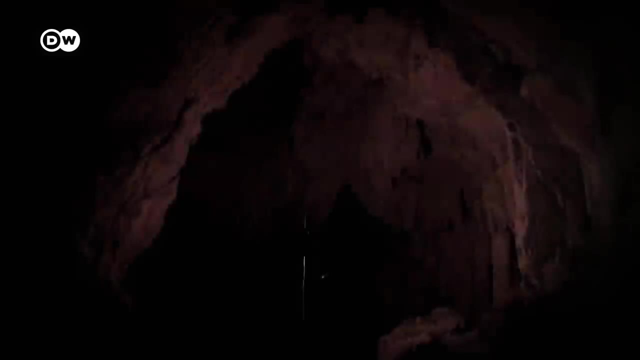 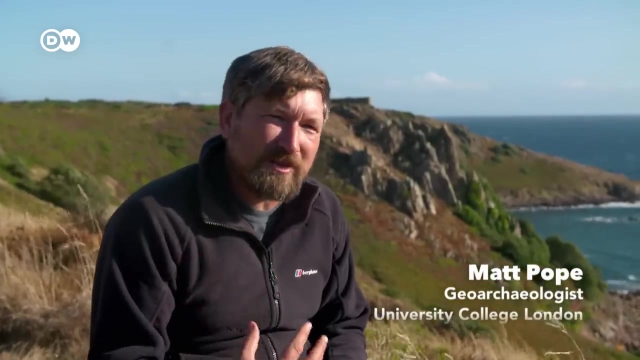 But this discussion also raises an important question: How closely did Neanderthals resemble modern people? The science constantly changes how we envisage Neanderthals And at the same time, we want to bring them close to us. We're seeing them as very modern in terms of their behavior. 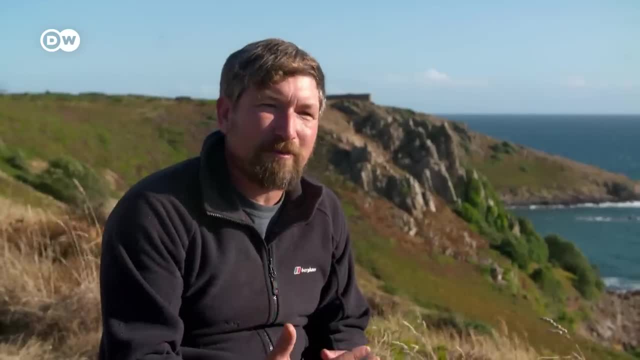 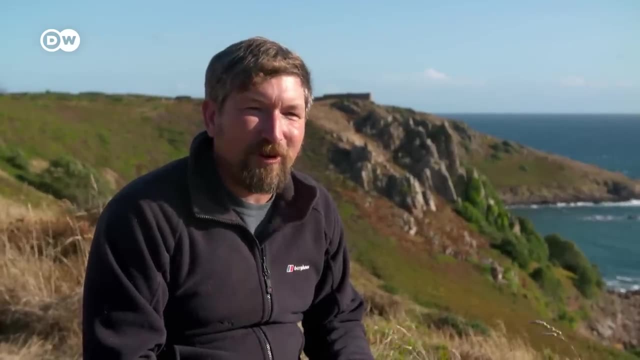 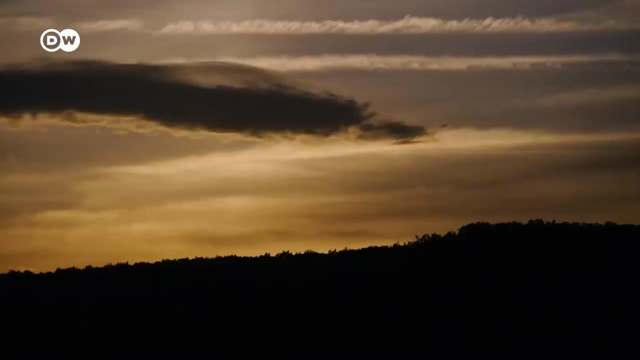 We should never forget the fact that if we were confronted by one, if we encountered one in the street or in the landscape, we'd instantly notice differences in their morphology, in their face, in their bearing, in their gait. The first humans of the species Homo sapiens arrived in Western Europe. 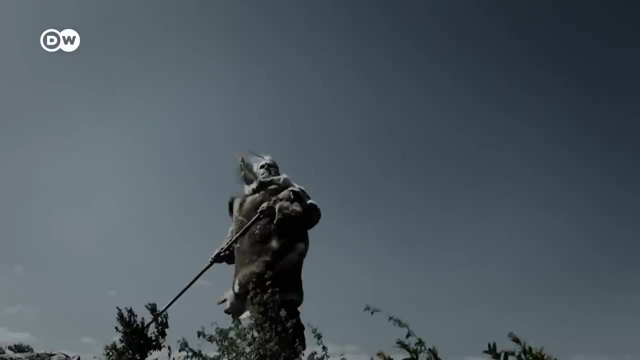 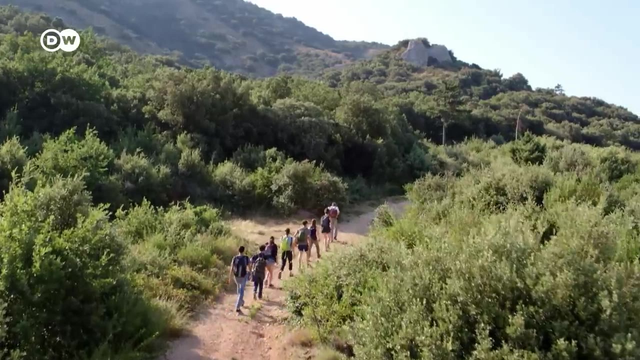 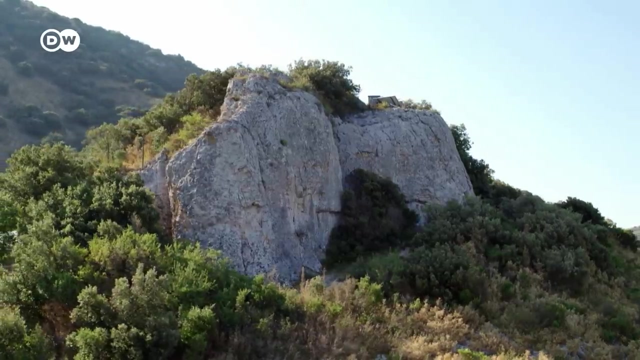 about 50,000 years ago. This development appeared to seal the fate of the Neanderthals, who were far less sophisticated. Studies of the Mondrang Cave, the reconstruction of settlements there and the discovery of flint objects indicate that Homo sapiens 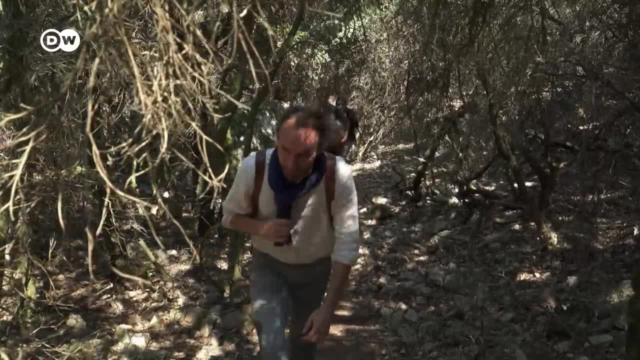 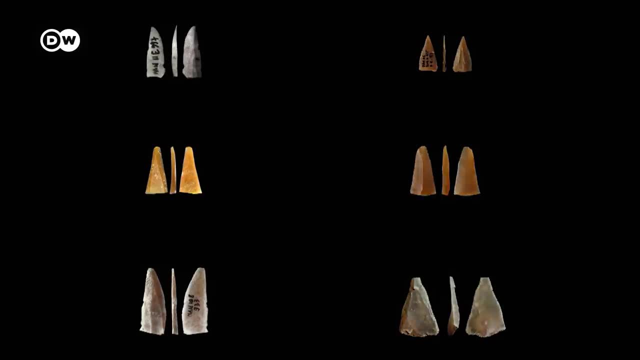 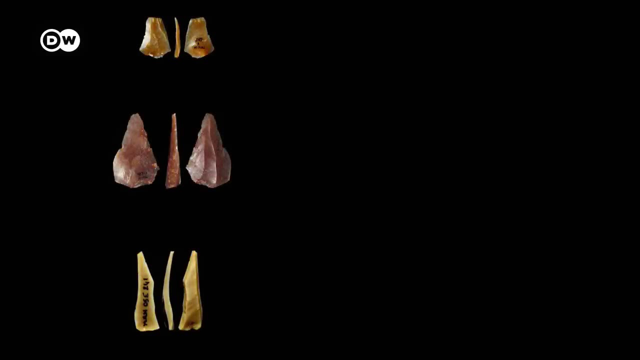 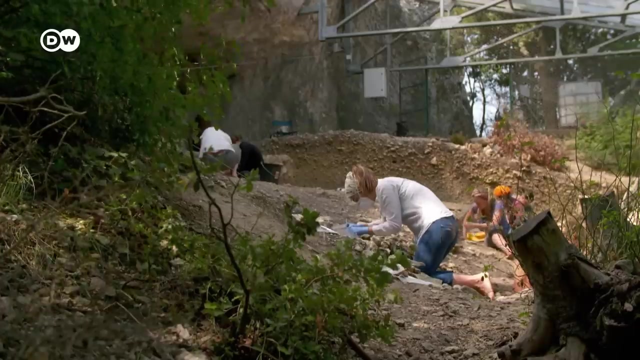 came to Western Europe in two waves. The first consisted of scouting parties who used advanced flint tools. That group disappeared after about 10 years and the Neanderthals gradually returned to the Mondrang site. Homo sapiens returned to the region a few thousand years later. 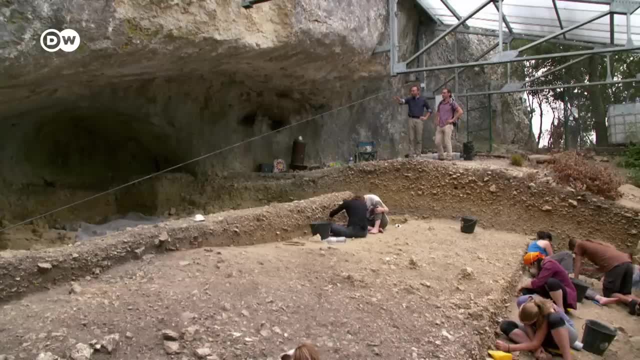 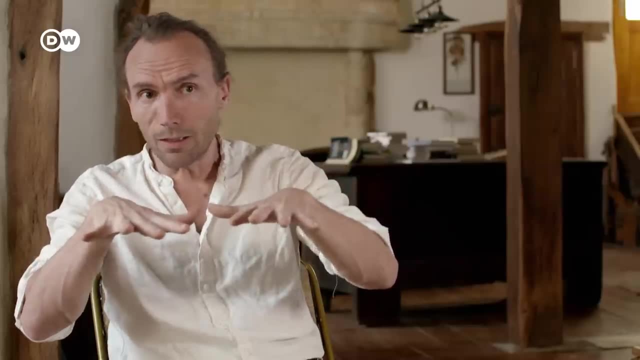 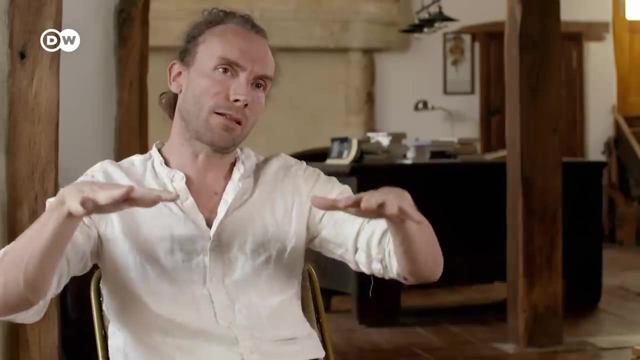 around 42,000 years ago. This cave was home to both the last Neanderthals and the first modern humans. They probably traveled north from the Mediterranean through the Rhône River valley. They settled there and it's likely that they came into contact with Neanderthals. 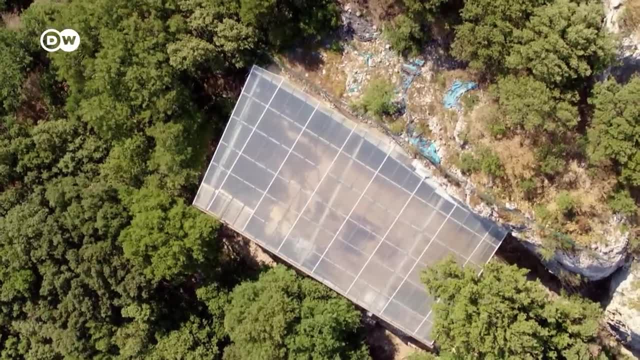 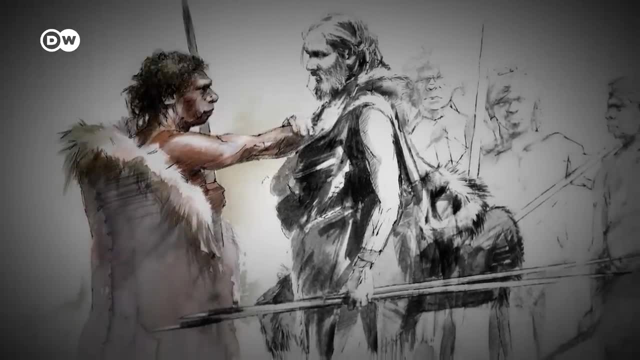 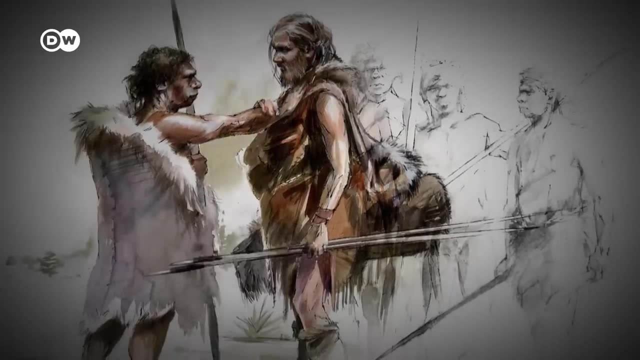 This was just about the time that the previous residents of this region, the Neanderthals, started to die out. There's been a lot of speculation about why and how this happened. The Neanderthals had been there for dozens, even hundreds, of generations. But suddenly, with the arrival of Homo sapiens, they disappeared. They never returned to the caves where they had lived. Studies at sites in France, other parts of Europe and Western Asia have concluded that the Neanderthal population became extinct about 42,000 years ago. 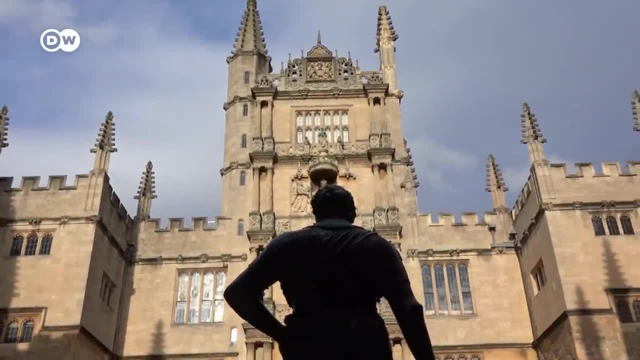 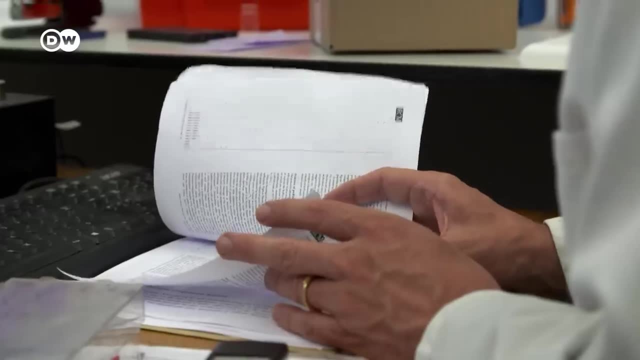 Tom Haim is an expert on carbon-14 dating. He's a professor of archaeological science at Oxford University and says that recent scientific studies have provided new information on why the Neanderthals died out. And actually this is different to what I originally thought. 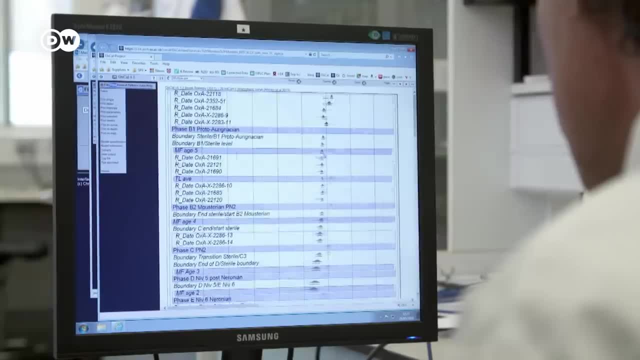 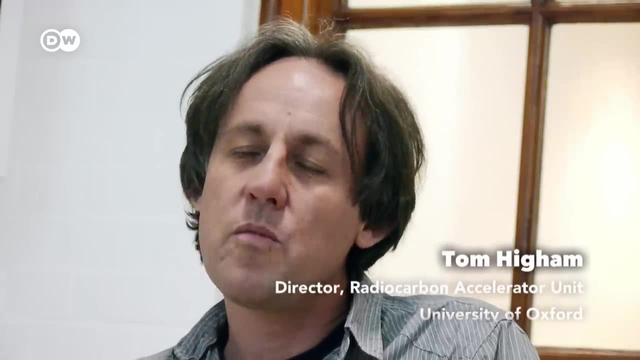 when I first started working in this area I thought that modern humans would kind of sweep in and Neanderthals would go extinct relatively soon after. But actually it seems to be a lot more complicated than that And there seems to be a mosaic of populations in different parts of Europe. 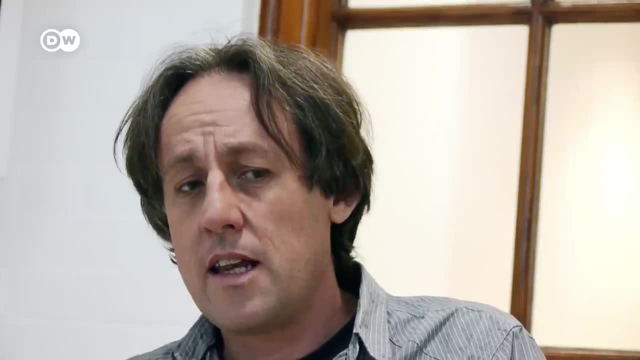 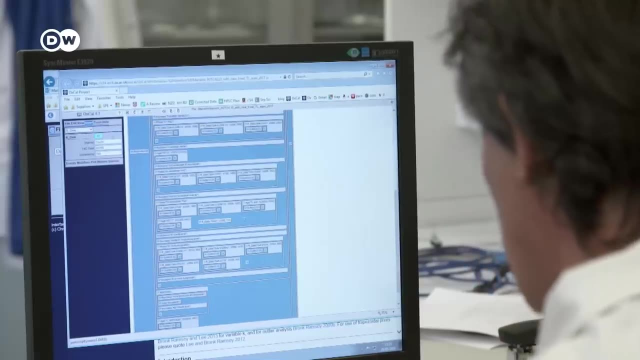 We also know, of course, that the DNA is telling us that these two populations not only met, but they interbred with one another, which adds an increased layer of interest and complexity at the same time, I think, over the 2,000 to 4,000 years in which we see modern humans. 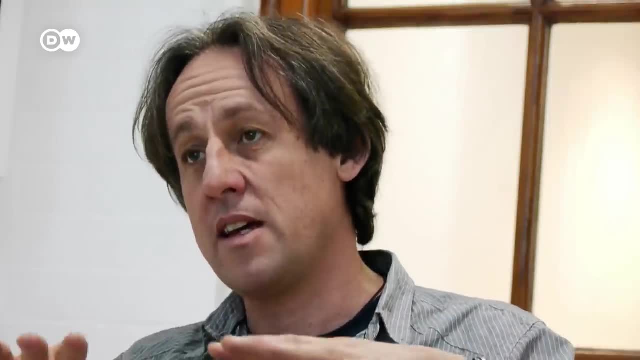 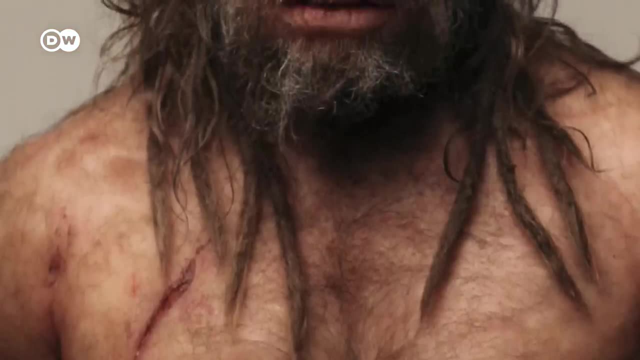 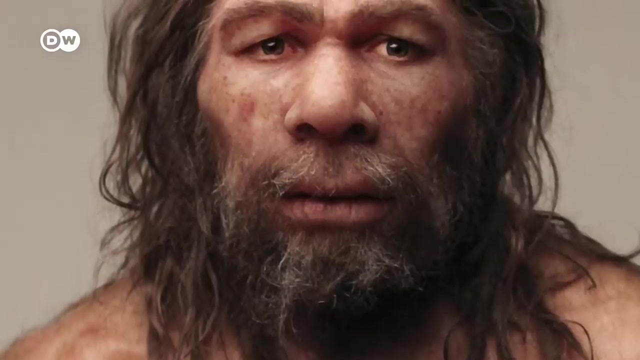 and Neanderthals living or overlapping in Europe that there was a slow and gradual disappearance of Neanderthal groups. As Neanderthals started to interbreed with Homo sapiens, their numbers grew smaller and smaller until they eventually disappeared altogether. 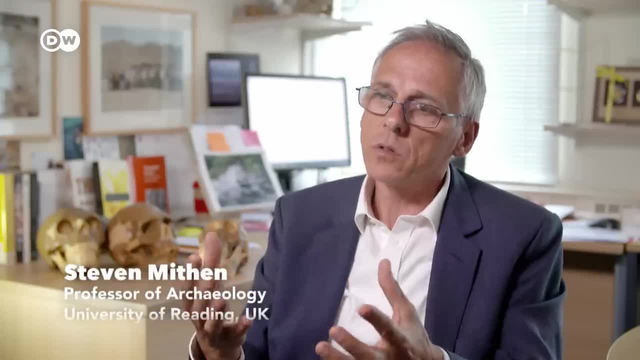 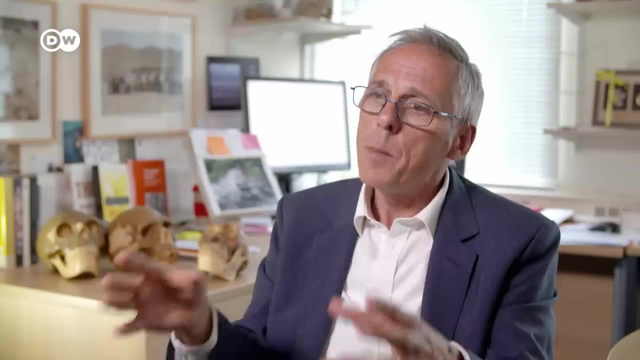 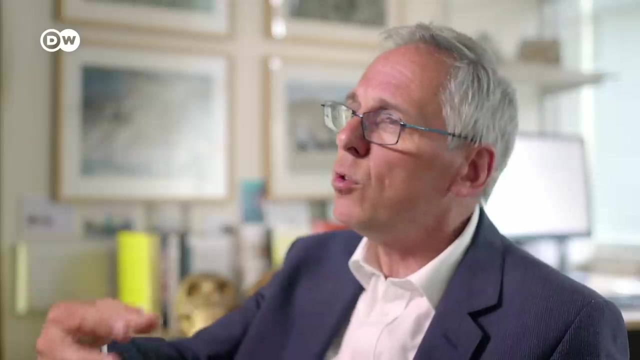 I think the Neanderthals were to some extent trapped in their success. They survived for 200,000, 300,000 years through huge amounts of climate change in very challenging environments, But their culture remained pretty stable For 200,000, 300,000 years. they were making basically the same types of tools. 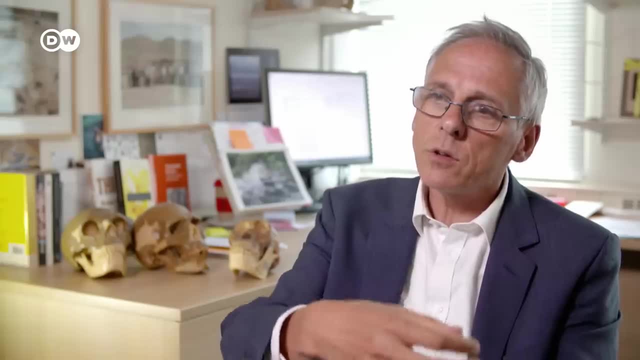 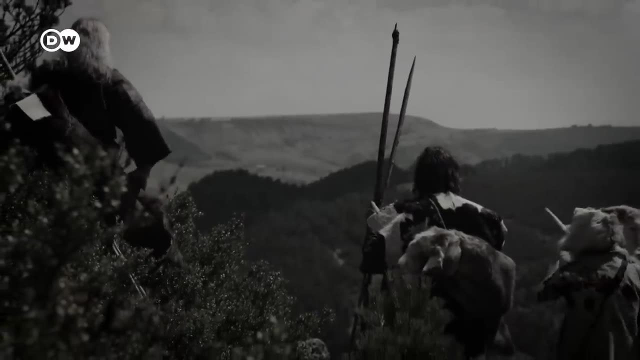 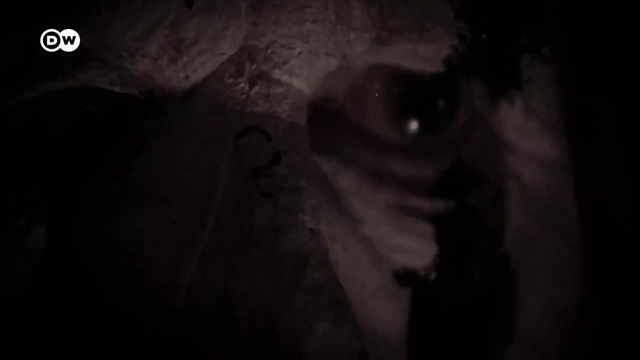 They were exquisite tools, But the amount of innovation, the amount of creativity is minimal. Neanderthals and Homo sapiens coexisted across Eurasia for several thousand years. These ancient humans managed to survive major changes in climate, but they failed to adapt to the arrival of a superior species. 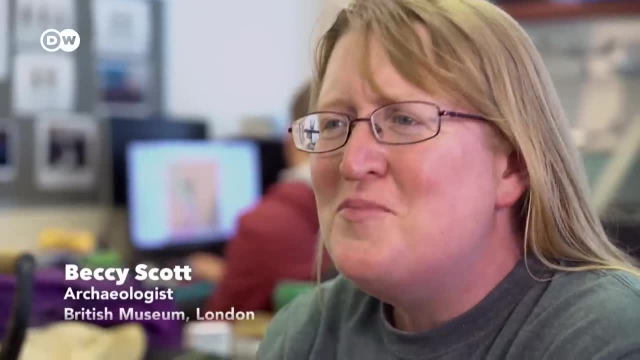 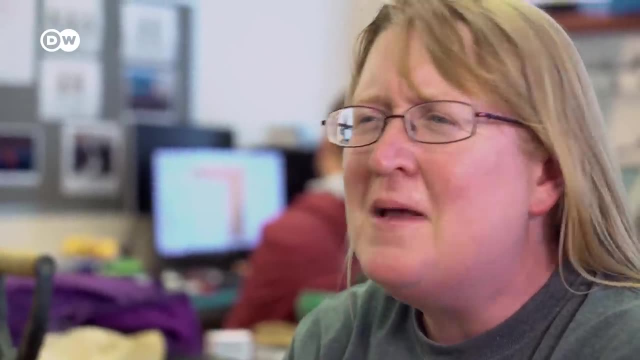 The thought that there was a point where there was a group of people you know surviving in the same landscape who were, you know, superficially so similar to us but maybe did things in a different way. it's almost like playing a hunter-gatherer thought experiment, or something. 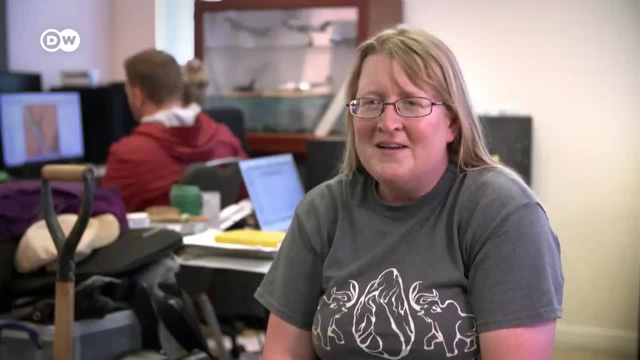 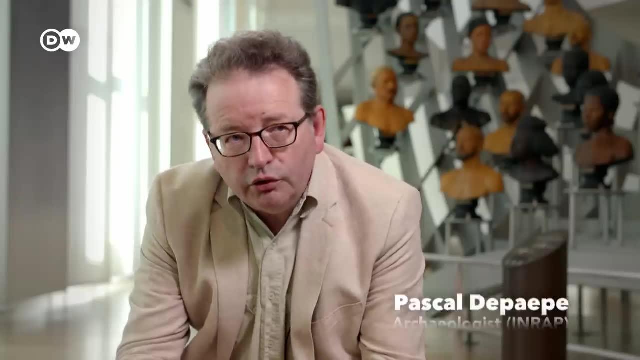 I just think it's incredible that at one point, we weren't the only human species that walked the Earth as we are today. I think that the way that we look at Neanderthals says a lot about how we deal with others. 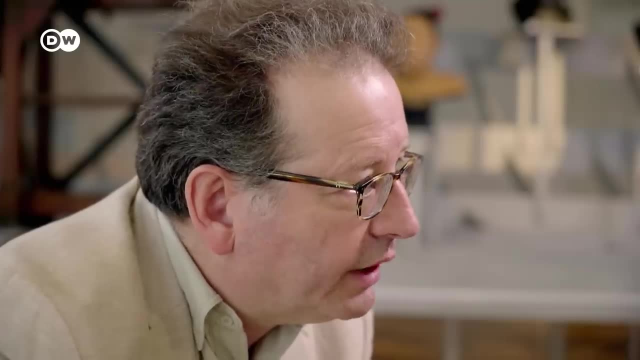 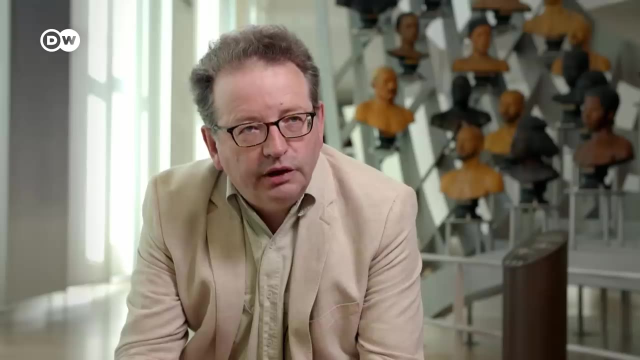 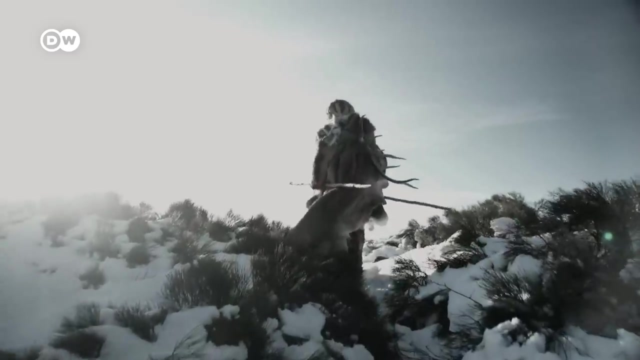 And this raises the question of how we treat other members of our species. Today, people are always talking about the cultural shock of migration. I think the situation is exaggerated, but it still reflects on how we deal with others. From time to time, archaeologists find new evidence. 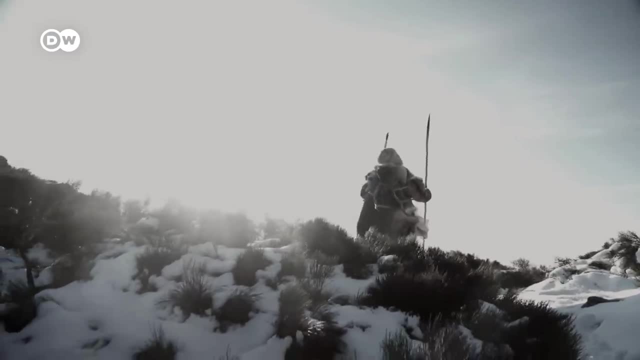 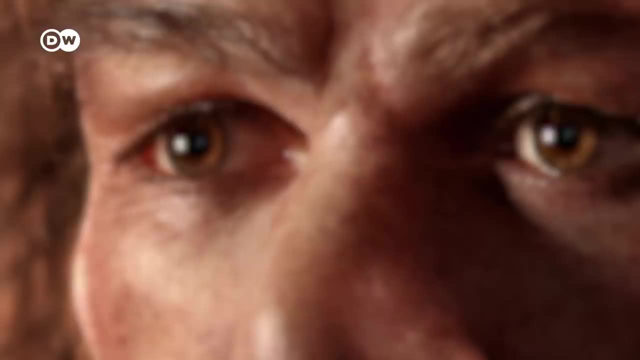 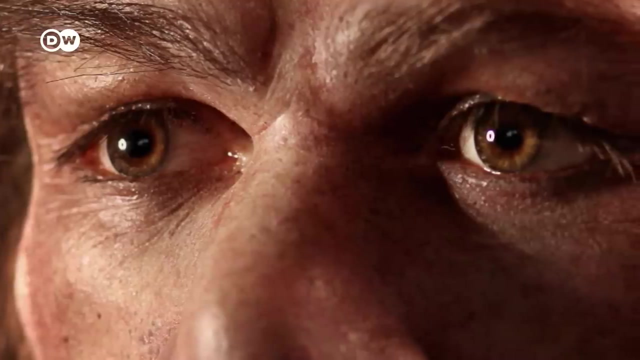 that helps us to better understand how Neanderthals lived, But these are just fragments from the long history of this species. Modern humans inherited part of their genetic code from Neanderthals. Perhaps that's why many of us are fascinated with the relics of these ancient people. 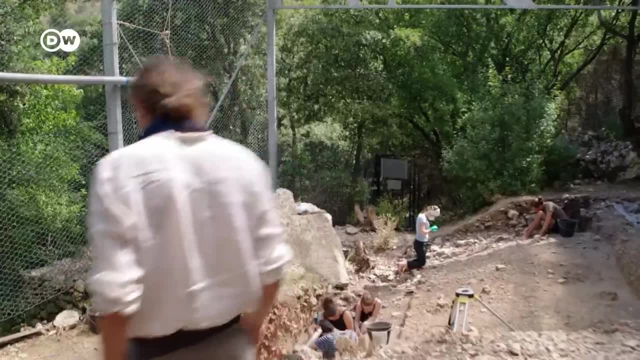 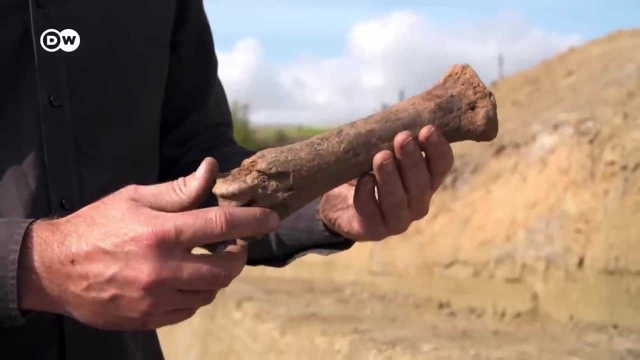 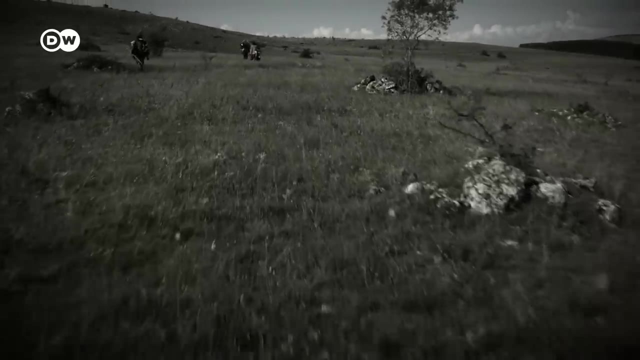 and the similarities that Neanderthals share with modern humans. If they had managed to survive, the world would likely be a very different place. Neanderthals developed a distinct social intelligence and were much more attuned to the world. They were more interested in their environment than was the species that replaced them. 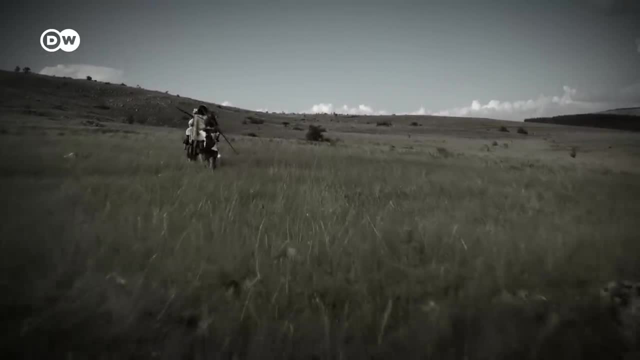 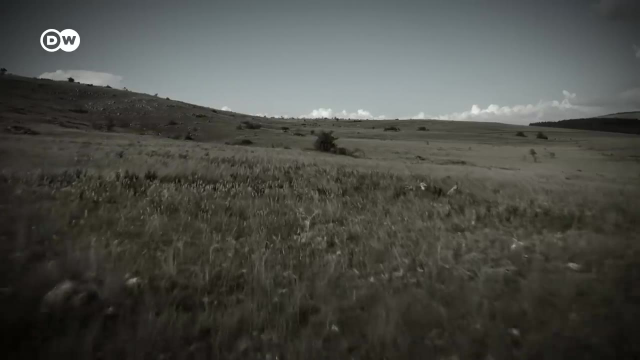 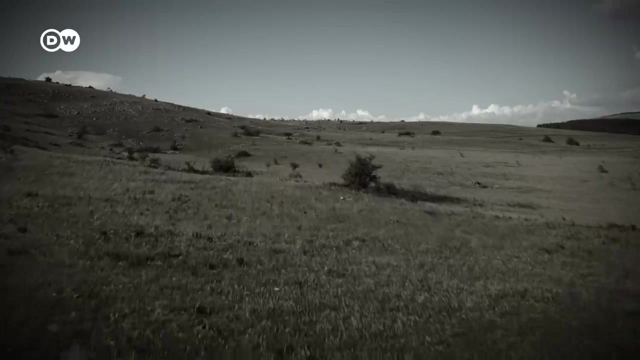 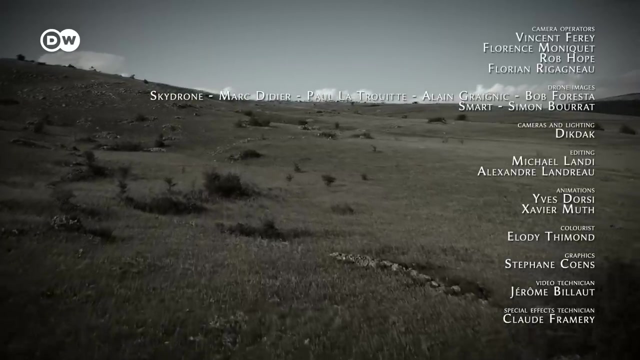 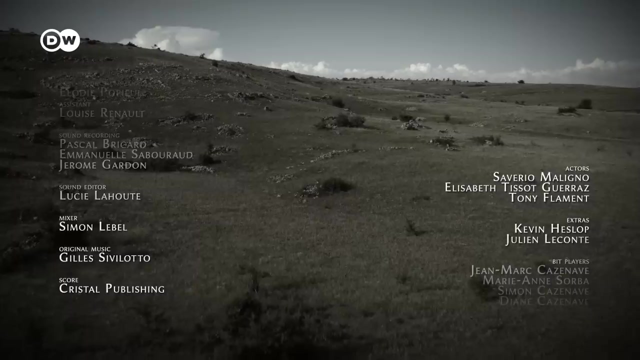 We can only speculate on what influence the Neanderthals might have had on the course of human history, for better or for worse. This is a story about the ancient Neanderthal species. National documents on the Neanderthals. They don't get a lot of evolution. 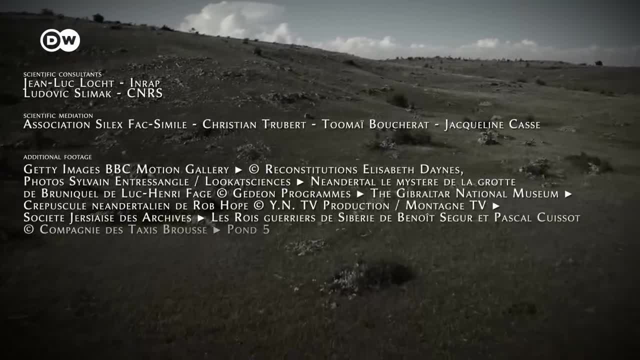 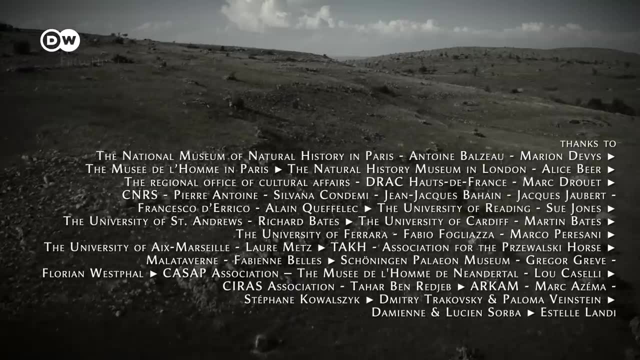 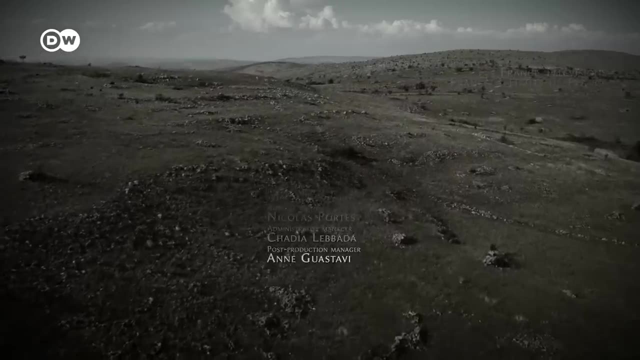 They don't even know how long a human was. We need to get to the point when we get to the point where they say we know This is a story that has been telling for centuries. There are many engineers in the world who have been trying to figure out. 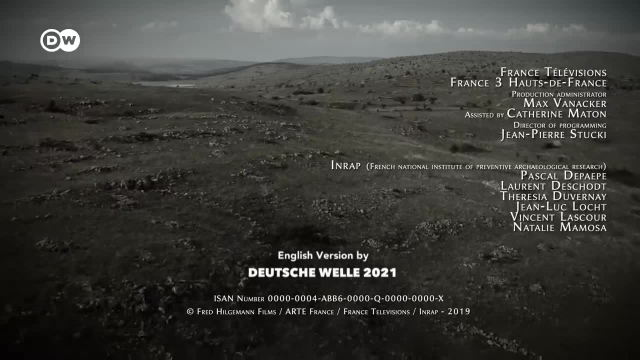 how Neanderthals lived. Thanks for watching. 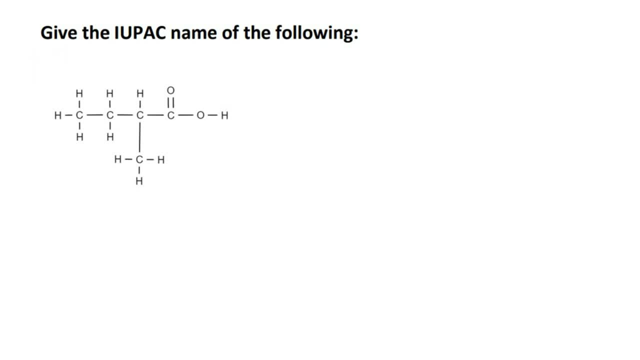 So here we need to come up with the IUPAC name. So the first step is just to make sure we see the longest carbon chains. That would be one, two, three, four. Okay. so four means butte, Okay now. 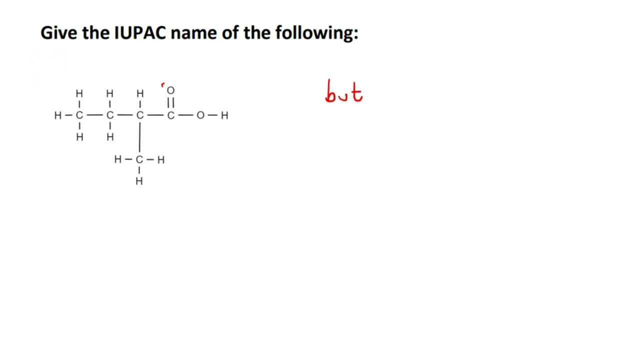 if we start, we're going to start. this is the functional group. Okay, so you're going to start naming from the side that is closest to the functional group. So this is number one, number two, number three and number four. So on carbon, number two: you see there's a branch over here. 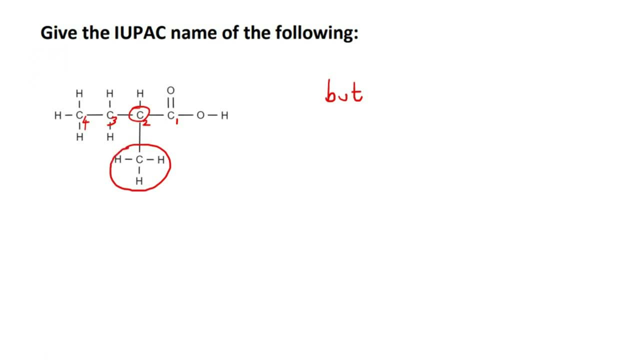 How many carbons are in that branch? One, So that's meth. So you say that on carbon. two, there is a methyl branch. Okay, we need to make this one word. Okay, now we need to think about. what type of molecule is this Like? is it an alcohol, alkene, ester? Well, what you should.